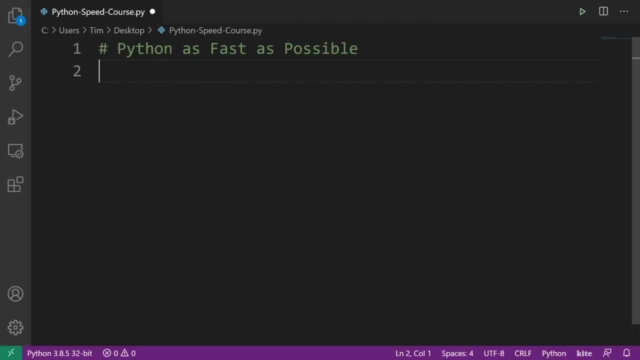 Hello everybody And welcome to Python as fast as possible. In this video, I'm going to be trying to teach you Python as quickly as I possibly can. That means I am going to go over things quite quickly, I'm going to talk very fast and I will note that this is not for absolute beginners. If 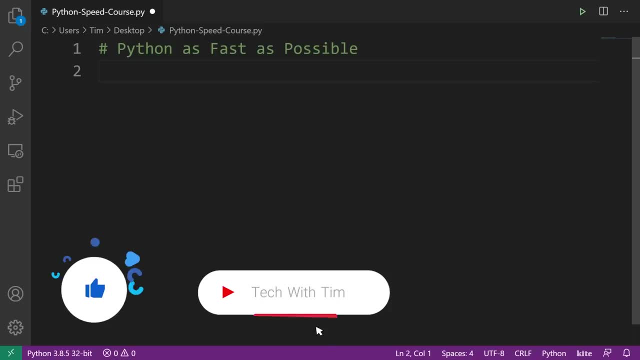 you are looking for a beginner level tutorial series. I have many on my channel. I will link a ton of resources down below, And if you feel that I missed anything or made any mistakes, please do leave a comment. with that being said, let's go ahead and get started and get into. 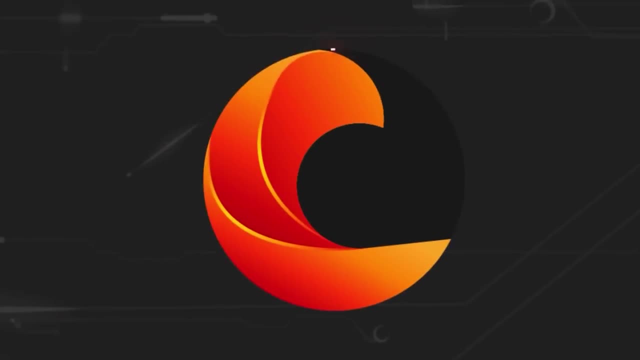 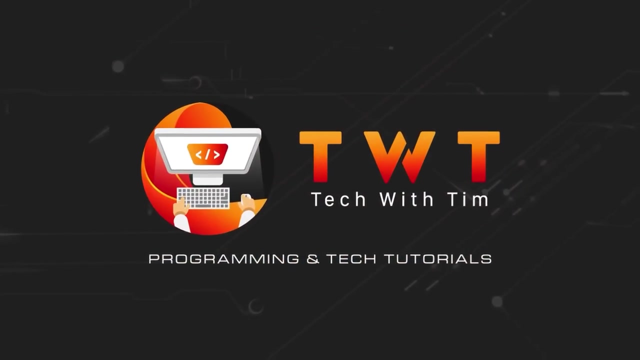 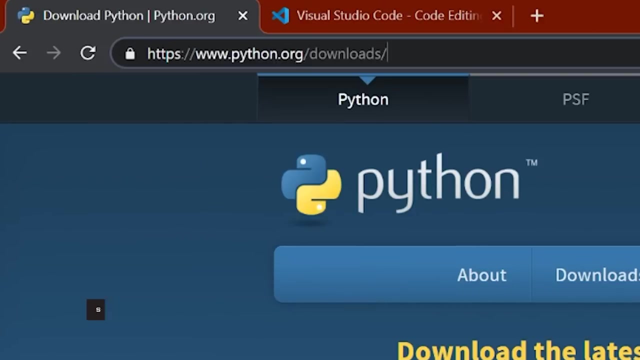 Python as fast as possible. To get started, we need to download and install Python. Please download the most recent version of Python from the Python website, which will be linked in the description. If you're using any version of Python which is below 3.6,, that will not be compatible. 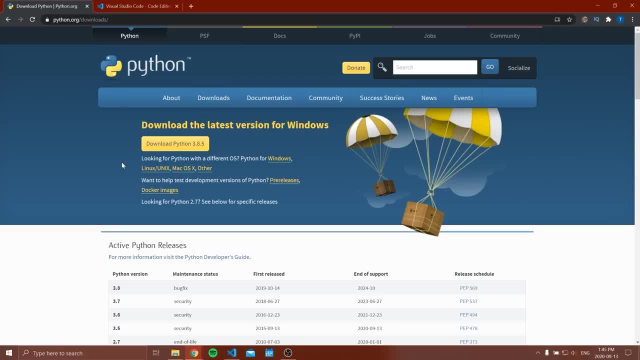 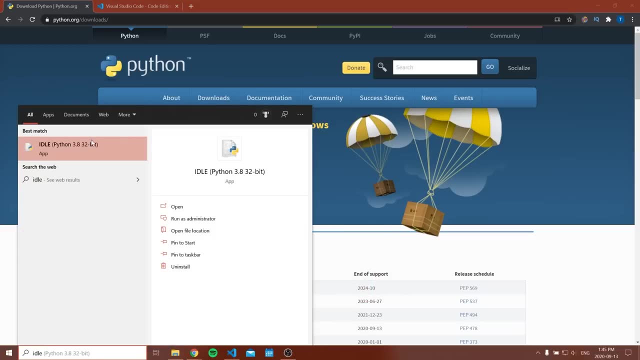 with this tutorial. When downloading, please check the box that says add Python to path. This will make your life Easier in the future. Now Python automatically comes with its own environment to write code in. This is ideally. you can use this to write your code if you'd like, but I prefer to use visual. 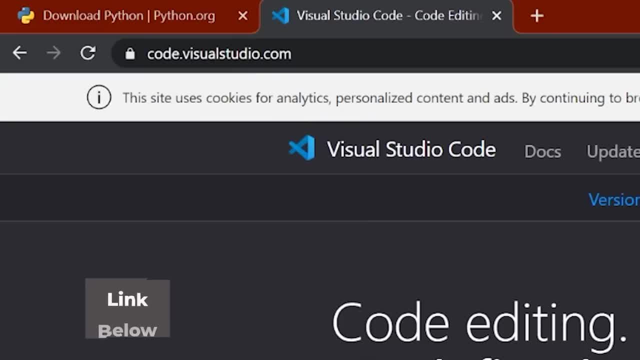 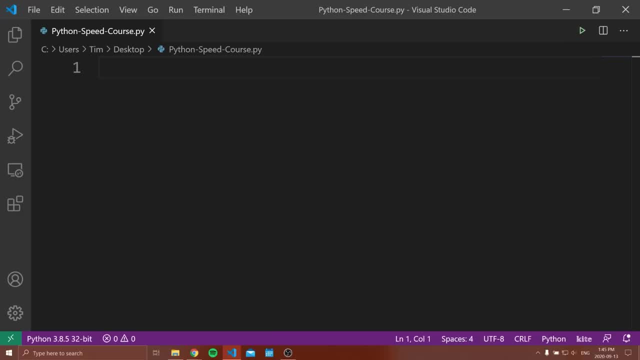 studio code, which is a text editor to download, that You can go to the link in the description and just download the stable build for whatever operating system you're on. Now, if you're using VS code, there is one little bit of setup we need to do to get started here. We simply need to. 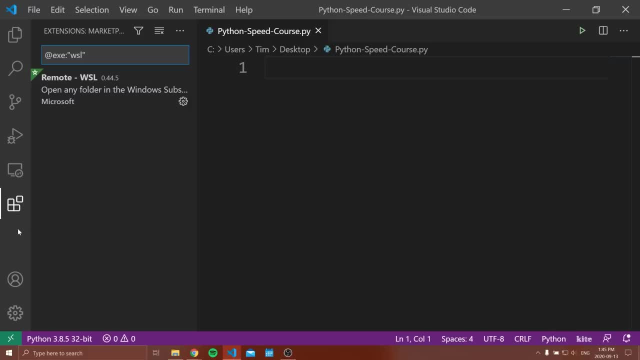 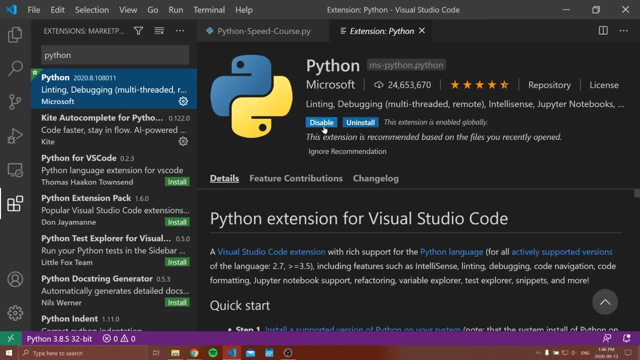 install the Python extension. go to the extension tab here. This will bring us to the VS code marketplace. We can type Python and then we can see the Python Extension and simply press install. You can see for myself. I already have it installed. 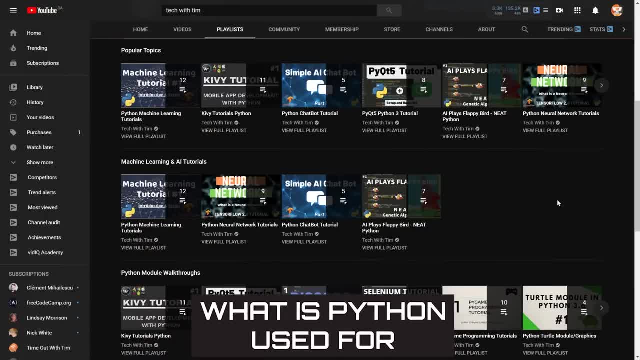 So, before we get started, I thought it would be a good idea to talk to you about some of the things that Python is used for. here I am on my channel, in the playlist tab, and you can see a bunch of different playlists just giving you an idea of some of the things that I've created with. 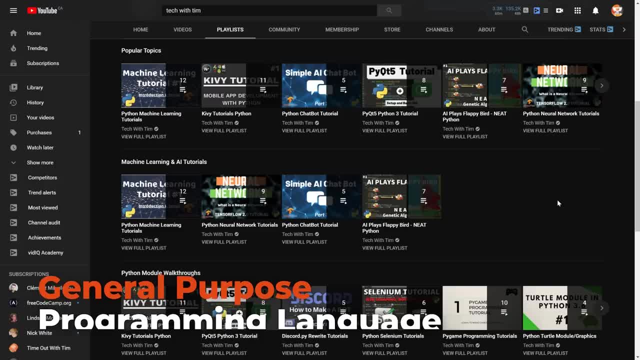 Python and taught on this channel. Python is a general purpose programming language. It is very easy to learn, versatile and really easy to write it. The core advantage of Python is typically how simple it is, How easy it is to write it. The core advantage of Python is typically how simple it is, how easy. 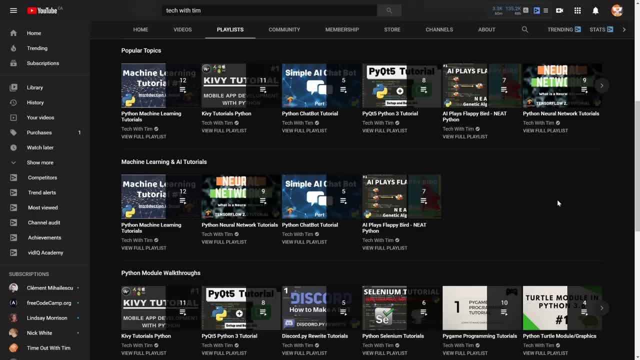 the syntax is to read and just how fast development is with it. That being said, Python is mostly used on the web and in machine learning, artificial intelligence and data science related tasks. Now, the sponsor of our video knows a ton about that, And that is simply learning. I need to. 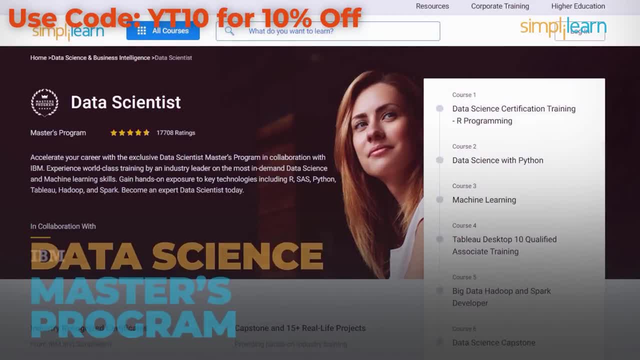 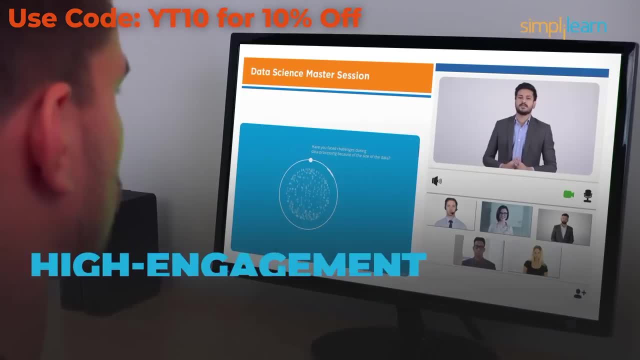 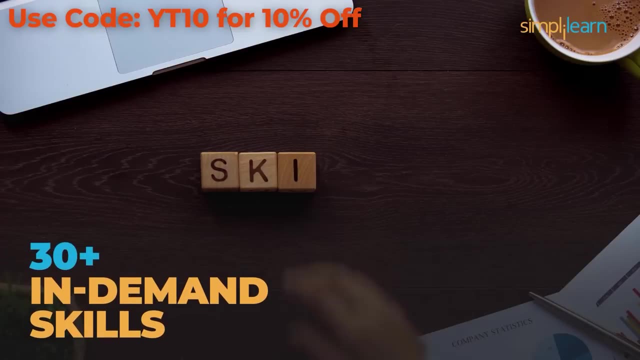 thank simply learn for sponsoring this video and giving you all a discount on their data scientist master program that was co-developed with IBM. This program is comprised of six unique courses that implement a unique blended learning experience and a high engagement online classroom environment. During this program, you will master 30 plus in-demand skills and work with 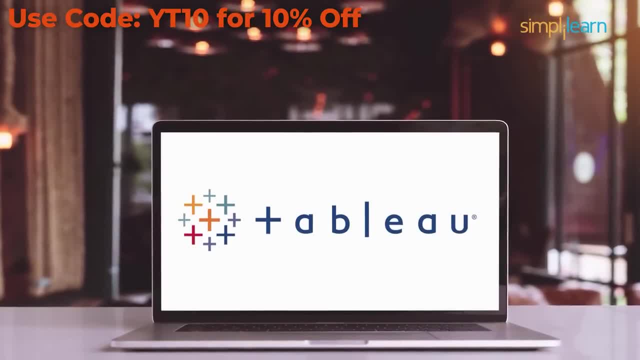 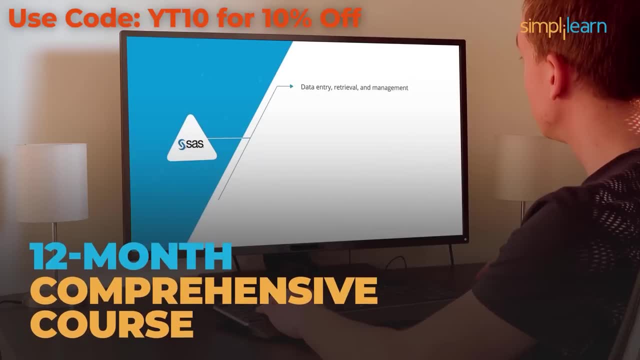 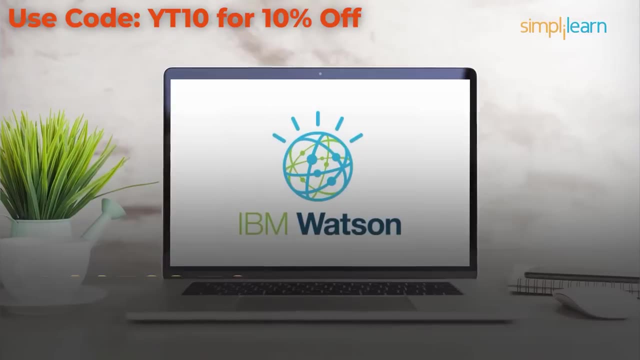 tools and languages like R, SAS, Python, Tableau, Hadoop and Spark. You'll master these skills through 15 real life projects and one capstone project during this 12 month comprehensive course. You'll also be given 1200 USD worth of IBM cloud credits to use during your 24 seven access to the 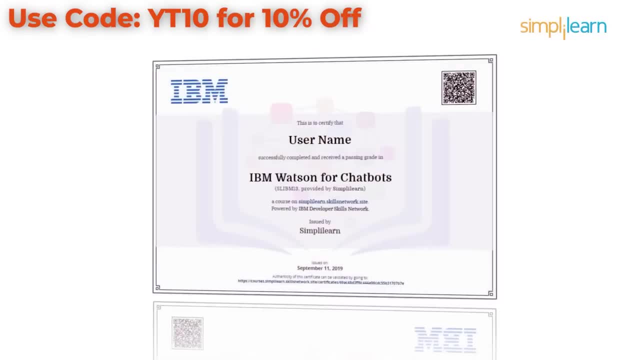 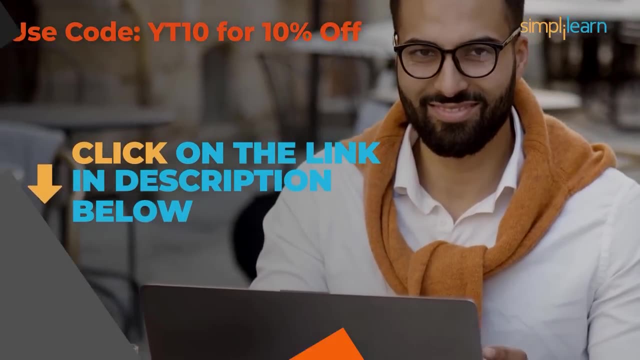 IBM Watson platform. After completion of this course, you'll be given certificates from IBM and simply learn to testify to your skills As an expert in data science. get started by hitting the link in the description. I want to start by covering the core data types in Python. These are in float, string and wool. 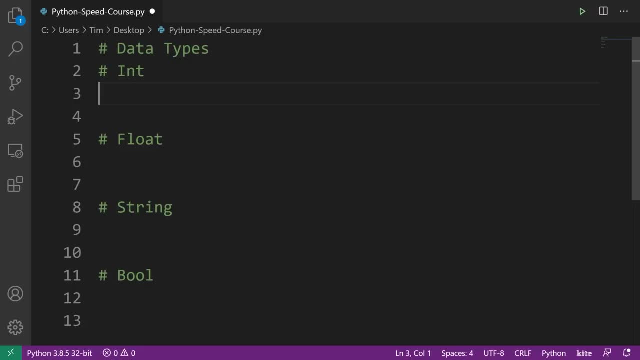 int, otherwise known as integer. Now, an integer or int is simply any whole number that does not have a decimal point on it. So 2,, 3, 7, 3, 7, that was going to be an int. negative nine, That's an. 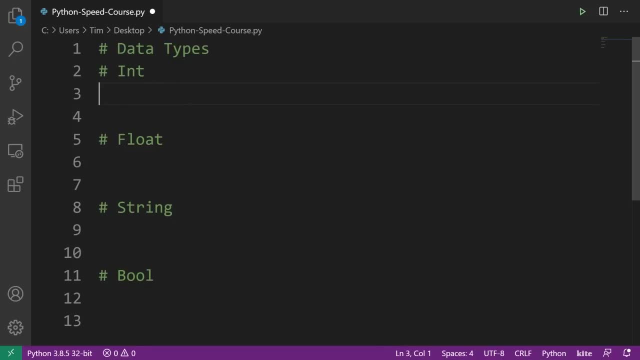 ant: negative. Some random large number is an int. so long as it does not have a decimal point on it, We consider it an int. Float is almost the opposite of that. It is simply any number that has a decimal point on it. So something like 2,, 7,, 2.0,. this is a float, Even though you can consider this a whole number. 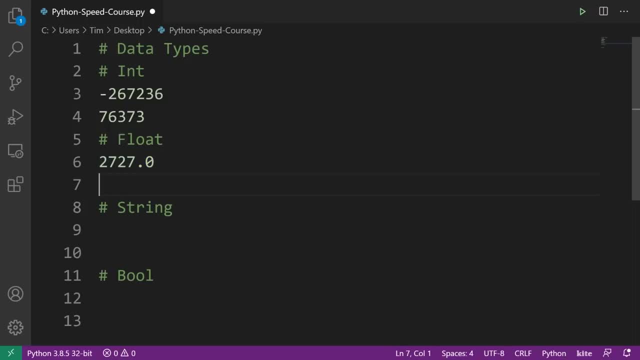 the 0.0 adds a level of precision to this which makes it a float. Of course, something like 9.7 would be a float. Whenever you see a decimal point, that means the number is a float. Next we have 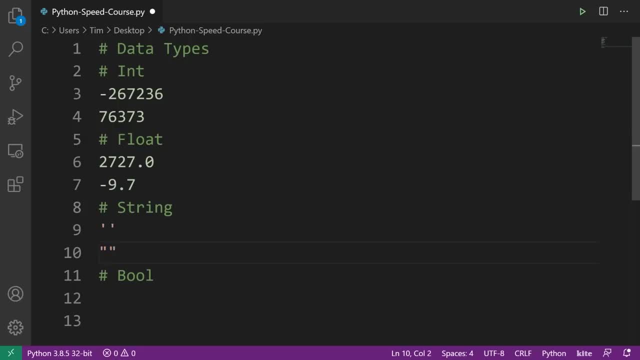 string. A string is simply anything surrounded by single or double quotation marks. Typically, we consider this a sequence of characters or numbers, So if I type something like hello and I type something like hello, these two strings are actually completely equivalent. It does not matter whether you use single or double quotation marks. 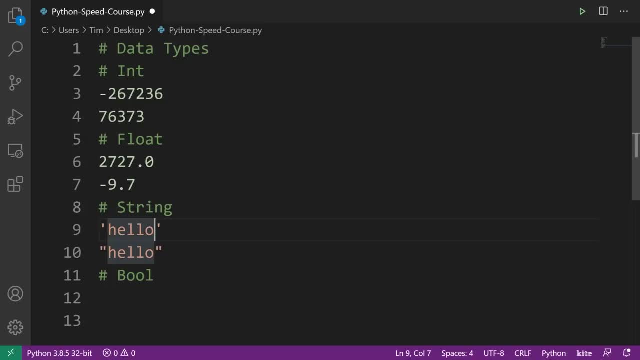 There is no difference. I will note that if you want to embed a double quotation mark or a single quotation mark in the actual string itself, then you would usually wrap the string with the opposite type of quotation marks. So in this case I want to have this double quotation mark inside the 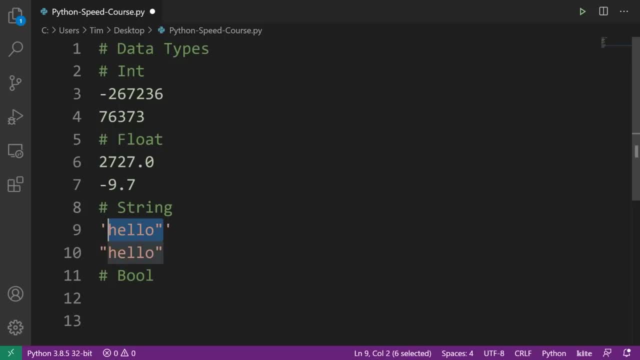 string. So I wrap the string with single quotation marks. Now, just to note here if I do something. six: even though you might consider this a float, this is a string, again, because it is surrounded by single or double quotation marks. Remember the definition: anything defined or surrounded. 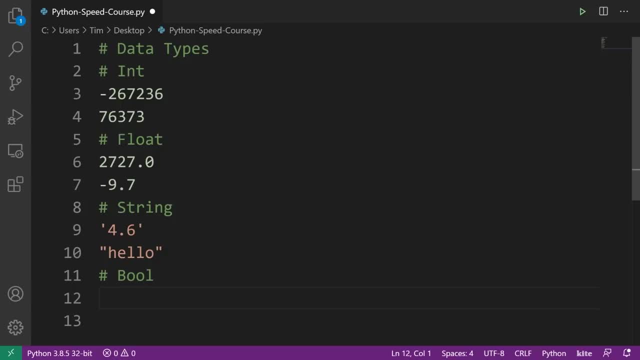 sorry, by single or double quotation marks. Next, we have Boolean. This is one of two values. we have true or we have false. Some people may consider this one and consider this zero. We're going to look at these later on and you'll see why that's important. but that is a Boolean value And these 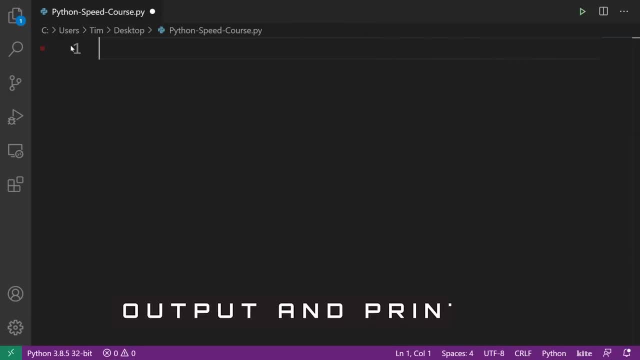 are the four core data types in Python. The next topic I'd like to cover is output in printing. This is very important And we will be doing this a lot in this video. in Python, There's a simple function called print. This is how you output something to the console. 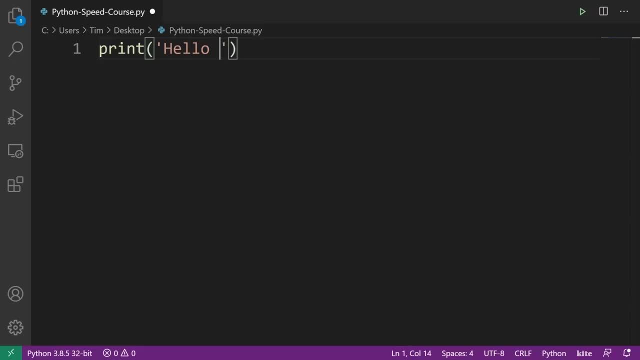 When you run your program, typically when you print something you'll put it in strings. So I want to print, say hello world, So I will print the string hello world like that. And if I run my program by pressing this run button you can see down here in the console we get hello world. 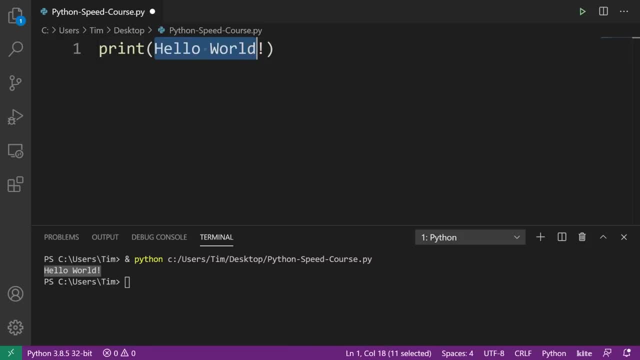 Now notice that if I just type hello world like this and I don't put it inside of a string and I run my program, I will get an error. This is because I cannot simply print something like this. The program does not know how to. 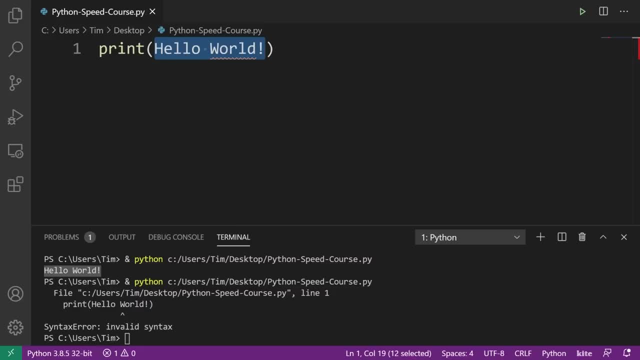 interpret hello world. If it is not wrapped in strings, that is because this is not one of the core data types and we have no variable or anything that denotes what hello world is. That being said, if I want to print a number, say like 4.5, Python knows what 4.5 is because it is. 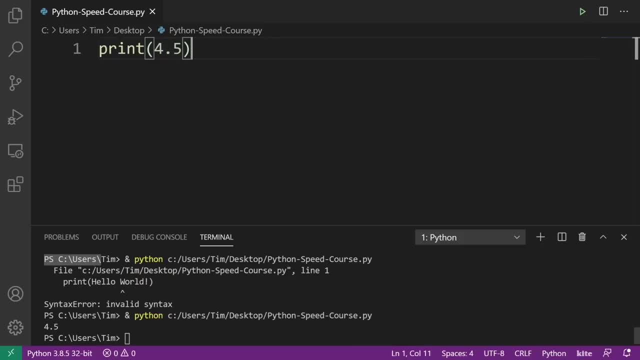 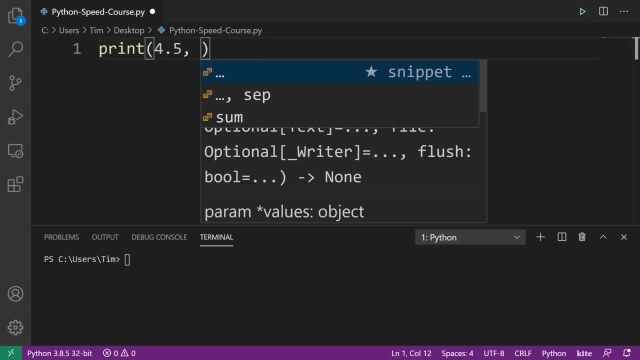 a float. You can see when I highlight it it says float. If I run this, it will print 4.5 out and there will be no problems. Now, if you want to print multiple things, what you can do is separate them by commas. So say, I'd like to print 4.5, and then I would like to print hello. 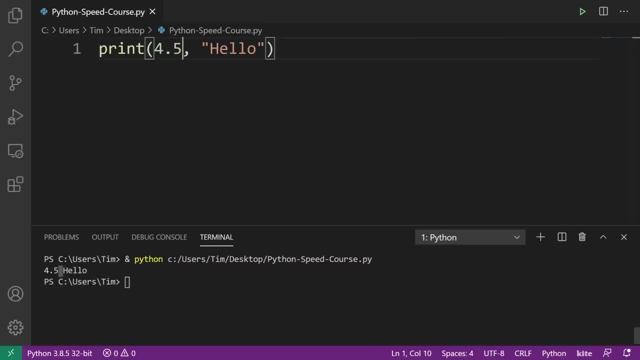 When I do this, it will automatically add a space between the two things. Let's just put another string here just to show you what I mean. So 4.5, hello notice, it adds that space in between. Now we will talk about how you can print things without the space in between later on. 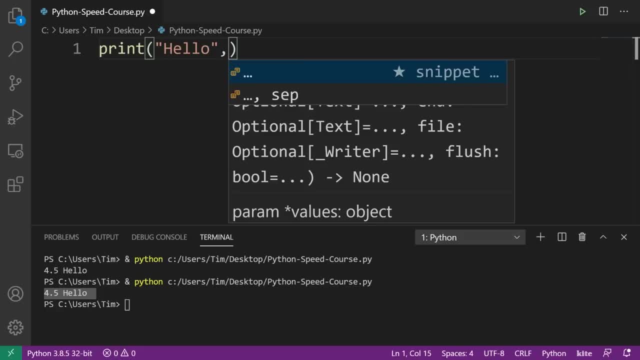 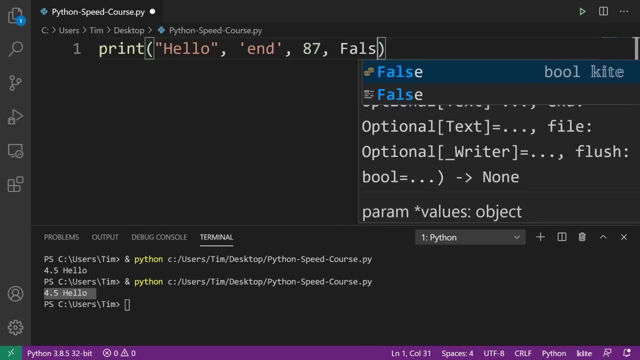 but that is the basics of a print. If I want to print many things on the same line, I can go hello, I could say and I can say 87, I can say false, and I can run this and this will all work. Hello And 87, false. Now there's a few arguments. 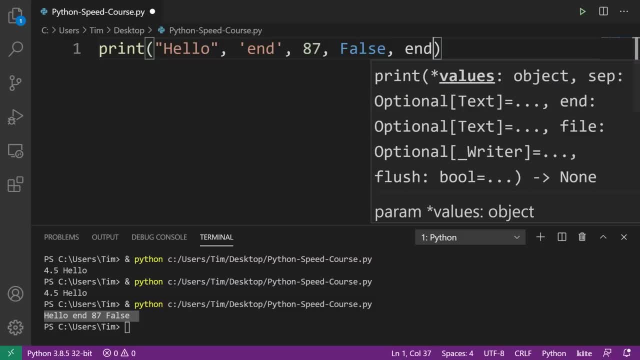 that you can pass into the print function. If you do a comma and then type end equals, you can denote what you want the end of this print statement to be by default. The end here is a carriage return, which is backslash, And what that means is go to the next line after this line is: 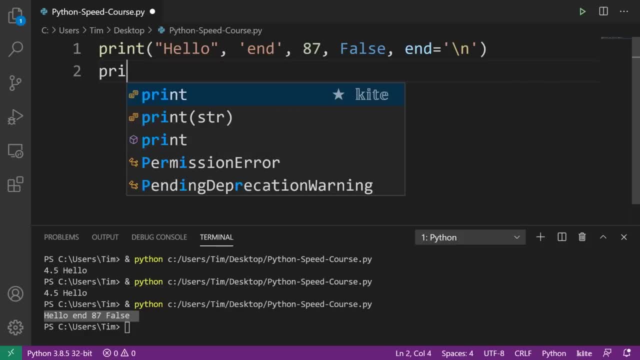 printed. Now notice if I don't add this backslash enter, in fact. let me just show you what happens by default. So let's say I have hello and 87. I'm going to get rid of this and I print both these things out. We get these on two separate lines. That is the 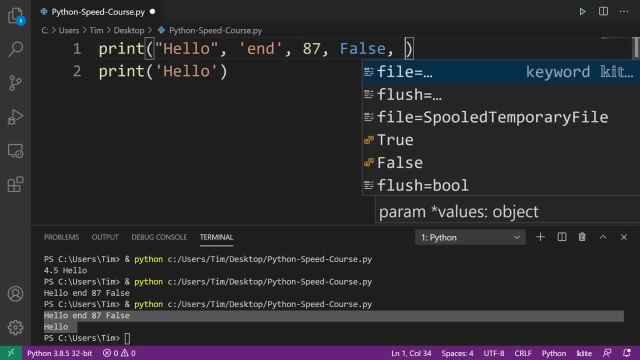 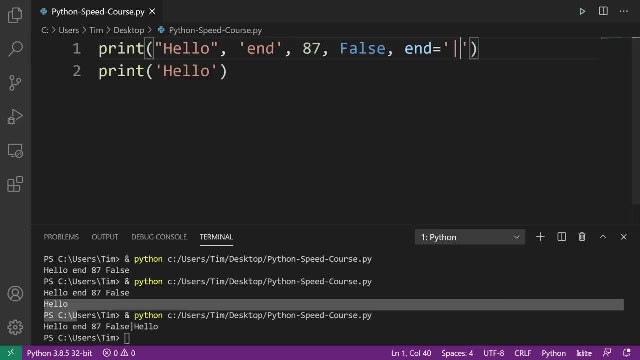 default behavior of the print statement and prints on a new line. Now notice: if I add end E, end equals and instead of a backslash N let's say uh, this pipe like that. And I run this now at the end of the print statement. it simply prints a pipe. It does not add the carriage return. 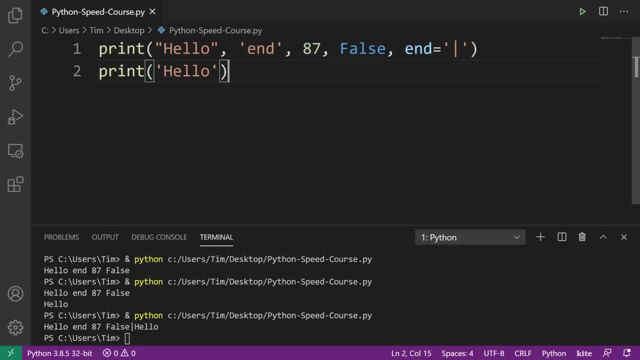 which means we do not move on to the next line. That's a little bit more advanced, but essentially the carriage return is that backslash N, And again that means just move down to the next line. That is the basics of printing and output. And now let's move on. next, Let's move on to variables. 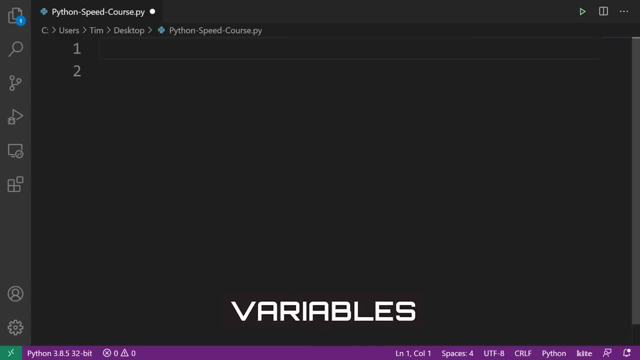 Variables are an important part of any program in Python. They are quite easy to create. When you create a variable in Python, you simply type a variable name, a space and equal sign and then assign it to some value. This value is going to be some data type, some function, something else that. 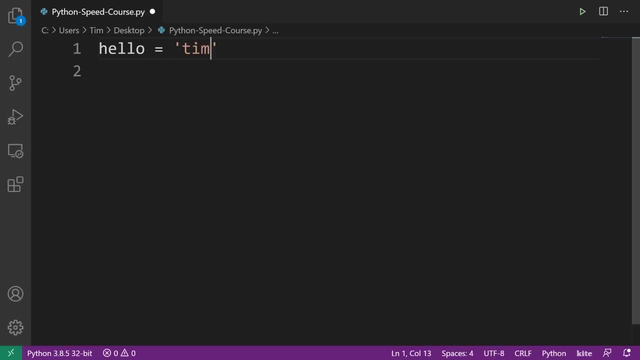 we'll talk about later on. To give you a basic example, I'm going to set the variable Hello equal to the value Tim. Think of a variable like a bucket that stores some data or stores some type. Now, if I want to access, 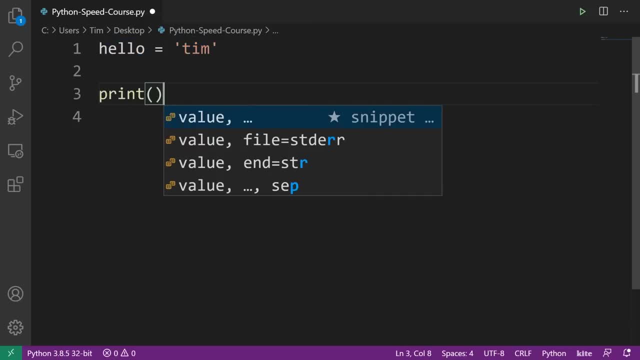 the value that is stored in hello. what I can do is I can simply say print Hello. What this will do is it will say: okay, this is a variable. I know it's a variable because I saw it earlier on the program. Let me see what its value is And I will print that value. So now I'm going to run and you 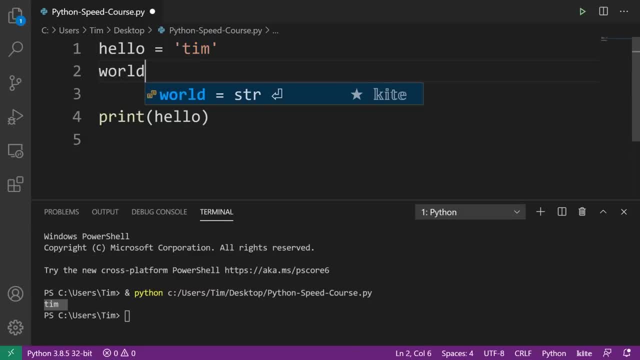 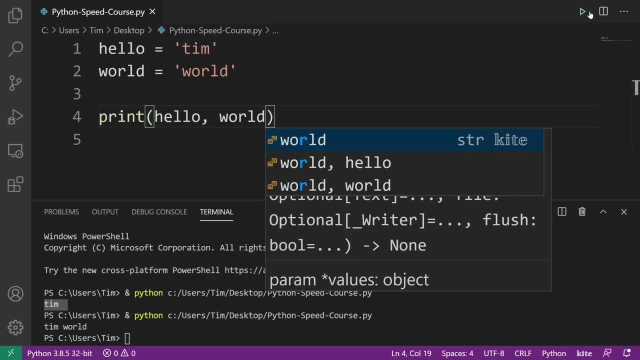 can see that. we get Tim. Let's make another variable. Let's call this world. Let's actually set this equal to the value world. Now let's print hello comma world And let's see what we get. We get Tim, and then space world. 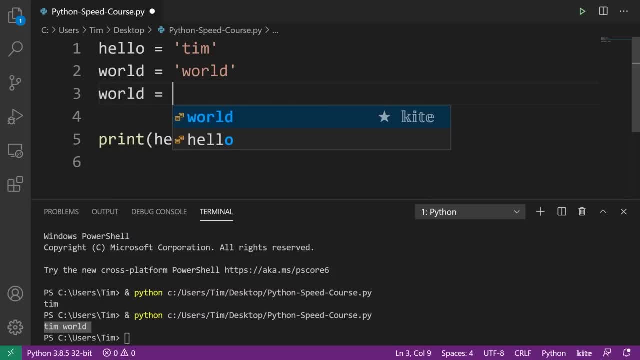 Variables are somewhat complex. You can make them equal to other variables. If I decide to change the value of world to actually be equal to the variable hello, what's going to happen is they're going to say, okay, hello is a variable. What is a low equal to hello is equal to Tim. So I will. 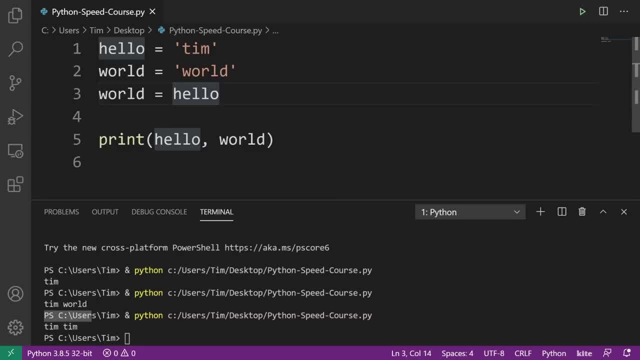 print Tim Now, watch what we're going to get. We get Tim Tim. Now what happens if I come here and I change hello to be equal to no? If I do this, what's going to happen is: world will not change, because world was set equal to the value. 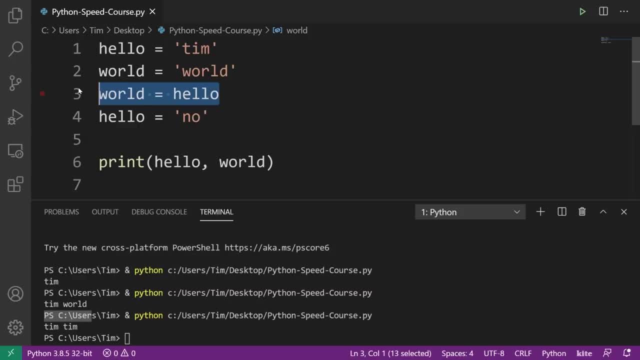 of hello at this line, at this point in time, line three- because our program reads from top to bottom: the value of hello was Tim, So world gets set to Tim, Then hello gets set to no. that does not change the value of world. So what you're going to see is we're going to have Tim and then 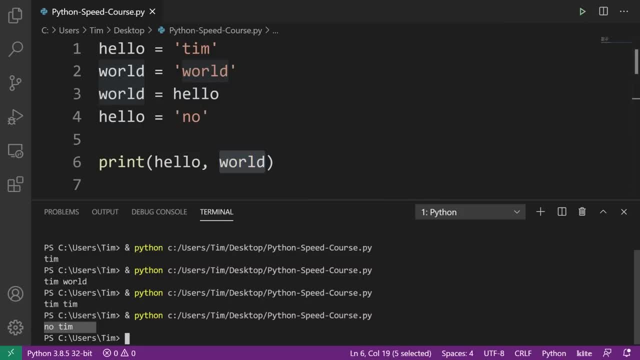 we're going to have no. So let's have a look here and sorry, other way around We get no, Tim. my bad that we printed a hello first And then World. I had that mixed up. That is the basics of variables. There's many other things that we can. 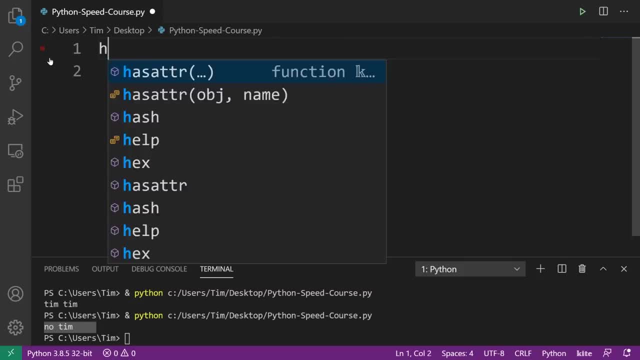 do with them, but let me just tell you about the naming conventions for them. So in a variable you are not allowed to have any special characters and you cannot start with a number, So you are allowed to have an underscore. That is the only exception in terms of special characters. 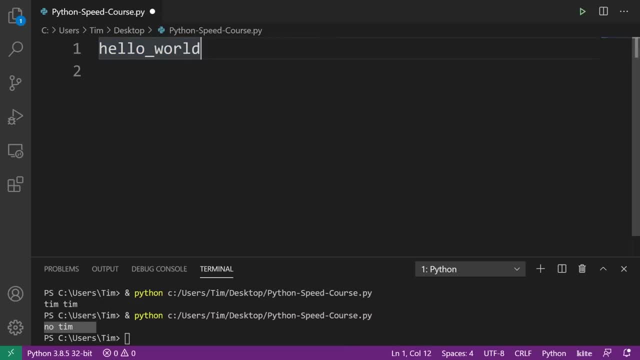 Usually you will use that when you're denoting a space, and in Python the convention is typically to separate things using an underscore, and other languages You may see something like hello world. If you want it to make a variable that has multiple words. 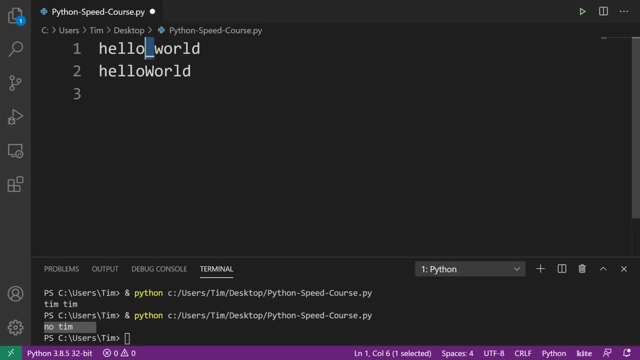 in it, but in Python stick with snake case, which is what this is known as. the other one is camel case, and use underscores to separate your variables. Just to give you an example of what I mean: you can not start a variable with a number So nine. 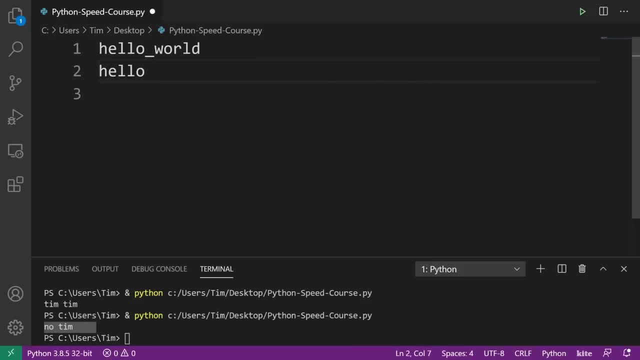 hello- notice, I'm getting the red line popping up here and I could not do something like hello nine. That does not work. But if I want to, hello world 32, that is totally fine. That is a valid variable name. The next: 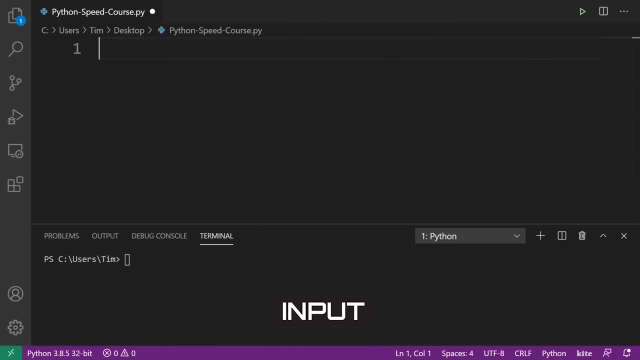 topic I want to talk about is getting user input. Just like printing something is very simple. Getting input is simple as well. What we do is we simply use the input function. We have our open and close parentheses and then we type what's known as. 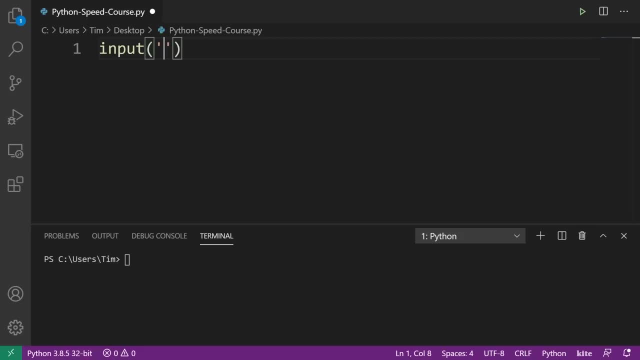 a prompt inside of these brackets like this. Now, this does need to be in a string, Unlike the print statement. we cannot do something like 4.5 in here. That will not work. We do need a string. So what I'm. 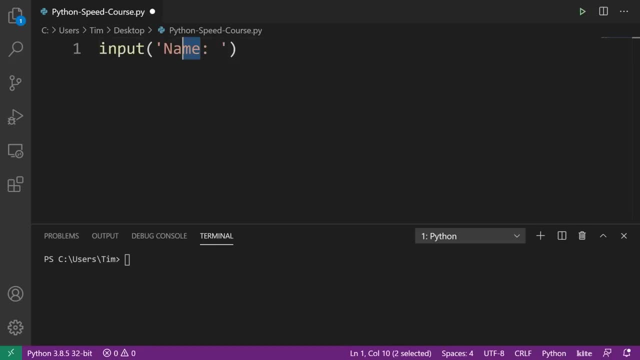 going to do is I'm going to add a prompt, Say I want the user to type their name, Then I will say name, I'll do a colon And then I will add a space between the colon and the end of the string. 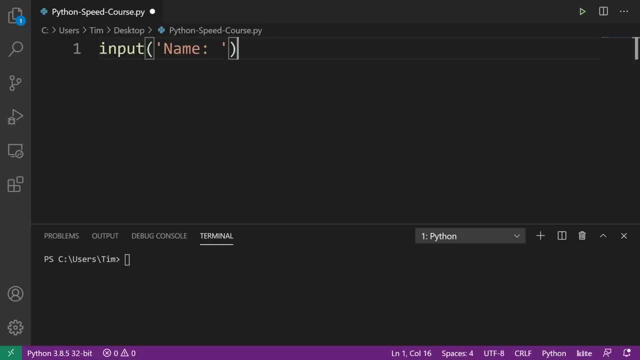 The reason for this is that the user will be able to start typing at on this line right after the prompt. So if I don't have a space, then what's going to happen is the user will start typing right where the colon is: which of 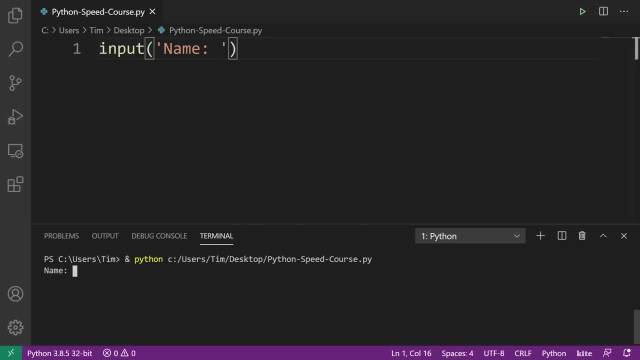 course is not going to be good. So let's go ahead and run this and have a look at what happens. We can say name colon space and now I'm going to type Tim, That's great, But how do we actually get? 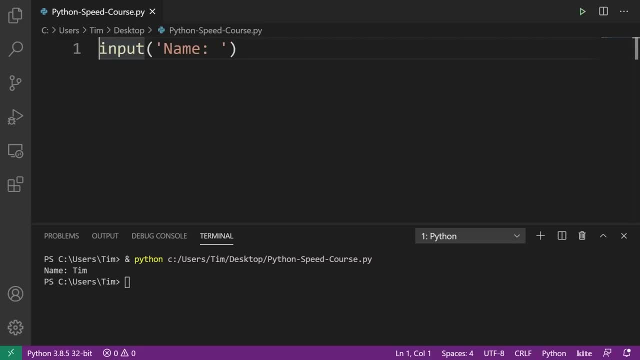 the value. How do we store what the user typed in so we can use it later? Well, we need to assign this input to a variable. So what I'm going to do is I'm going to say name is equal to input. I just 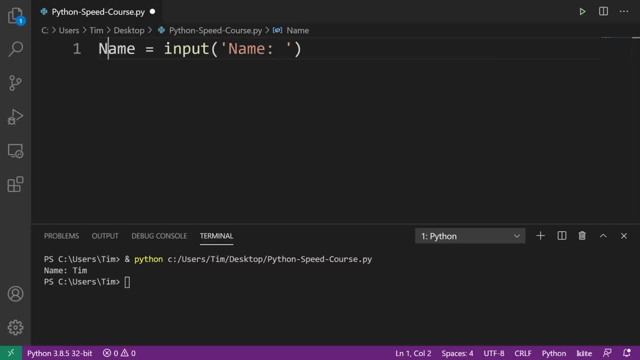 want to note, because I forgot to say this previously: we could have capitals in our variable name If we want. that would be fine, but I'm not going to do that. And now what will happen is, whatever we type in will be returned to us. 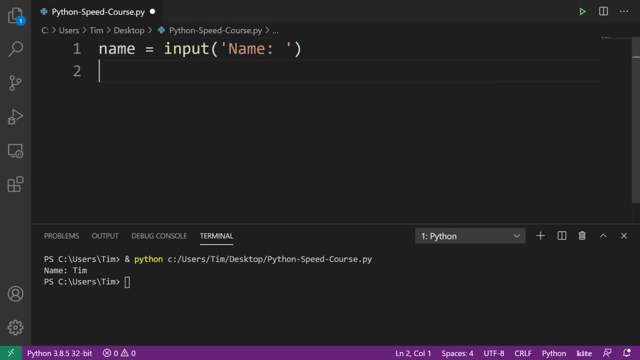 in the statement as a string and it will be assigned to this variable name. So if I go ahead and print the value of name, what's going to happen is whatever we type in here will be printed out. So let's have a look at this name. 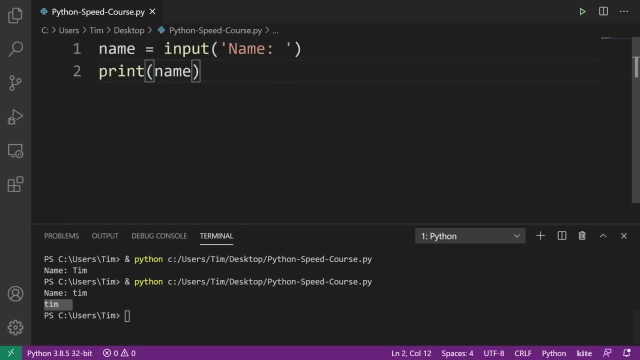 Let's type Tim And we see that Tim is printed out below there. Now we of course can get multiple user input, So I can say something like: age equals input, age colon. And now let's see what happens when I run this. So we: 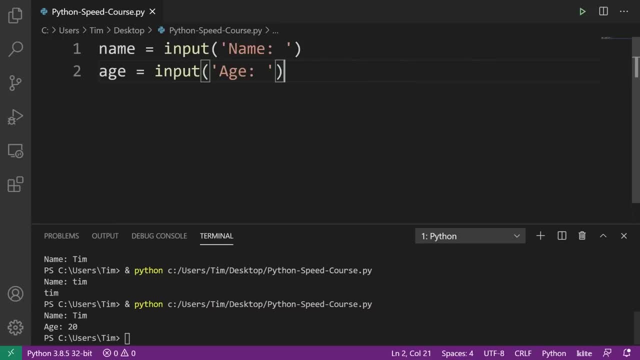 go name Tim, age 20, and we could put print those out if we want, but I'm not going to. actually, you know what. let me show you one example where I print them out. Let's say hello And then let's go comma name. 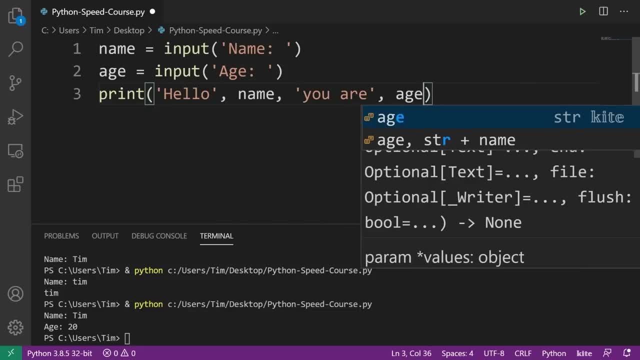 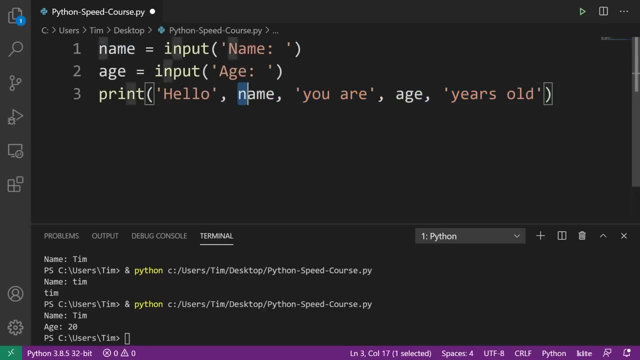 And then you are- comma: age: years old. So this is a way that we can combine variables and strings so that we print out a meaningful response that says: hello, whatever the name is, you are, whatever the age is- years old. So in this case I'll say: 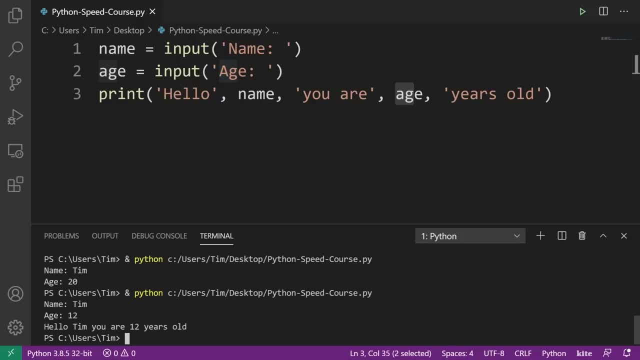 name Tim, age: let's go 12 and it says: hello, Tim, you are 12 years old. All right, So that is it for input. Now we're going to move on and talk about how we can actually convert, say numeric input into. 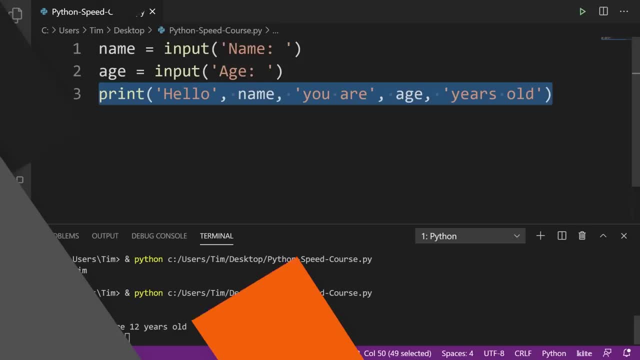 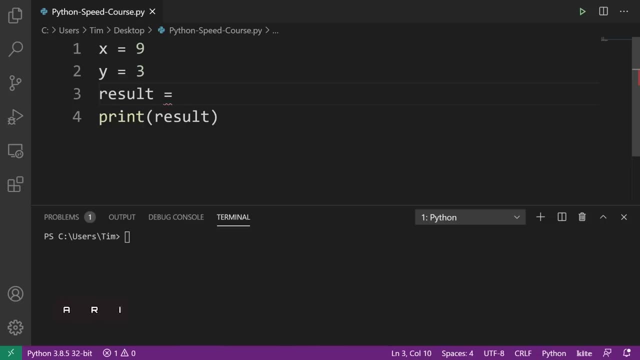 a integer or float, because a default comes back as a string. All right, So the next topic I want to cover is arithmetic operators. These, essentially, are like plus minus multiplication exponent- how you perform mathematical operations in Python. Now just something to keep in mind when we're 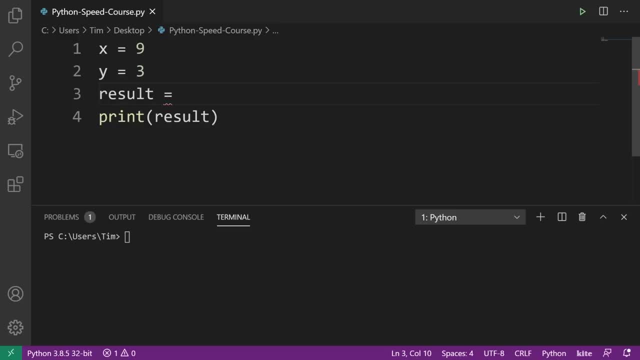 performing and using arithmetic operators, we have to make sure that the data types on the left and right-hand side of these operators are operators otherwise known as the operands, are the same data type or are both numbers. What I mean by this is if I have something. 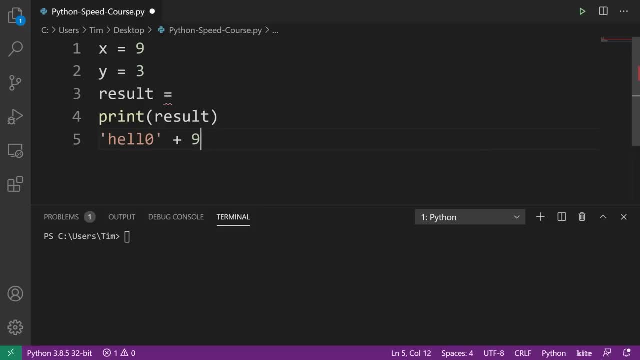 like hello, and I try to add nine to it. well, that just does not make any sense And we are going to get a PR error and something's going to be wrong with our program. So just keep that in mind. I cannot. 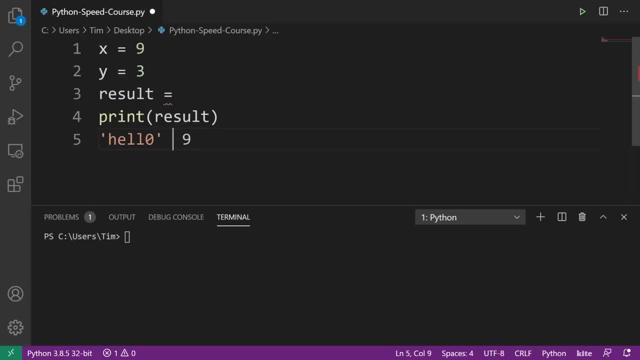 do hello minus nine. You cannot do hello divided by nine. You actually can use the multiplication. You can take a guess at what that's going to do, but I will show you that later. All right, So let's go through the. 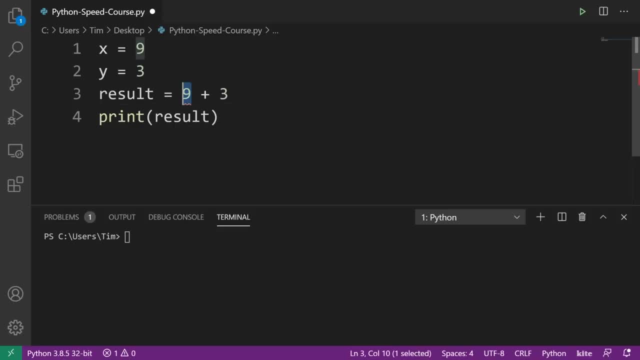 basic operators. The first one is the plus sign. Very straightforward: We can add nine plus three, or in this case I could add X plus Y. So X is nine, Y is three. We can add those two values together, Ignore the 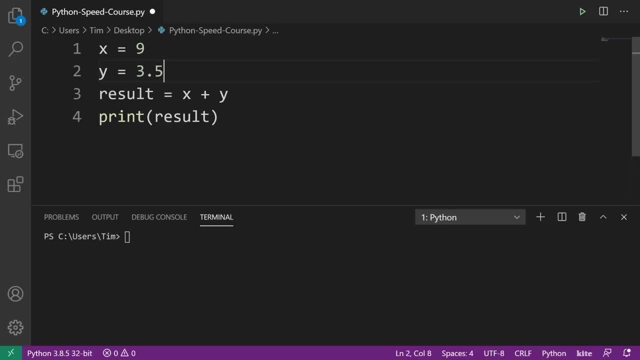 squiggly When I save, that goes away Now. so I'm going to keep in mind if I make this 3.5, this works totally fine, even though these are different data types. since they're both numbers, I can add. 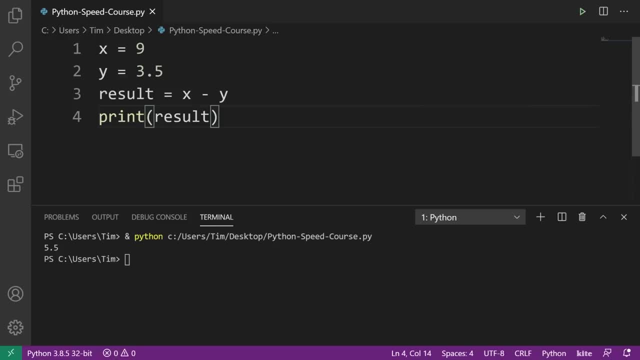 them together, Of course. I can do the subtraction- Let's run that- I can do the multiplication, which is an asterisk, and I can do the division. When we do the division, we get some crazy number. Just keep in mind that. 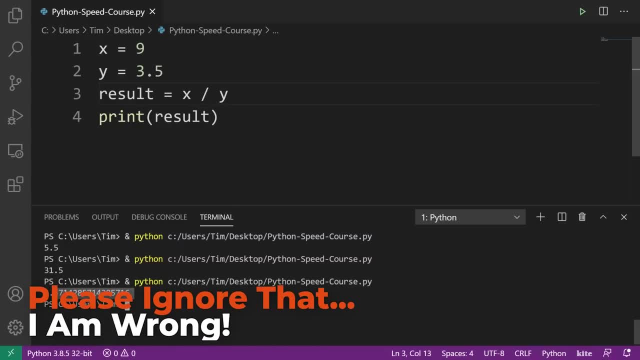 the maximum per decision in Python, I believe, is 13 decimal points. There is ways to get beyond that, but that is kind of too advanced. I'm not going to cover that right here. And when you ever do division or you're dealing with. 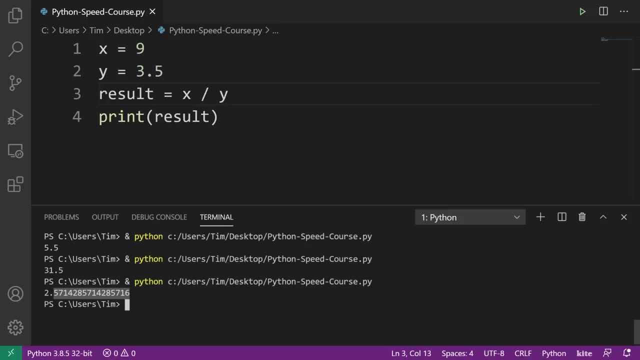 rounding and all of that. um, that's always a problem in computers, So just keep that in mind. You're not going to get the most precise answers with division like this. Uh, if this is a non terminating decimal point anyways, hopefully that makes. 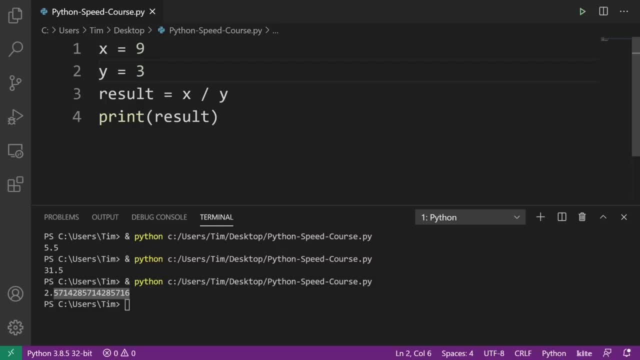 sense. Now I just want to point something out. If I actually have, say, nine over three, of course you know that that answer is three And that is a whole number. right, Three is a whole number. but this is actually returning to us a. 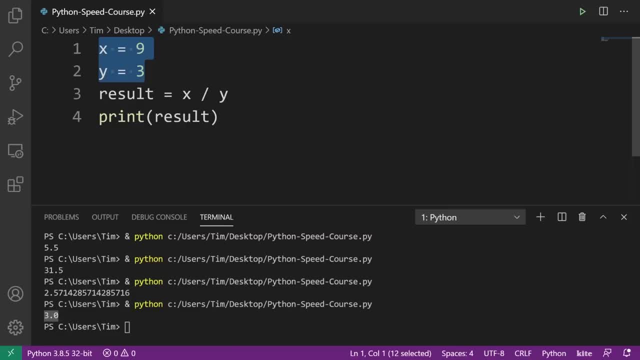 float, not an end, even though neither of these data types are afloat. The reason for that is because, whenever we use the division operator, it returns a float because it does not know if it's going to need to represent a floating point or it's. 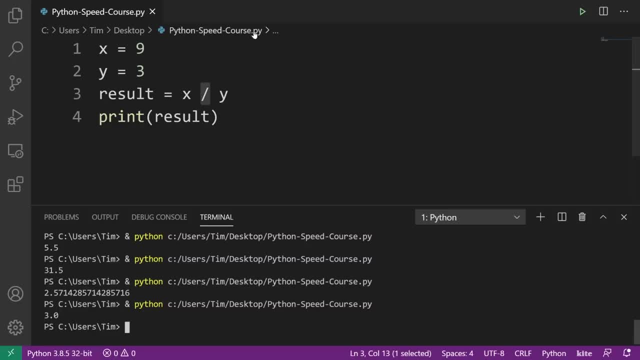 going to have to represent some level of precision, So just keep that in mind. If, for some reason, you don't want this to be a float, of course you can convert the result to an end by just doing int like that. Okay, So? 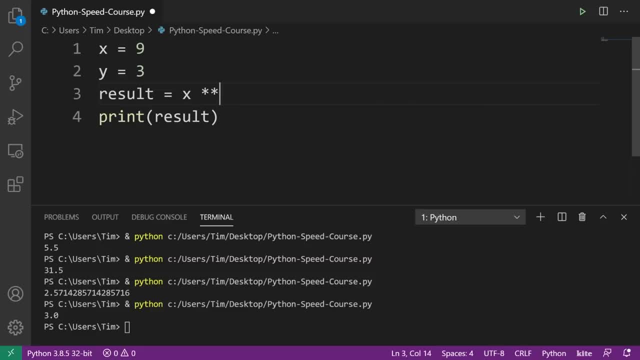 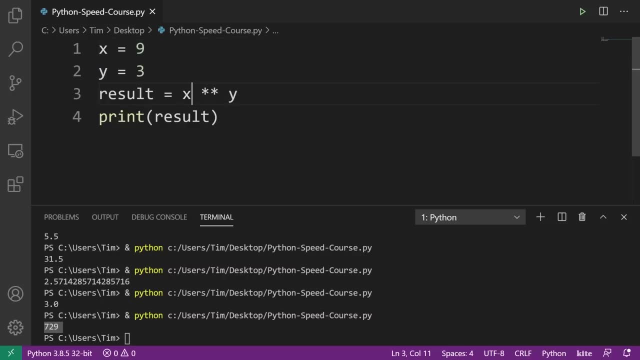 those are some of the basic arithmetic operators. Next we have exponents, So that's two asterisks Like that. this will raise X to the power Y, So we can see where that gives us 729.. And then next we have floor. 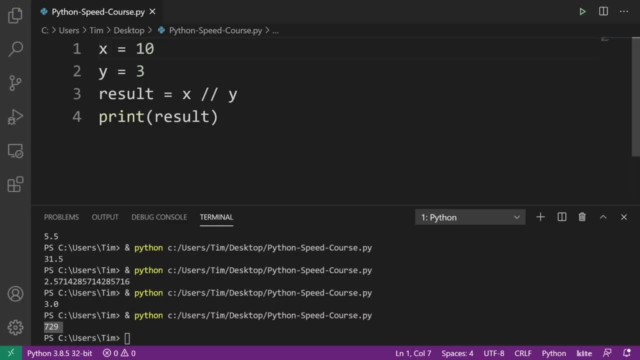 division. So what I'm going to do here is actually make this a 10, have a guess at what you think this is going to give. but this gives us three. The reason it gives us three is because this will give us the integer result of 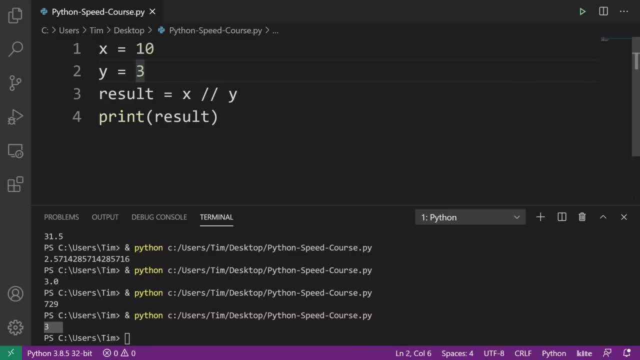 whatever the division is- Imagine this was like 9.333 or whatever it may be- It just simply removes all of the decimal points and just give our. sorry, it'd be 3.333 removes all the decimal points and just gives us. 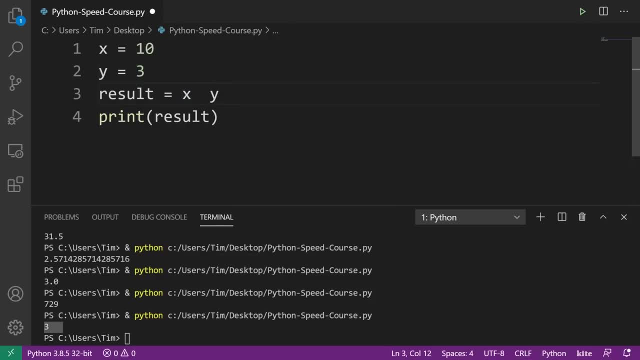 whatever that integer result is. Next is mod. This is the percent sign. This returns to us the remainder after a division, in this case 10,, a mod three is going to be. well, the answer is nine, and then remainder one, right. So 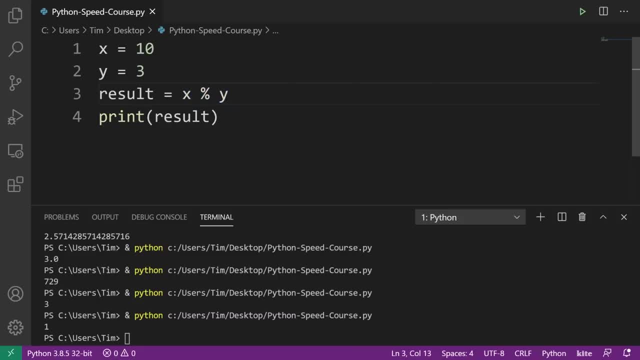 that is why we get one from this here. I think that's it for those operators. Now I will simply show you how we can do, say, order of operations. So if we want to do order of operations, we can use brackets, or if we want, 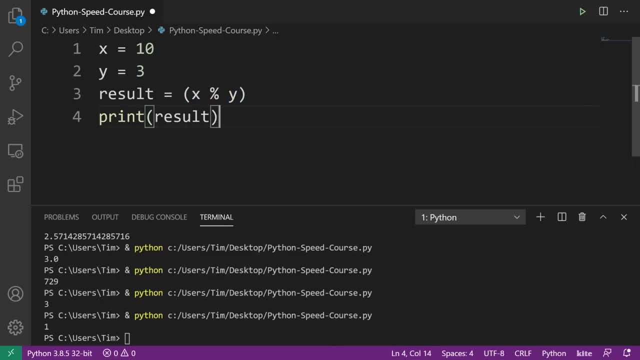 to evaluate things in a specific order. this does follow the simple order of operations, which the acronym I know for it is bed mass, which is B, E, D, And I hate this auto complete. It's making it very hard to do this. 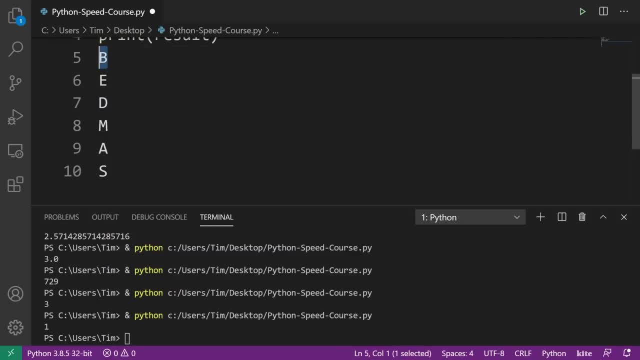 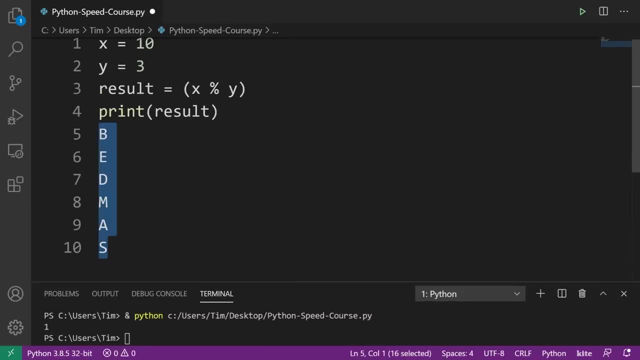 M a S. Okay, So what this stands for is brackets: exponents, division, multiplication, addition, subtraction. Python does follow those standard order of operations If you just write an expression, but of course it's always easier to use brackets. 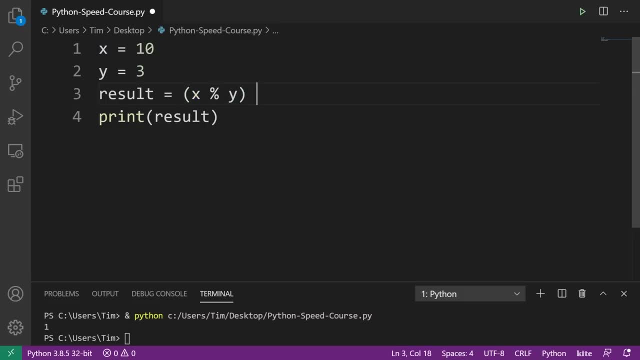 and spread things out. So I can say something like X, uh, mod Y, and then I can multiply that by two. since I didn't say it, The integer division and mod operators are in the lowest order of order of operation. So if you use 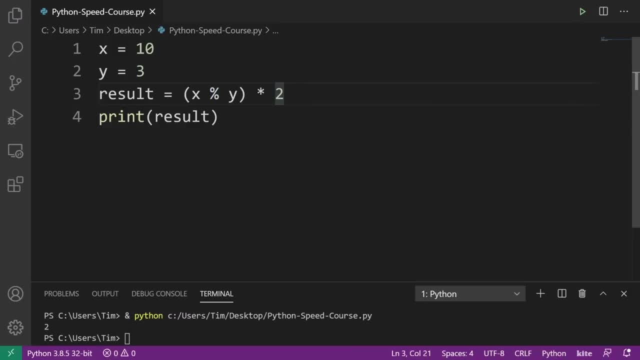 mod. that is going to be below addition and subtraction. Pretty sure that's correct, but someone can correct me from the in the comments if I'm wrong about that. But anyways, you get the point. you can use brackets and that is how you can. 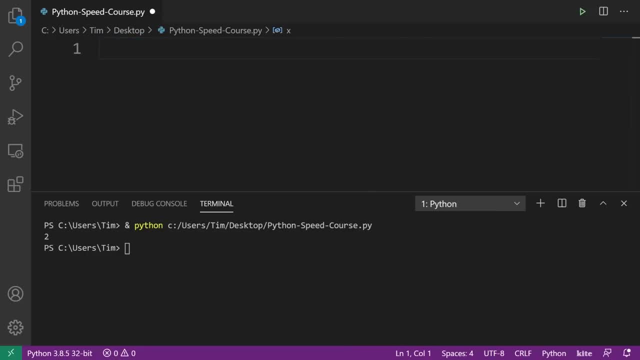 perform and do arithmetic in a certain way, All right. Next thing I need to cover here is simply just an example using input. So what I'm going to say is: num equals input and we'll just say number colon, like that. What I 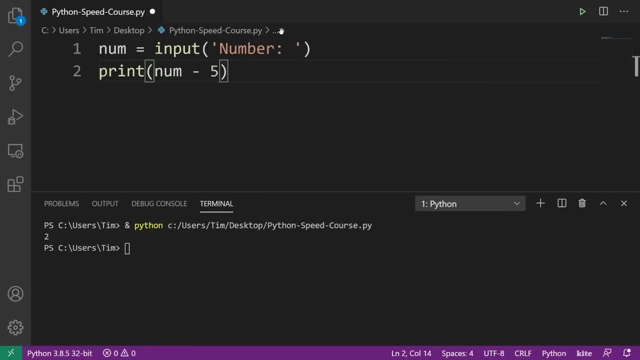 want to do is simply print the result of a numb minus five. So I want to take whatever number they type in and I want to subtract five from it and print that to the screen. So let's try it, And I'm equals five. notice that it says: 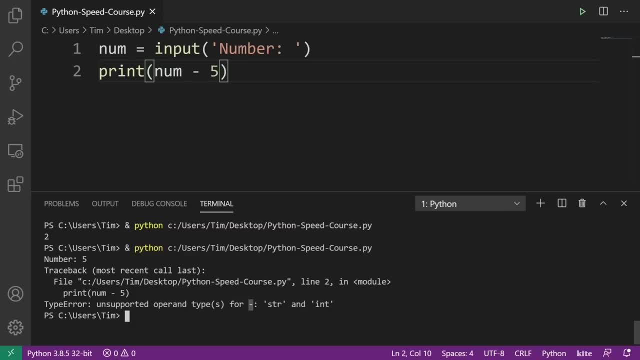 unsupported operand types for minus our four, sorry, Yeah, minus string and it. So what that's saying is that numb is a string, even though it looks like an into us. I'll explain why in a second. and we cannot subtract the number five from it. 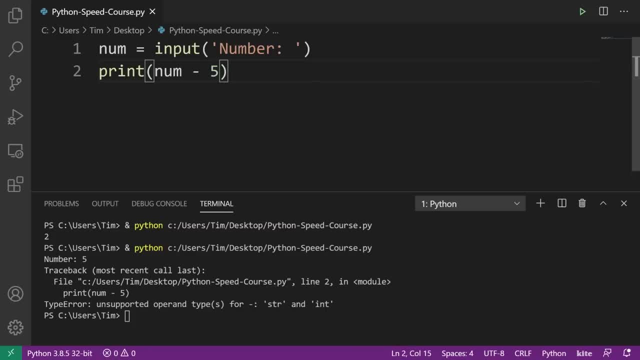 That just doesn't make any sense. The program doesn't know what to do with that. So think about this: Why is numb a string? We typed in five. This should be an int value, from what we understand about our data types. Well, this input. 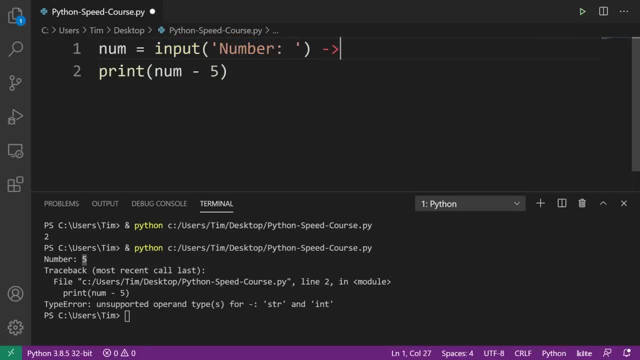 automatically returns to us whatever we type in in a string. So just imagine that whatever we do here, it's going to give us a string And that means that if we want this to actually be a new where numeric value and be able to 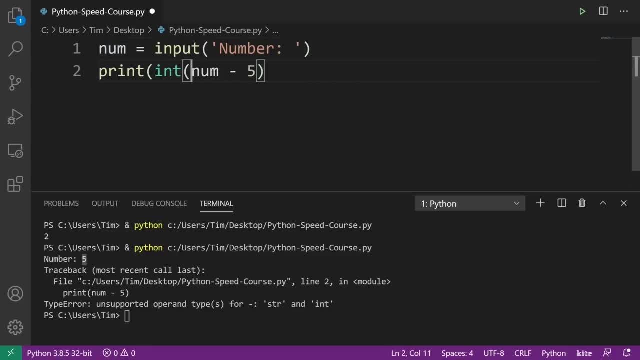 perform arithmetic on it, we need to convert it to an int. So there is this fancy function called int in Python. This will take some string, assuming that there is an int inside of that string, and it will convert it into its integer representation. 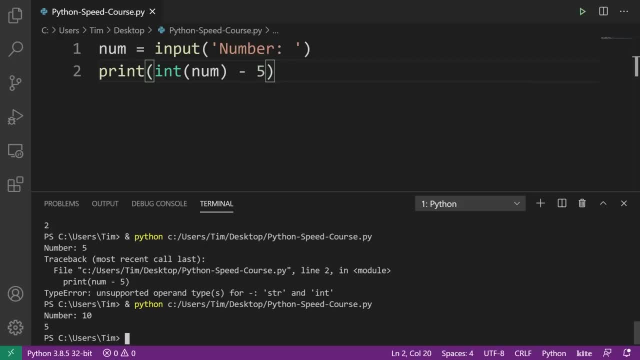 Let's have a look now. when I type a number, let's say 10, of course we get the value five. It took numb, which was 10.. So the string 10, you know, I'll type it out Like here we have. 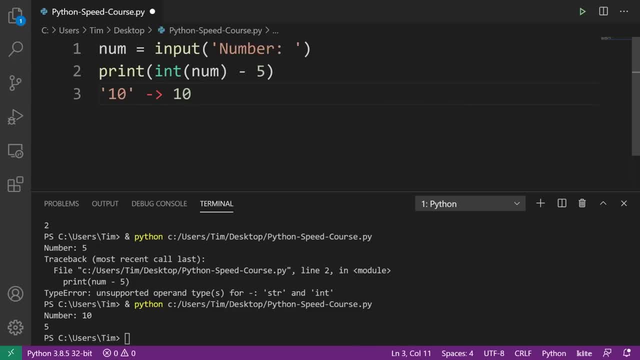 the string 10 and it's simply converted that to the actual integer value 10.. Now you can imagine we have other functions in Python that do this as well. We have, say, float, That's going to take whatever we have here and convert it into. 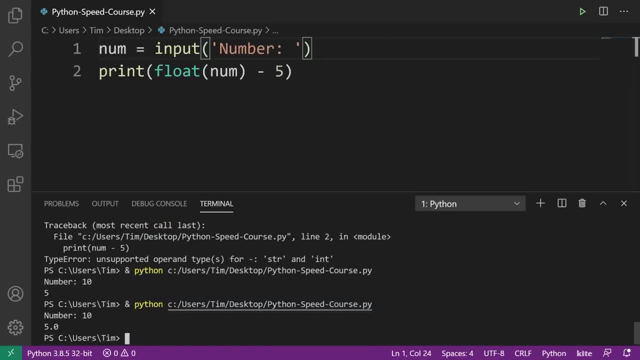 a float. Now notice what happens when I do this. If I do floats 10, we get to 5.0.. Whenever you have at least one float in your arithmetic, it's going to automatically return to you a float It needs to. 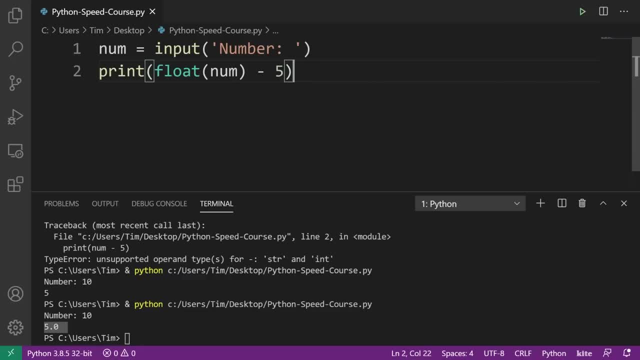 keep the level of precision that uh was in the original you know operation or in the original value. So just that's something to keep in mind whenever you're doing you know plus, minus multiplication if there is one float as 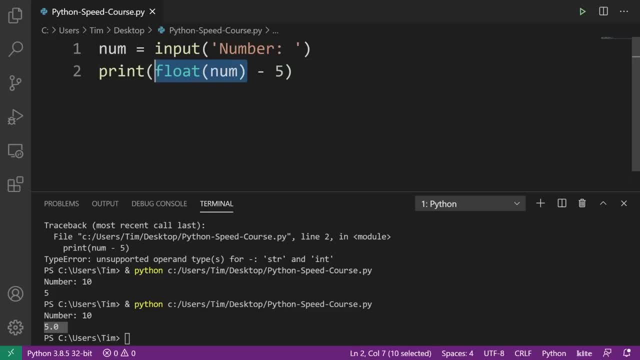 the operand, So on the left or right hand side of the operator, then you are going to get a float result back. All right, That is all I wanted to show for this. Now let's move on. So the next thing I want to cover is: 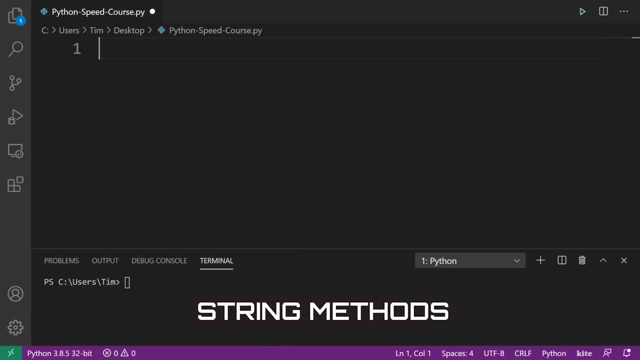 something called string methods. Before I do that, though, I need to define what a method is. So let's create a variable. Let's make this equal to hello, and we can just say hello equals the string Hello. I want to show. 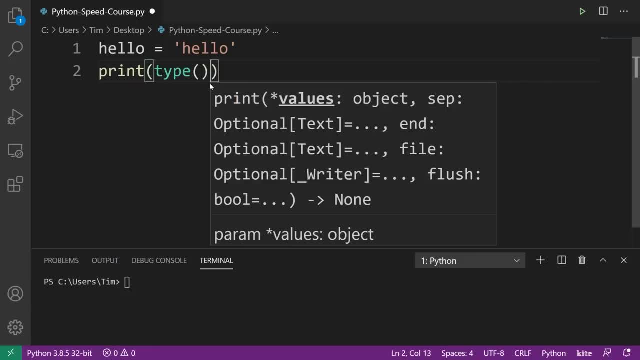 you this function called type, which will tell us the type of a variable. So if I print the type of hello, well you can imagine what type this is going to be. It's simply, it's data type. Let's have a look here. We 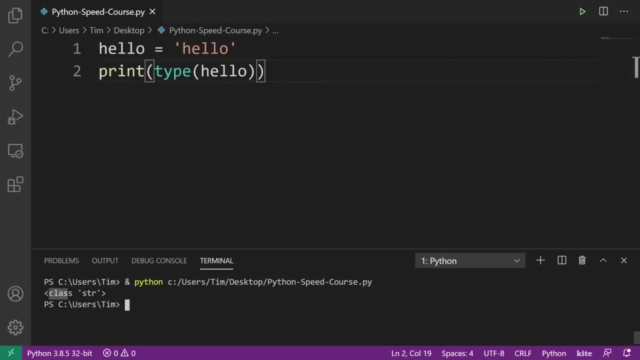 get to class string. You can ignore the angle brackets in the class. If you're more advanced, you probably already know what this means. but essentially what this is saying is that this string or this variable here, hello- is an instance of the class string. 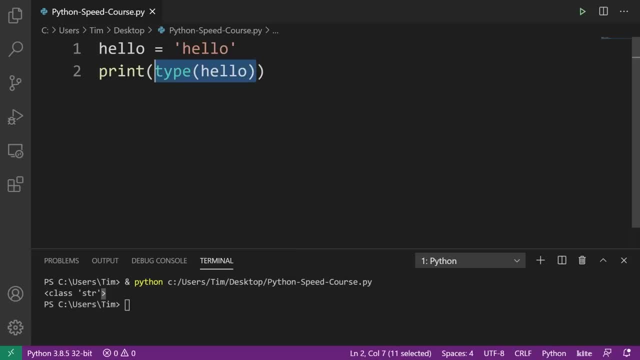 Again, big words. You don't have to know what those mean, but for anyone more advanced, hopefully that makes sense to you. All right, So how do we use a string method? Well, a method on a string. and what is a method? 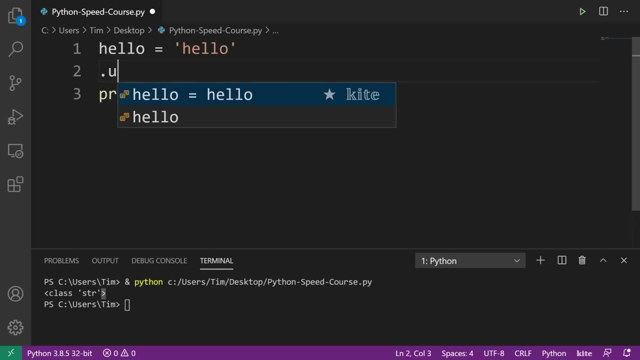 Well, a method simply is something with a dot operator. So we have dot, we have some, a name. whatever the method name is, in this case it's going to be upper, And then we have an open and close, a bracket or parentheses. 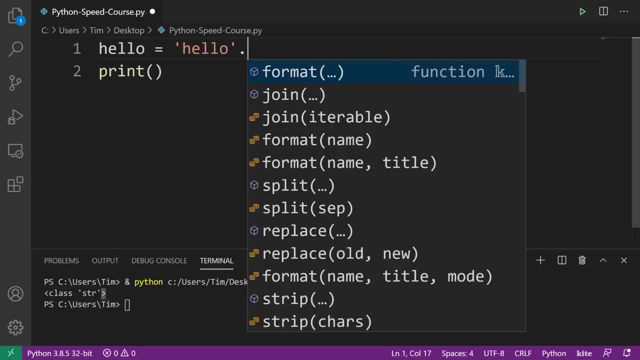 whatever you want to call them. Now I just want to show you what these methods do. So if I say hello dot upper, this is a method that we can call only on strings. So since this is a string I can use. 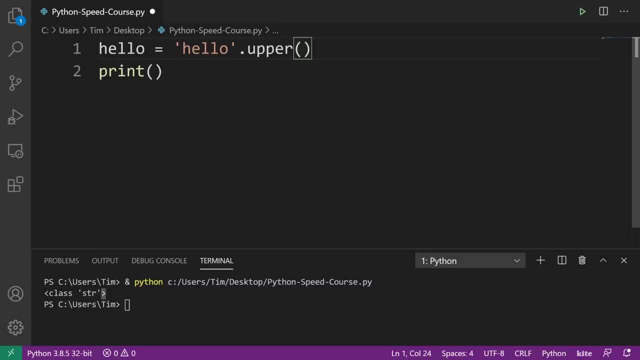 this a dot upper method on it and imagine what this is going to do. What this actually does is it uppercases Or it puts the entire string in completely uppercase. So if I have a look now at hello and we print it out, we can. 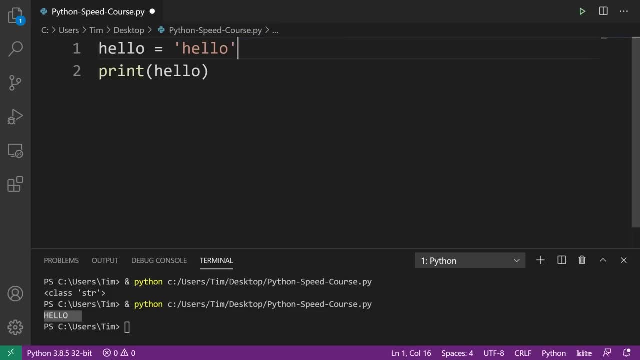 see, we get hello in all capitals. Now I don't need to call it like this, I also can do hello dot upper. Now, the reason this is going to give me the same thing is because, well, this is storing the. 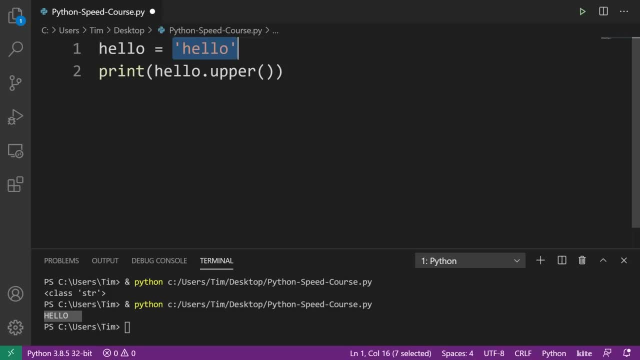 value of the string, which is hello. And then it was just making uppercase right here. Now what happens is says: okay, well, what is hello equal to? oh well, hello is equal to the string Hello. So you can think of it as a. 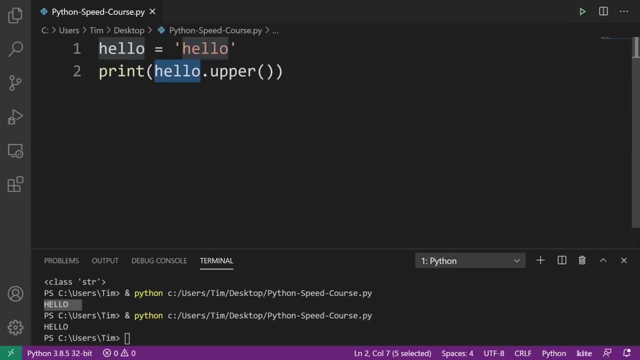 substitution. This string just goes where that is, makes it upper and then prints it out. There we go Upper. Now let's have a look at what dot lower does. You can probably imagine already, but it simply makes the entire string lowercase. These are: 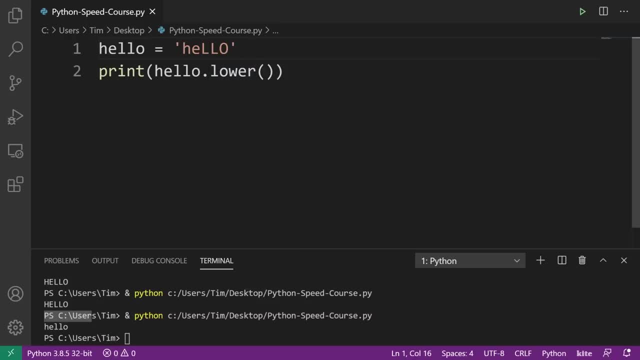 useful when you're getting user input and you want to validate and check if it's equal to something, which we will do later on. So a few other methods we have dot capitalize. You can imagine what this does: It simply capitalizes the first letter in the. 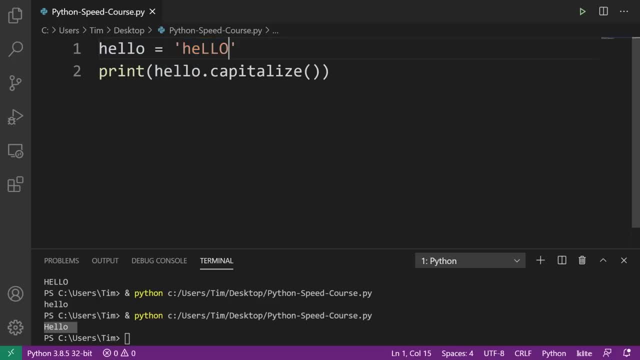 string and then makes the rest of it So it looks good, right? So if I had a sentence I said like hello world, like that, Let's have a look at this, It's going to give me hello world properly. 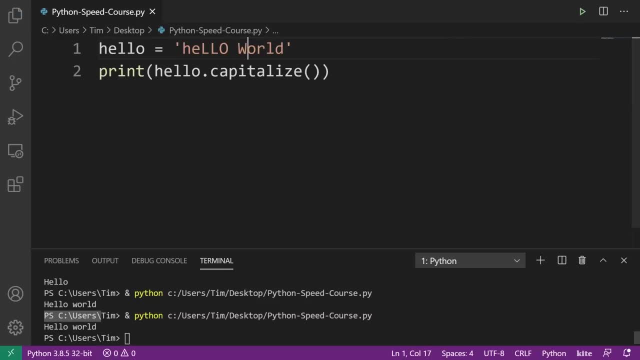 And if I added a capital W like that, it removes that And it just kind of formats it as if a sentence would. next we have this method called count. What count does is it will count a specific string within the string. So it looks for: 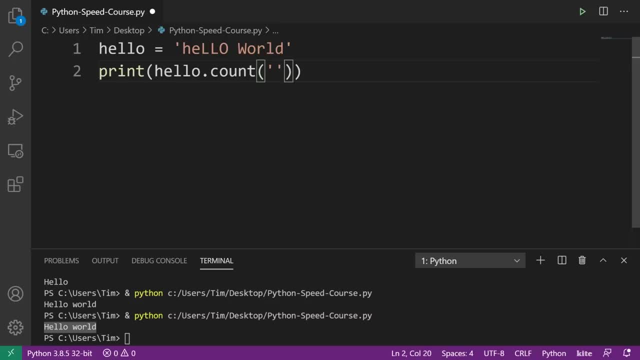 a substring in the string and how many times that occurs. Let's see. I wanted to see how many double L's were inside of this string. Well, I can say: hello doc, count double L, and then that will count and tell me how. 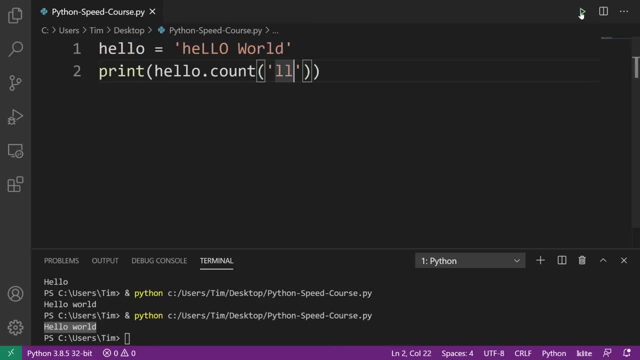 many are in here. Now have a look and guess how many you think are in here. Well, I can say hello. well, there's actually zero. The reason there's zero is because these are capital L's and this was looking for. 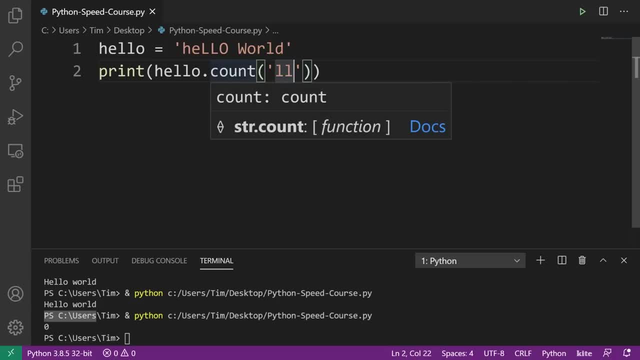 lowercase L's. So that's why it's very important to make sure that you're differentiating between capitals and lower cases, because two lower cases L's are not the same as two uppercase L's. But if I wanted to fix this problem, I can make the 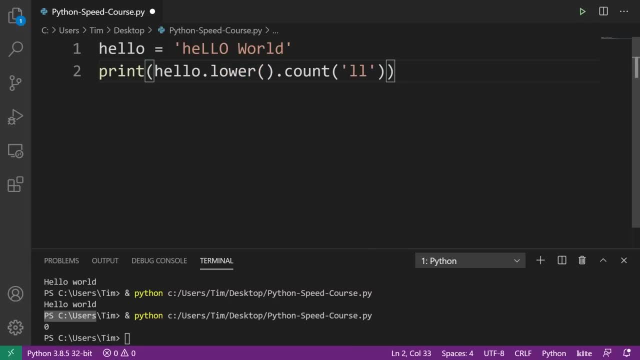 entire string lowercase. So I can say hello, dot lower, and then I could count all of the double L's in the lowercase string. So now let's look at this. In this case we get the value one. let's make this a. 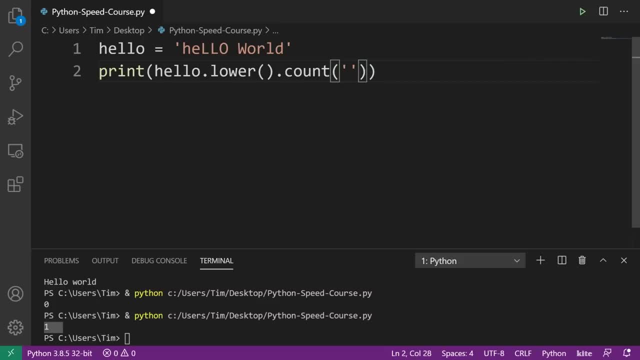 little bit better And let's look for all of the. is there any other ones that we can look for? I guess we can look for how many O's there are. All right, In that case we get two O's, So those. 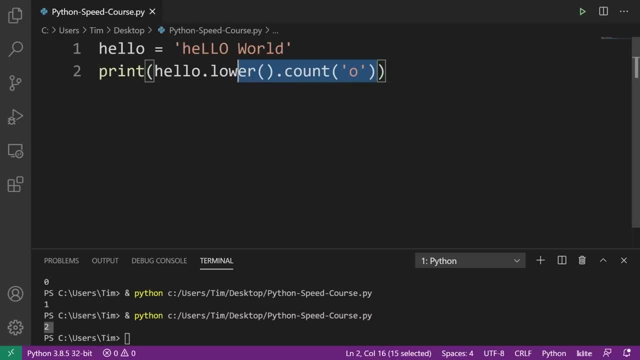 are a few basic string methods. There are some more, but I just wanted to show you how you use these and the fact that you can chain them on each other, Cause what happens is this will return a string. You can imagine that the substitution of this: 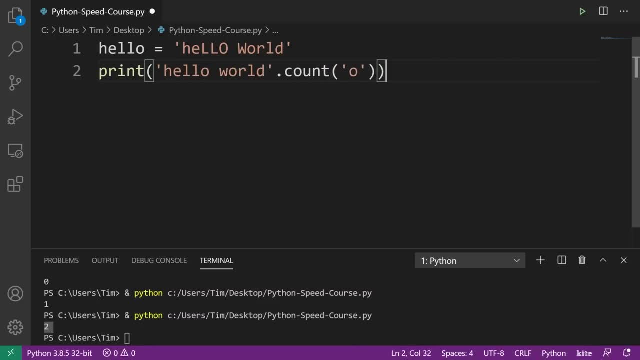 just looks like, um, you know, hello world, And then it's going to count all the O's inside of hello world and returned to us that value, which in this case was two. All right, So now we're going to move on to. 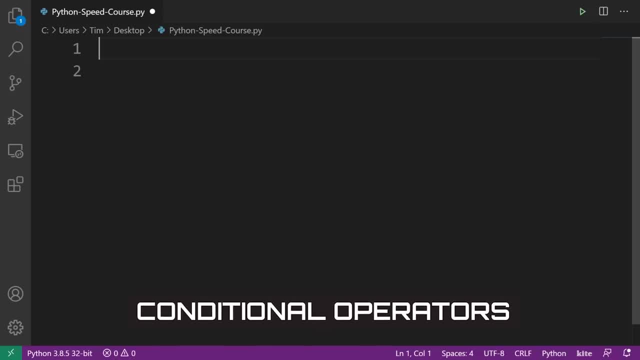 conditions and conditional operators, And before I mentioned that, I just want to go over Something that I forgot in one of the previous sections. this is simply string multiplication and string addition. This is important, So I'm just going to cover it quickly. but 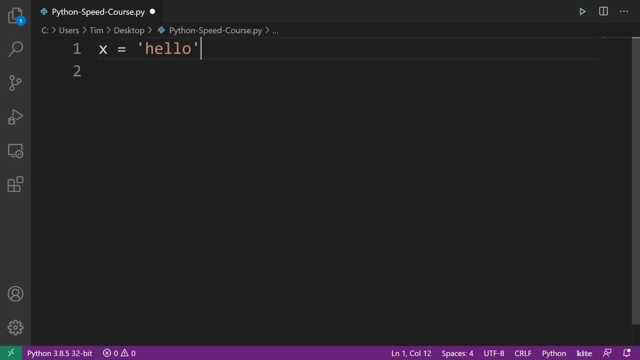 essentially, let's say I have a variable and that's equal to hello. So X equals to a low. have another variable And this is equal to. actually we can say three. Well, there's this cool thing in Python, but what I can? 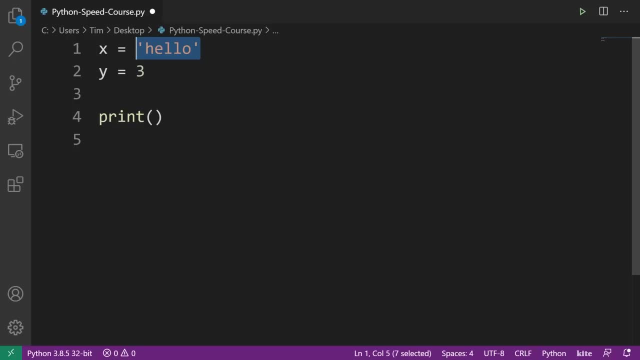 actually do is multiply a string by an integer And that will simply repeat the string, the integer number times. So if I say X multiplied by Y, even though these aren't the same data type, which I said before, might cause problems since it's a 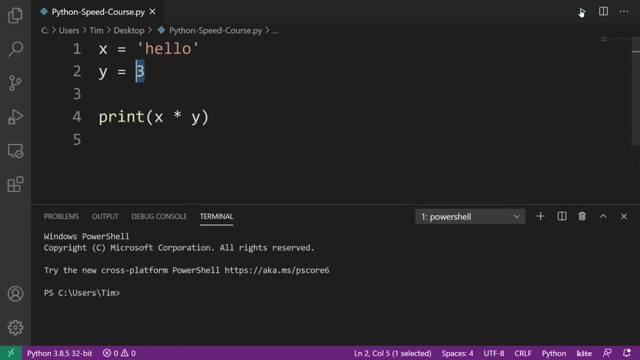 string and it's an integer and the string is on the left-hand side. we can do this. So I can say this: gives us hello, hello, hello, because we multiplied the string by the integer. So just something to keep in mind that we also can. 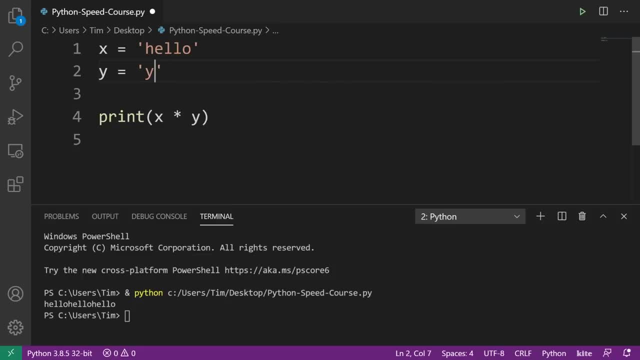 add two strings together because that actually makes sense. So if I say hello and then I say yes, well I can add these two together. This is known as a concatenation. So let's have a look at this and I get hello. 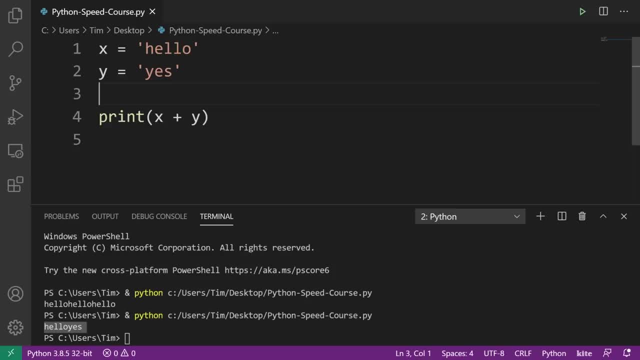 And then, yes, so you can do that. You can add two strings together and you can multiply a string by an integer. Just need to throw that in there, because that obviously is something that's important to understand. All right, Next we're going to 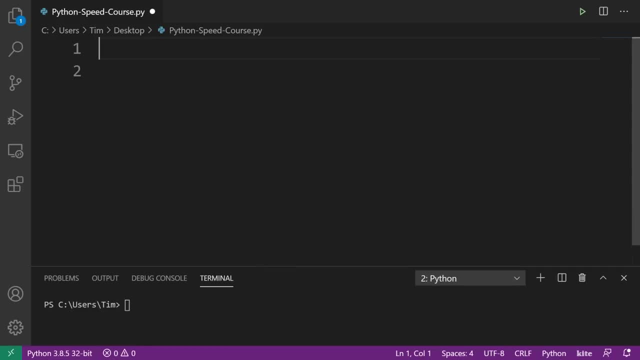 talk about conditions and conditional operators. So a condition is simply something in Python that evaluates or compares to variables or data types and returns to us either a true or false value based on the comparison. So to you know, give you an example of a. 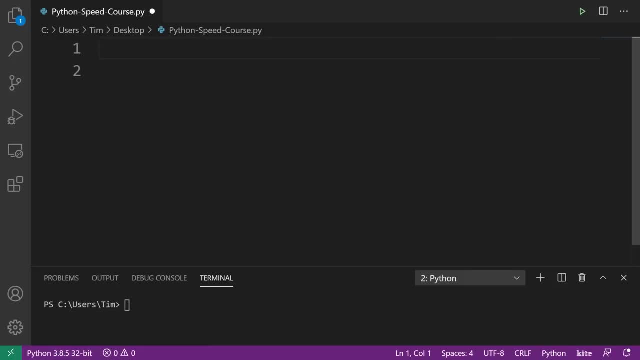 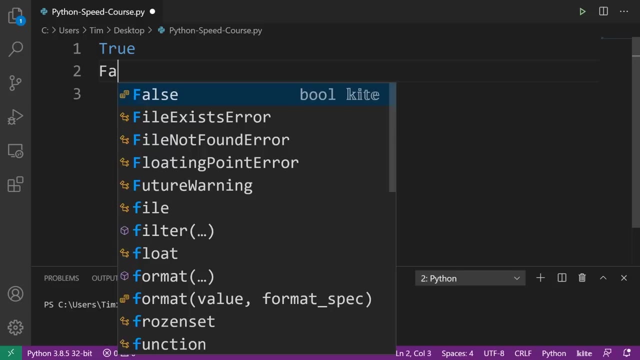 comparison: is X equal to Y? is X less than Y? Those are comparisons And the answer to that is either yes or no or, in our case, true or false. So we have that true And we have these falls. This is Boolean. 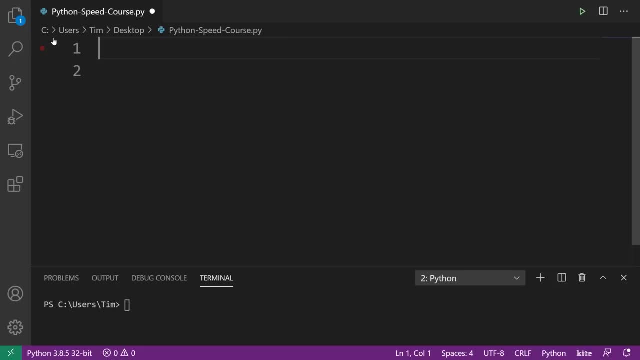 So the result of the comparison is simply a Boolean value. All right, So let's look at what these operators are. We have two equal signs which checks for equality. is the left hand side equal to the right hand side? We have not. equal to which. 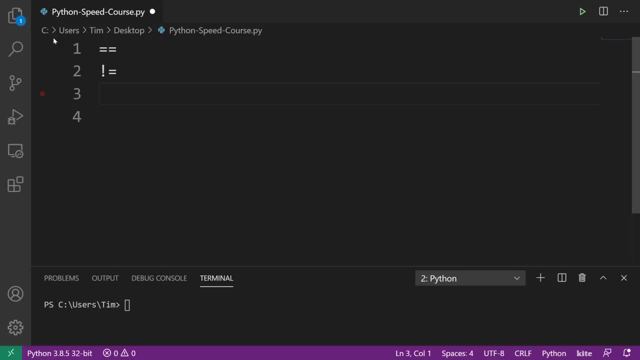 checks for inequality. So is the left-hand side not equal to the right hand side? We have less than, or equal to greater than, or equal to less than and greater than. that was a few other random ones. We're not going to go. 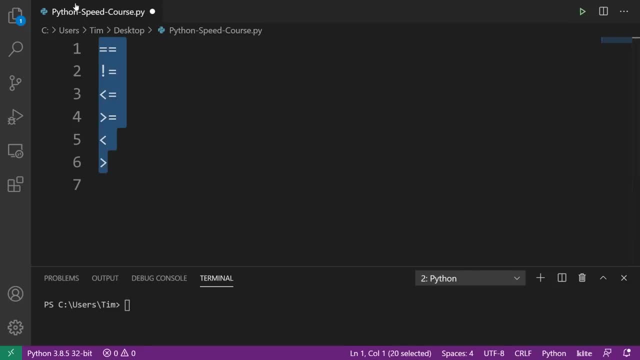 through those. but these are the core conditional operators. And let me show you an example of condition. Let's say I have X equals hello and Y equals Hello. I want to check for the comparison So I might do something like print: X equals equals. Why are 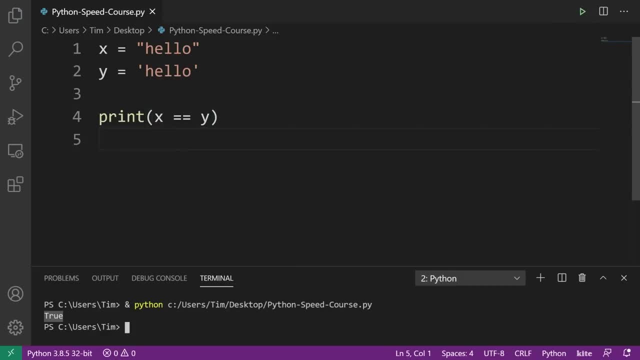 these two things the same? Let's see. Yes, they are. We get the value true. Now let's do the not equal to sign. Are these things not the same? No, they're not, So we get false, That is. 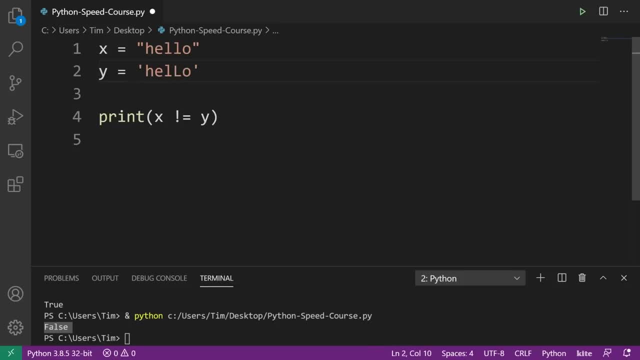 the basics of checking for equality. Now, what if I add a capital L inside of the string? Well, we know that lowercase and capital L's are different. So if I do this, uh, we get true, Which means no, these: 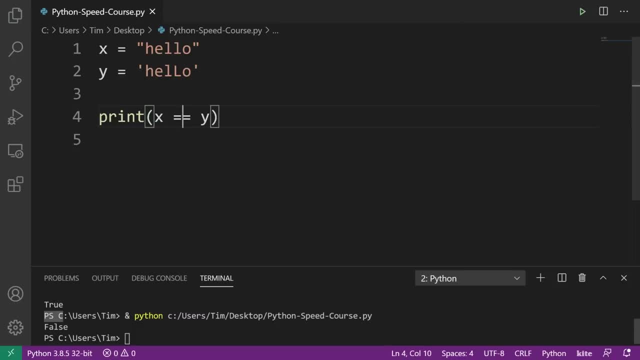 two strings are not the same, They are different. If I do double equal sign, then we get false. Now, interesting thing with strings, we can actually compare them using the greater than sign and less than sign. Now, it's not super intuitive, So I have to. 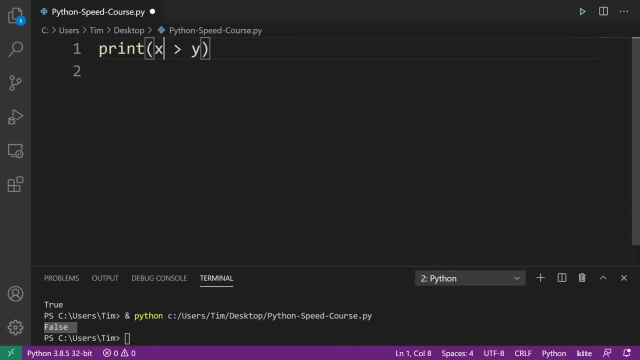 kind of show some more primitive examples here to give you an illustration of how this works. But if I have something like a and I say is a greater than, let's actually go with capital Zed, What do you think? the answer to that is: Well, that's. 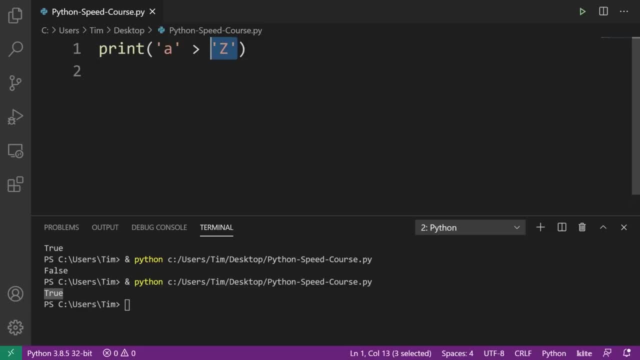 actually true. Now, the reason for that is, every single character inside of Python is represented by what's known as an ASCII code. We actually have a look at what this ASCII code is by looking at what's called the ordinal value of a character. So if I print, 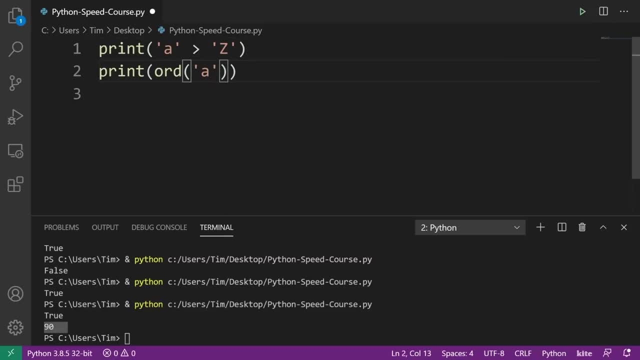 out the ordinal Zed, we can actually see that that's 90. And if I print out the ordinal of a, we can actually see that that's 97. So what that's telling us essentially is that this uppercase Zed is actually represented. 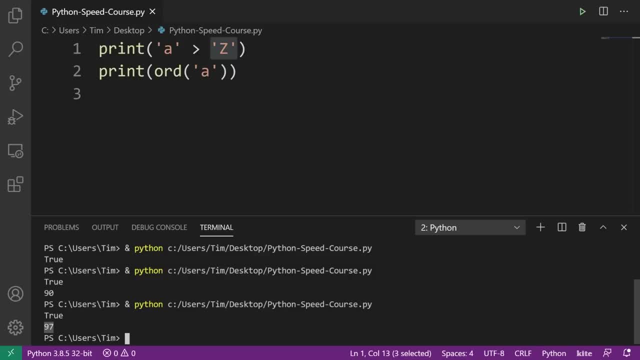 by the number 90 and the uppercase, or sorry, the lowercase, a is represented by 97. So what we do is we would compare the two ordinal values of these character characters and see that, well, actually a is greater than Zed. Now, if we do this, so I 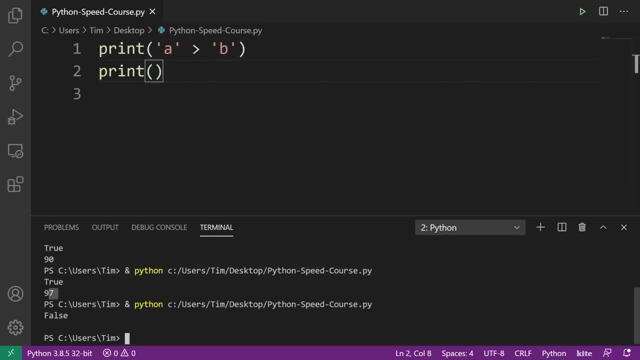 say a greater than B, then that's going to be false, because B is actually represented by 98.. There is some logical ordering for these characters, but I just want you to understand that we can compare strings using greater than less than equal to all of those. 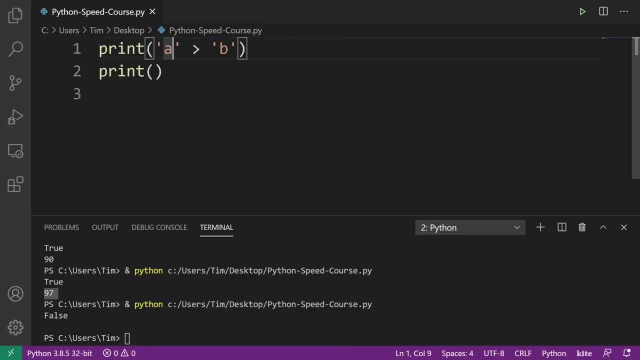 but just understand that we're comparing the ordinal value of the strings. Now, let's say we have something like a- B. what we're going to do is simply just go from left to right and compare all of the characters. So we would say, okay, is a greater. 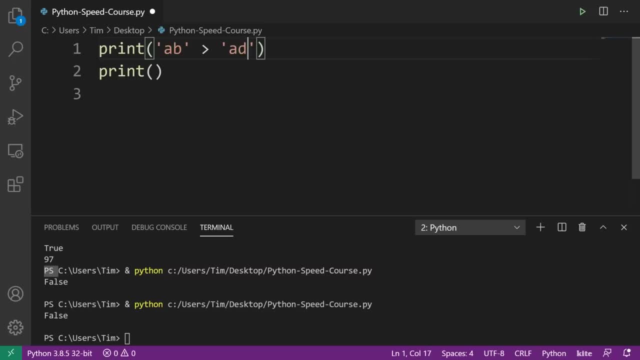 than B. Yes, it is a matter. Imagine these two were the same, So we had a and then we had D, like that. If these were the same, then we would go on and compare the next character, which would be B, in this case we. 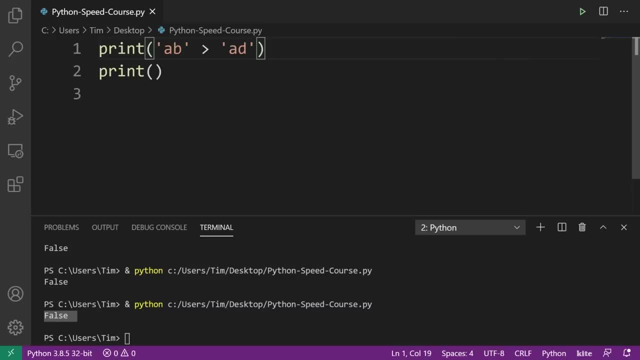 get false because obviously the D is greater. All right, So that is how that works. Now let's just show a few examples of numbers. Let's just say: 7.5 equals equals seven. Is that true? Obviously that's false. Let's say: 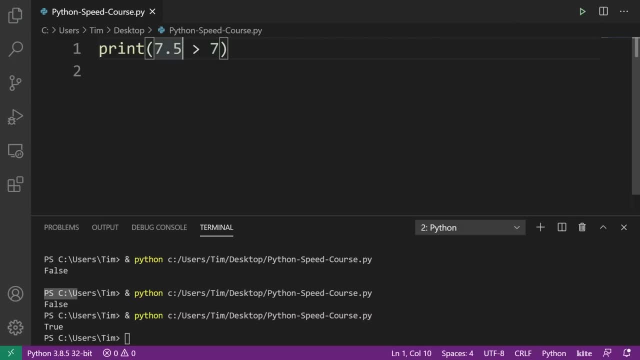 7.5 greater than seven? Obviously, that's going to be true. And what about 7.0 equals equals seven? Have a look at that. What do you think We get true? All right, That is the basics on the. 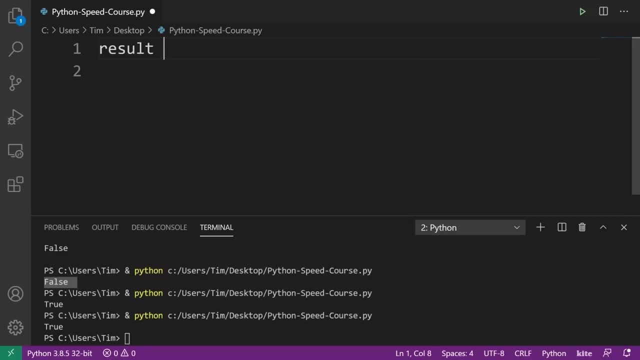 conditional operators and conditions. Of course you can store these things in variables. I can say: result equals six, equals equals six and print result like that And we get to the value True. Okay, Let's move on now to chained conditionals, So a: 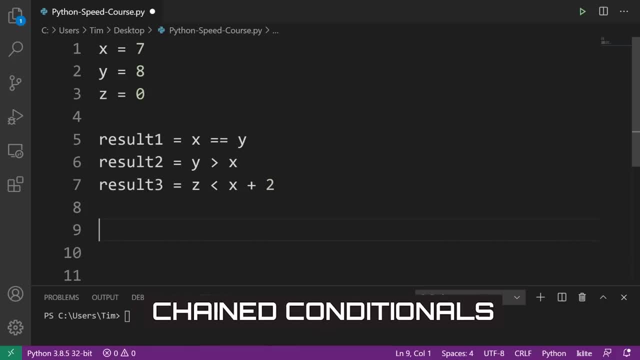 chained conditional is essentially combining multiple conditions together to create one larger condition. What I have right here is a basic example. I have three conditions right. I have result one, result two and result three. result One says is X equal to Y. result Two says is Y. 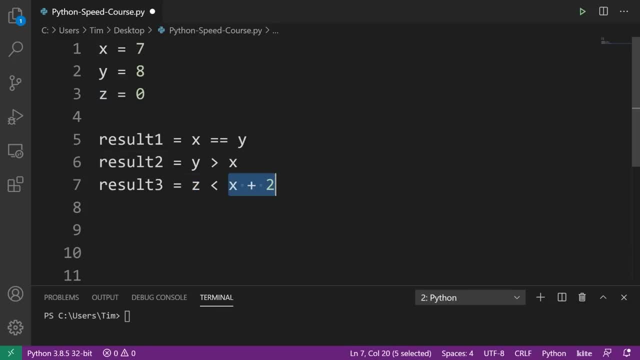 greater than X, And this one said is Zed less than X plus two. You can imagine that these have brackets around it. It works the same. So all of our conditional operators have a lower precedence than all of the arithmetic operators. So if I do something like 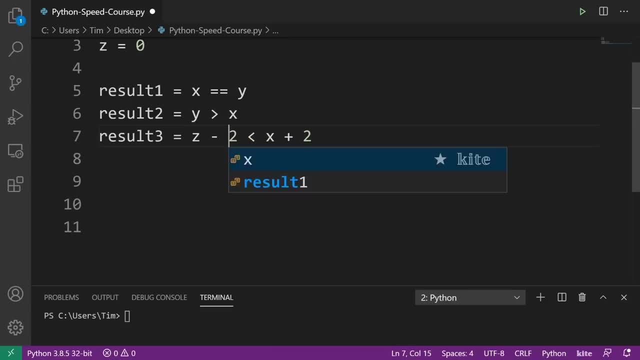 Zed minus two. less than X plus two- well that's not going to say Zed- and then negative two, less than that. It will evaluate on the left-hand side and it will evaluate on the right-hand side, And then it will combine and use. 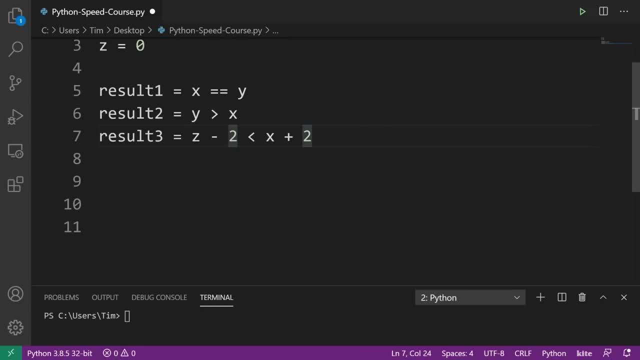 sorry, this conditional operator. So hopefully that makes sense. but just keep that in mind, that you can actually write expressions on each side of a conditional operator. Okay, So now that we have that, essentially what I want to do is say, okay, how can I? 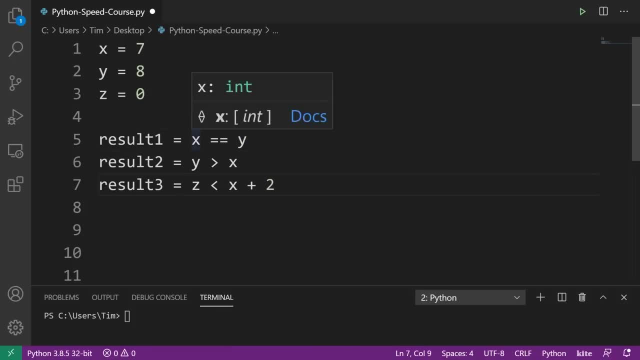 make a condition that uses result one, result two and result three. So obviously all of these are equal to true, false, true, false. They're equal to something like that. So what I can actually do is use a three separate keywords. So, and, or: 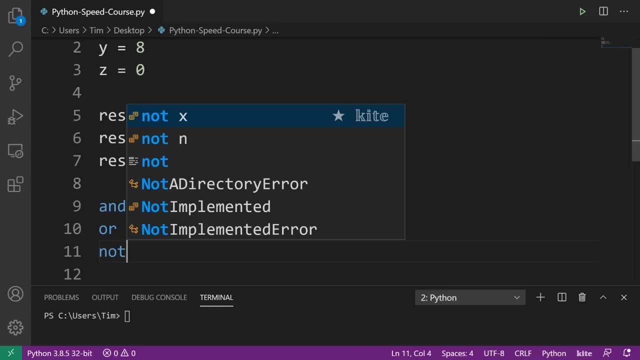 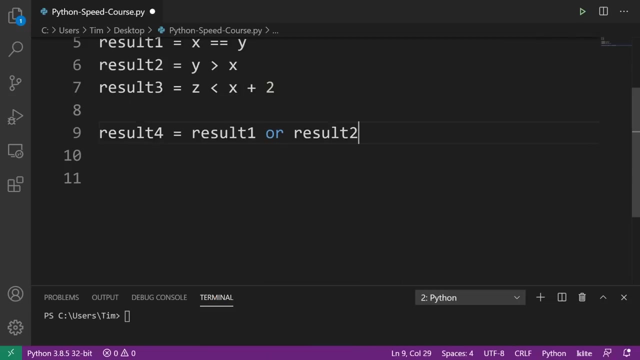 oops and not. So these three words are what I can use to chain conditionals together and create larger, larger conditions from specific conditions themselves. So what I can do is do something like this. I can say: result four equals result one or result two. Now what? 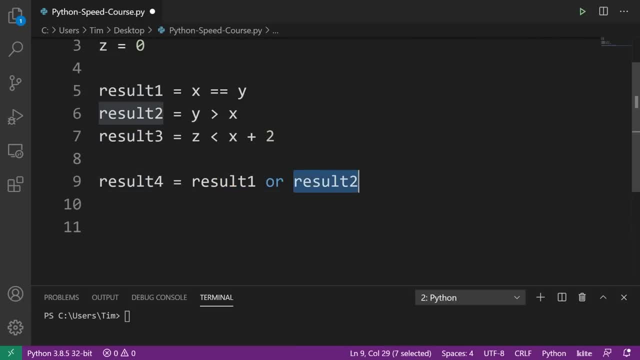 does the or operator do? Well, the left-hand side and the right-hand side of or have to be a true or false value, which they are, because these evaluate to true or false. What or we'll do is it will look at. 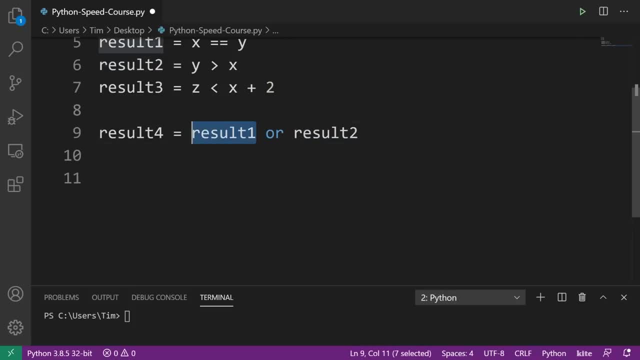 the left-hand side and right-hand side, We'll say okay, if the left hand side is true or the right-hand side is true, this whole condition is true. Of course, if they're both false, that's the only situation where this 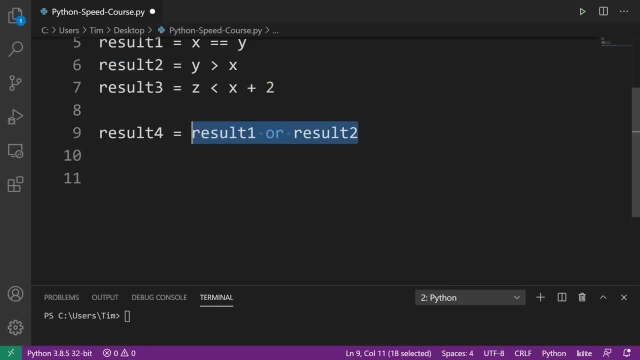 whole condition here is going to be false. So in three scenarios- cause there's four possible scenarios here- it's going to be true, And the other scenario, it will be false. So if both of these are true, obviously at least one. 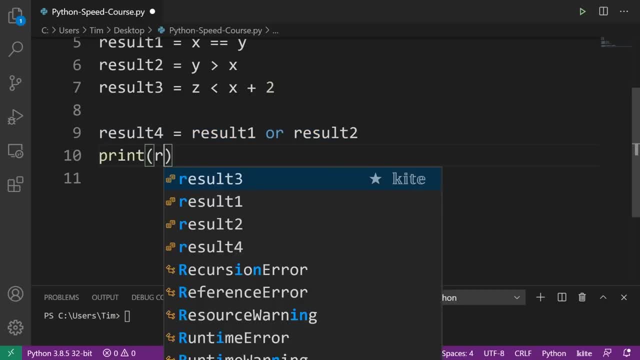 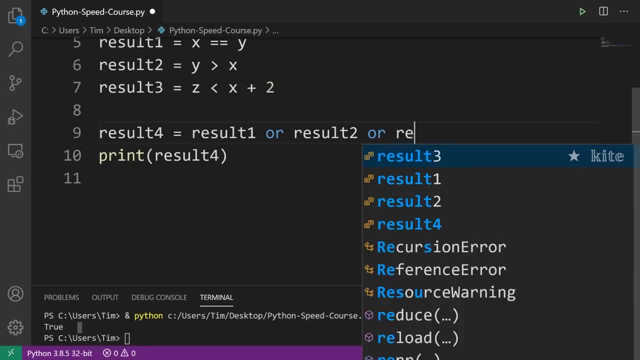 of them was true, So that evaluates to true. So let's actually just print result for and have a look at it. Great, We get true. Now what we can do is we can add another, or, if we want, and we can say: 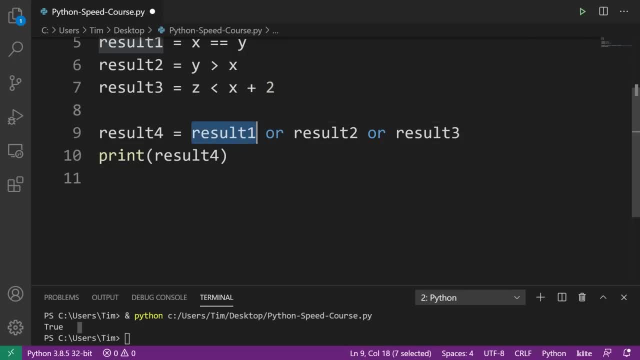 result three. Now what this says is okay. if result one or result two or result three is true, this whole thing is true, which of course it is. Now let's see how we can combine other stuff into this We can actually use. 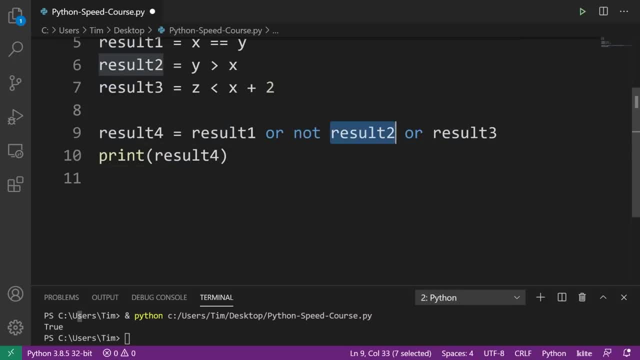 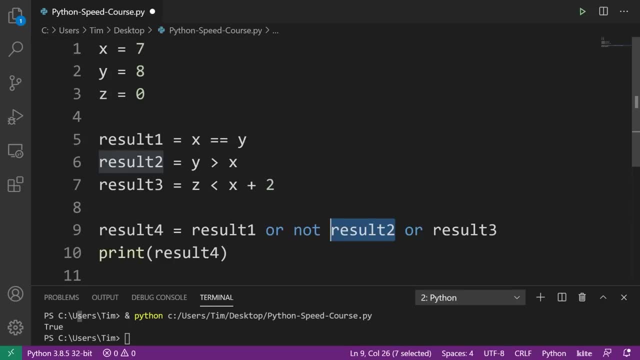 this, not keyword. What this does is it takes whatever is on the right-hand side of it. So in this case, it's going to be a true or false value and just flips it. So in this case, if, if, result two: 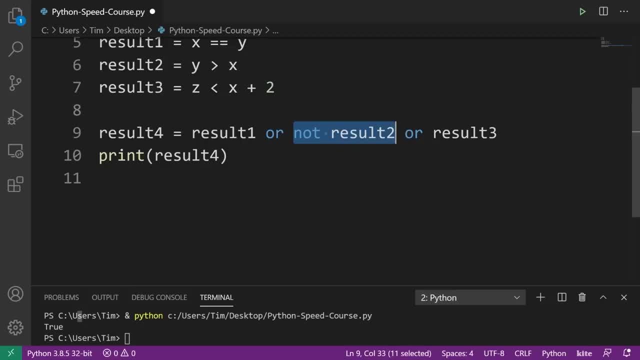 is true, which it is, it's just automatically going to become false. So if I actually I can show you on a more basic level. uh, if I just print a set of result four, I print not true, like that, This will print. 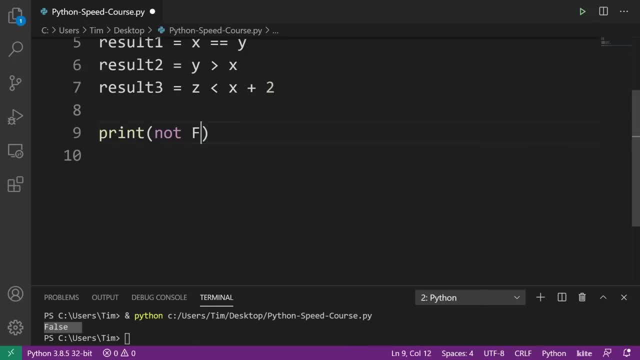 the value false, which you can see down there, And if I print not false, then this will print true. Now what I can do is do something like this: I can say not false or true, So let's have a look at. 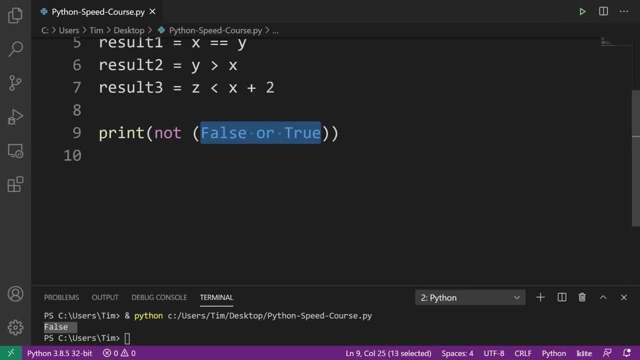 that, And there we go, We get false. So it takes whatever this is which is true, And then it just reverses it and makes it with the knot. Now, those are two that we've talked about. So, or, and not now what? 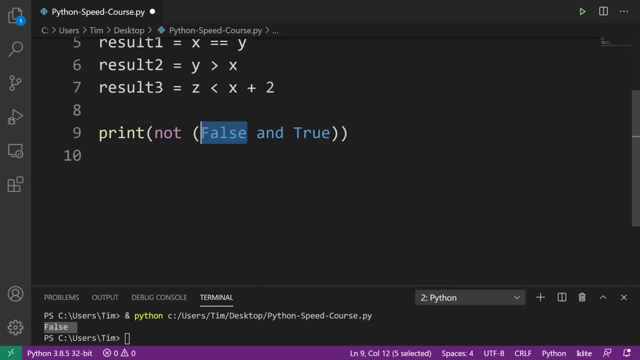 about and so and essentially says: okay, is what's on the left hand side and the right hand side True? If both of it is true, they are true. The whole condition story is true. Otherwise, it is false. So only in one. 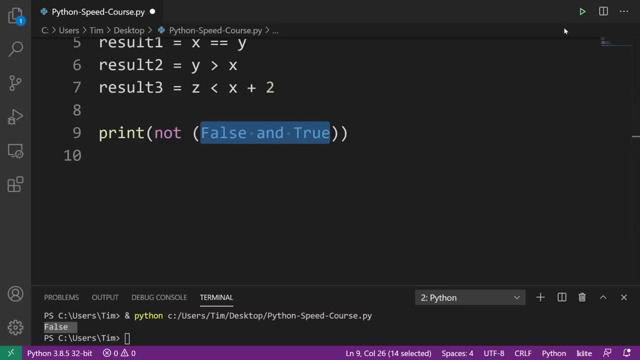 scenario out of the four possible scenarios here, with two variables or two values on the left and right hand side. is this going to be true? So let's have a look at this and we get true, because obviously this is false, Then we not it, And that turns to. 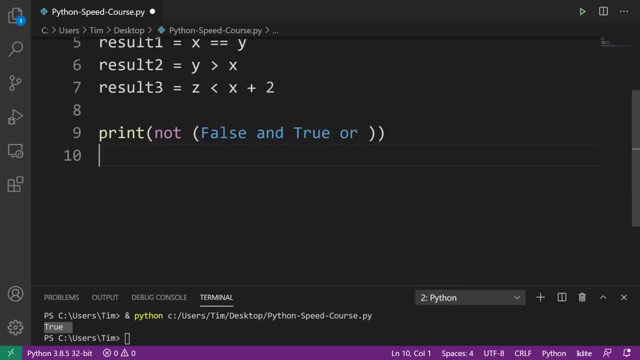 true. Now, of course, we can do a combination of and and or. now, when we use these combination of different things, right? So not and or, we have to know which is going to come before what, so kind of in the. 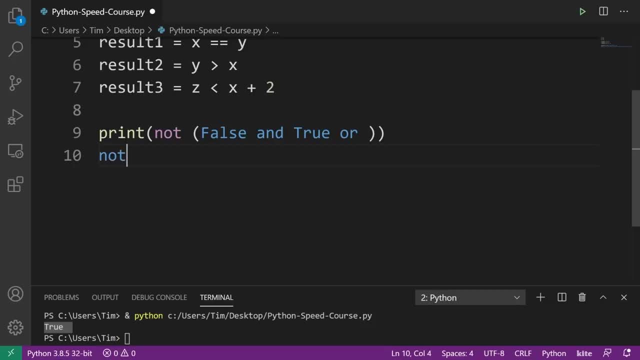 order of operations. Now, the way it actually goes is not is first and is second and or is last. So just keep that in mind because that will be important based on the way that you write your expression. So, essentially, if I say false and true or true, 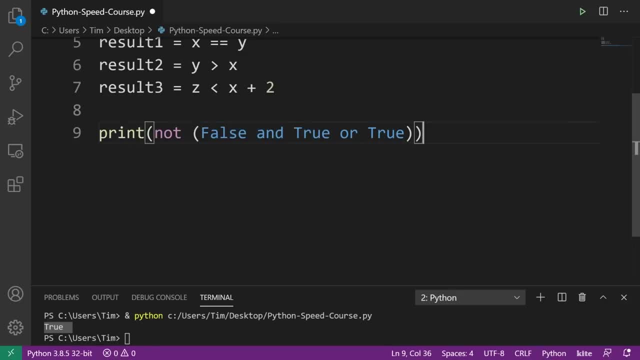 then we're we're going to actually do is evaluate the false and true first, And then we will evaluate the or of whatever this is And then that. so in this case this will be false. So then we would get false or true And 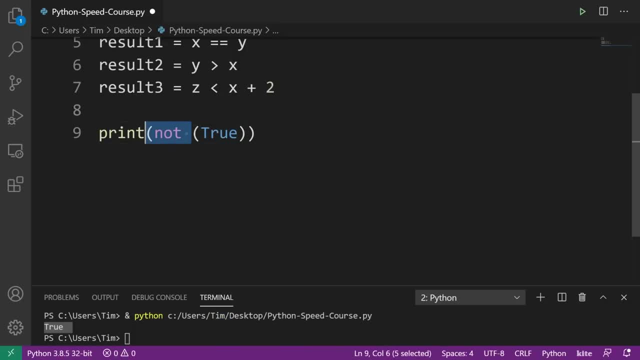 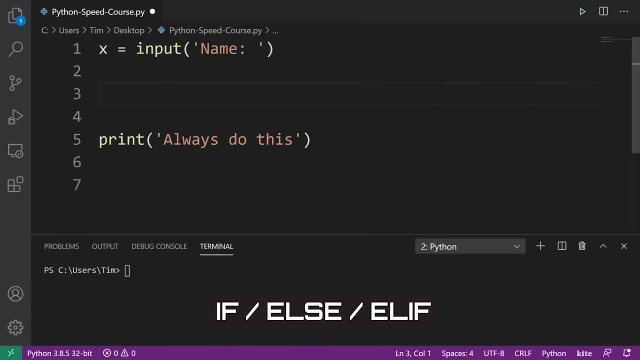 then this would turn into true, Then we would have the not and that would turn that into the false. So now we're moving onto the fun stuff, which in my opinion, is the if, else, if and else statement. if this essentially allows us to, 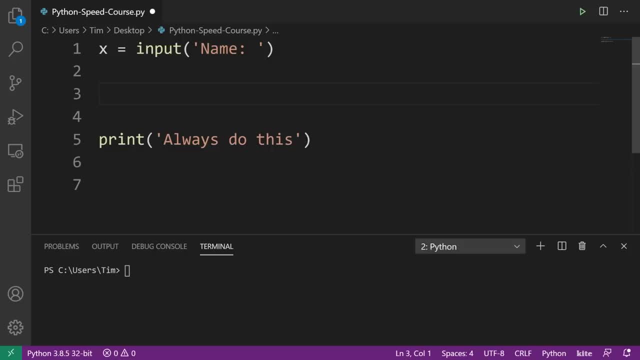 actually check if something occurs or if a condition is true, And if that is true we can do something specific. Otherwise we might not do anything or we might do something differently. So for the example I'm going to do here, I want 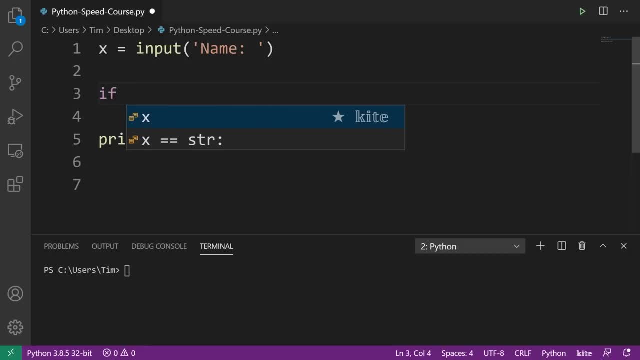 someone to type in their name and I want to say if their name is equal to, in this case, Tim, I will tell them they are good at Python. I don't know Something random, So in this case, to do that. 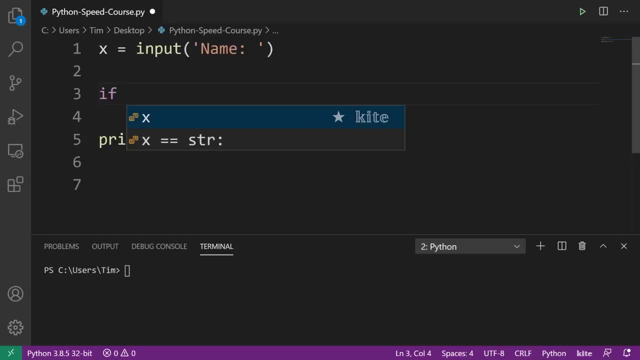 what I will start doing is writing an if statement. So the syntax of an if statement is if condition, like that- I know that's spelled wrong, but that's fine- Condition, colon, indented block, whatever I want to happen in the end- dented block And then 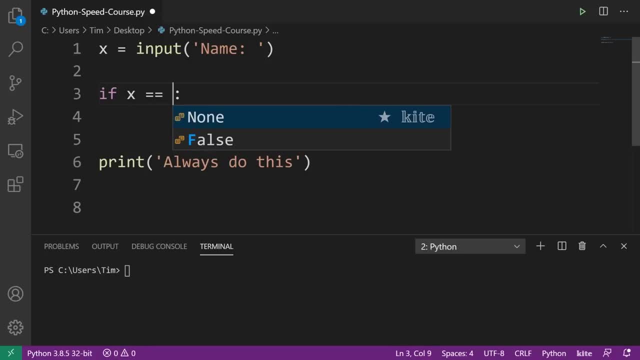 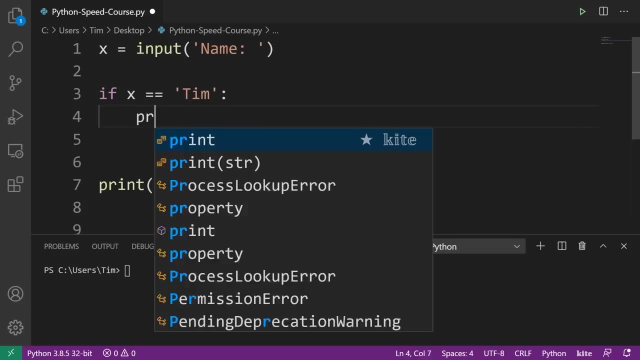 that is the basic syntax of the if statement. So for here, if I want to check if X is equal to Tim, I will say: if X equal, equal to, and then the string Tim with a capital T. I will simply print you. 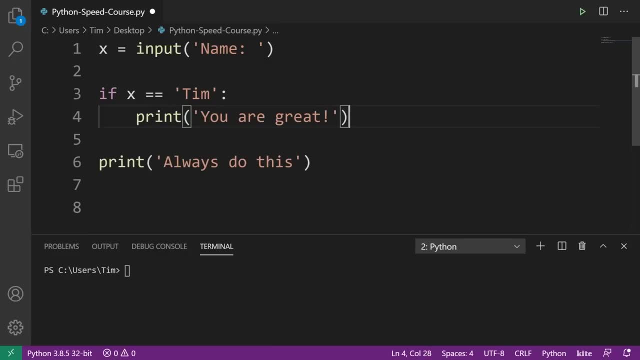 Are great. So now what will happen is: if, and only if, X is equal to Tim, will I print: you are great now in any situation. So regardless of if the name is equal to Tim or not, I will always do this. So I 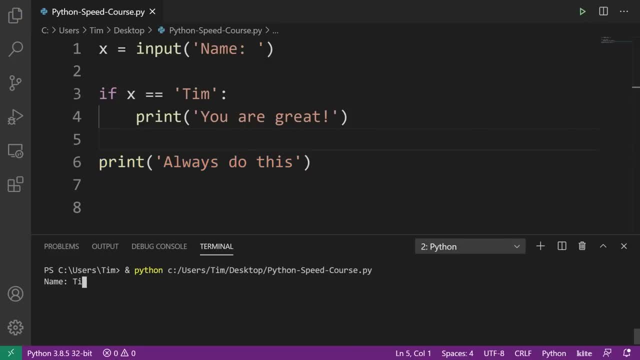 will print that statement. Uh, hopefully that's self-explanatory. So let's go ahead and do Tim. We can see you are great, Always do this. Now let's do another name. Let's go with Joe and it says: always do. 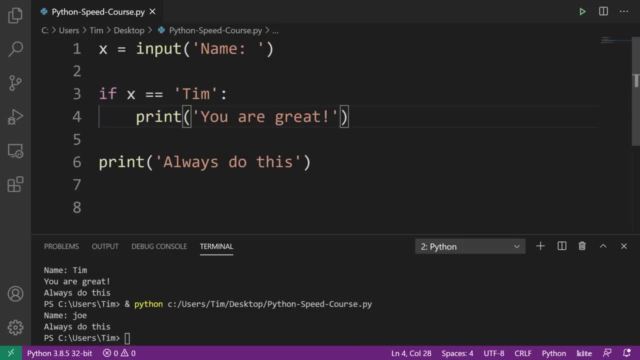 this. It did not print this statement. Now the addition to the if statement is: of course I can add more stuff underneath the indented block, So I could do another print statement and that would add a space. So let me actually just show you. 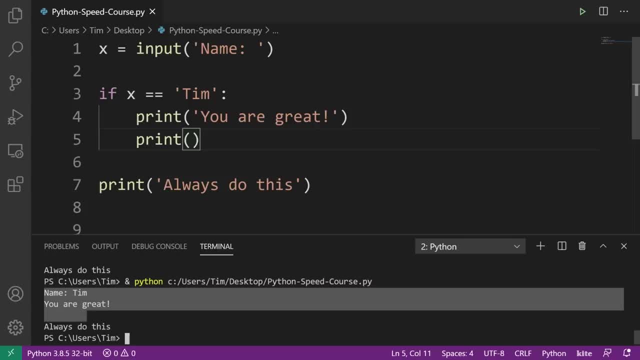 how this works. If I do, Tim Now, you see, we get that space by just printing an empty print statement, essentially Okay. Now, what we can do, though, is we can say: okay, how about? I only want to print a, you are? 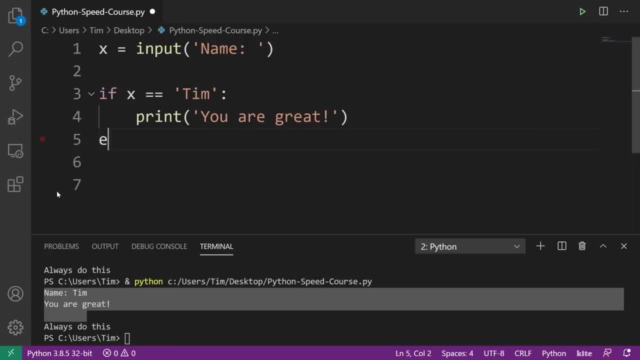 great, or I want to print some other message. I don't want to print two things. Well, what I can do is I can print, I can add this, else. This else must come after an if statement, And essentially, what allows me to do is say: okay. 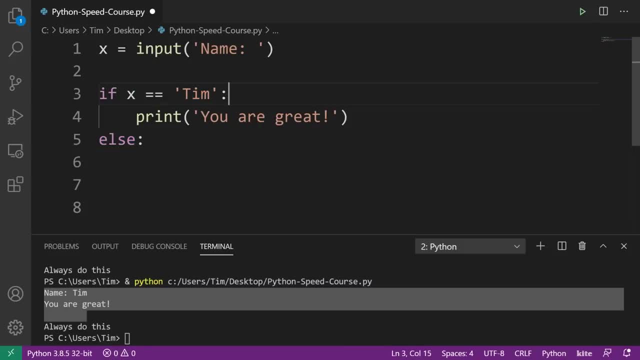 if this isn't true, do this. So it's an if else, right. If true, do this, otherwise do this. Never will I do both, So in this case I'll just print. no, you know, not very. 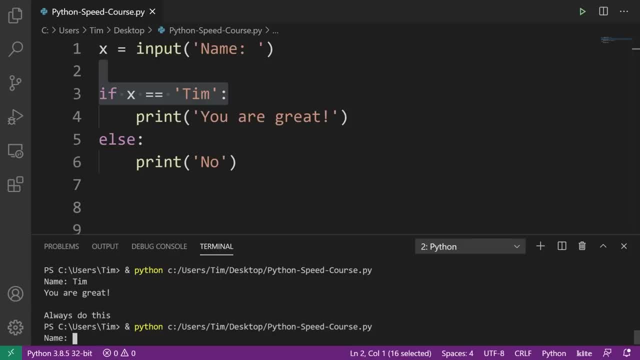 intuitive or it doesn't really make much sense, but that's fine. So now I'll go ahead and I'll say name. Tim says you are great, And let's actually just go with no, And then it prints out No, All right. So 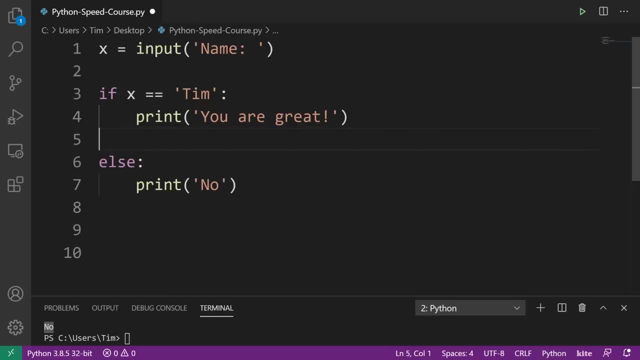 that's the basics on the if else. now let's say we actually want to check multiple things, So maybe we want to check a bunch of different names And if the name is Joe, maybe we want to say: you know, thanks, Joe, I don't. 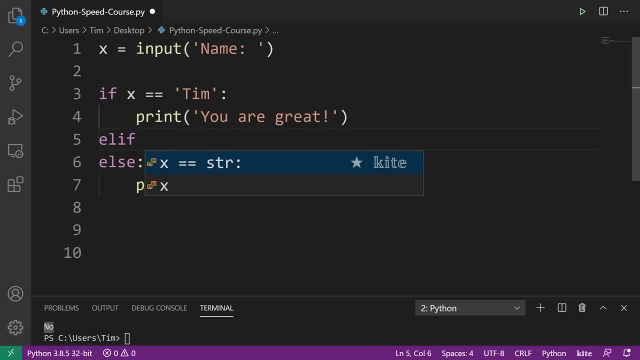 know something random, right? Well, what we can do is use this LF statement. The LF statement can be used as many times as we want, but it must come after an if and it must be before any else's, So I can't just. 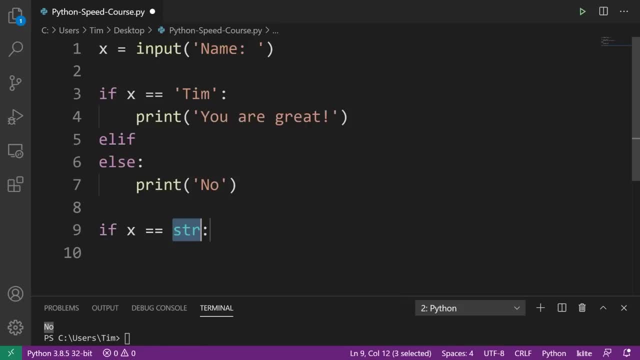 go ahead and start writing these random LFs everywhere only is going to come after an if statement. So there's only ever one if only ever one else, but as many LFs as we want, and you'll see how this works in a. 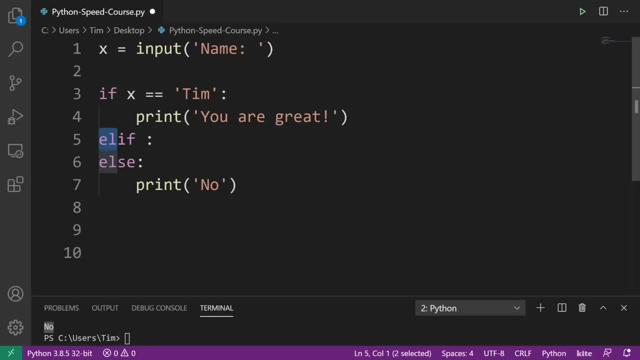 second. So the LF syntax is the exact same, except it starts with the yeah. So I'm going to say LF, uh, X equals equals Joe, And then I'm going to print uh by Joe, Why not? So now, 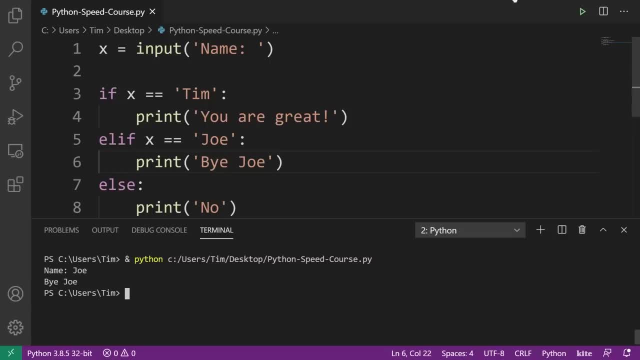 let's run this and let me just show you what happens when I go with Joe. It says by Joe and let's just print something random. It gives us no. no, of course I don't need this L statement. I can use an LF without the. 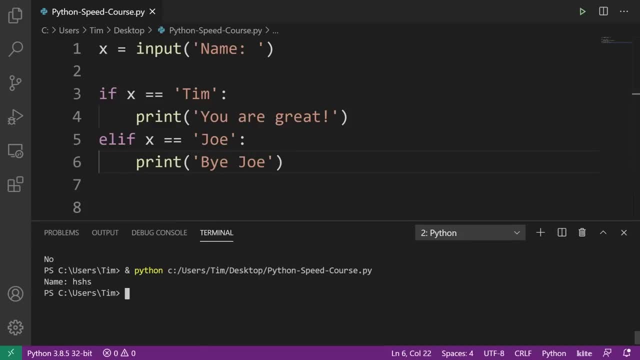 L statement. That's totally valid in this situation. If I do something random, just nothing will happen. But if I put Tim or Joe, then it will give me the valid response. Now let's add another LF. Let's say: if LF X equals equals. 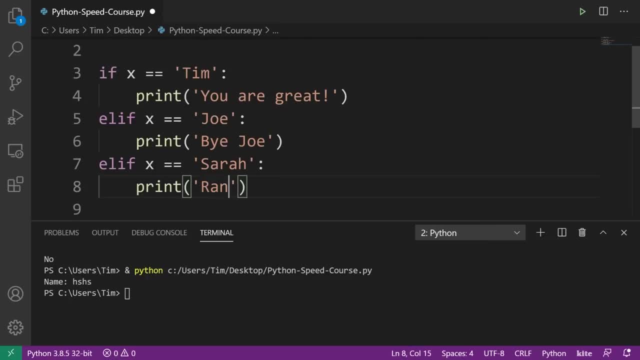 I don't know. let's go with Sarah. Uh, we can print random, Okay, And now let's try this out. And that works. Now, of course, we could add the else at the end, but that is the basic for. 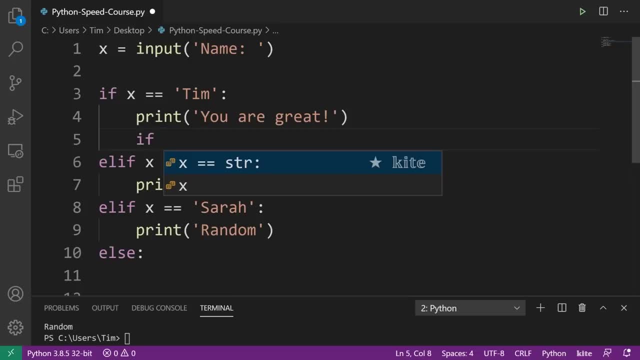 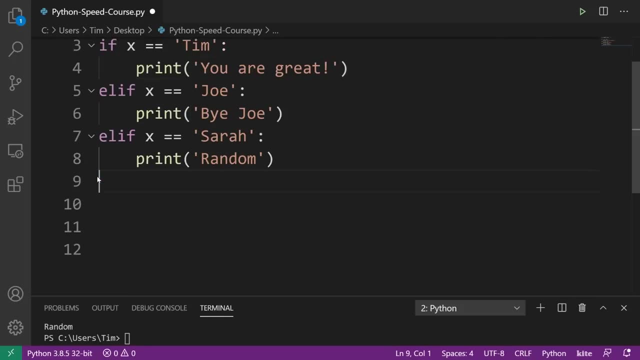 the if, L, if and else. now of course you can chain and add stuff inside of another if statement. I could put another if statement inside of this, but just make sure you keep the indentation correct, because that how it. that is how it. 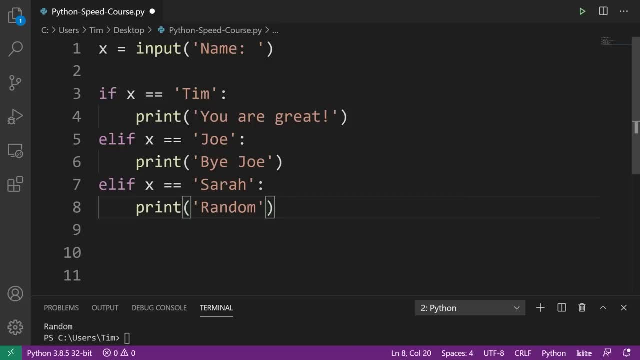 determines what we are going to be printing and what we are doing, If this statement is true. So in these next few sections I'm going to be talking about collections, how we deal with collections, looping over collections and all of that fun stuff. 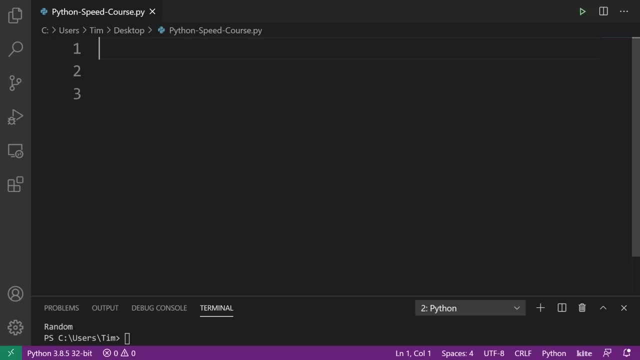 But what is a collection? Well, collection is simply an unordered or ordered group of elements. Now, the two collections I'm going to discuss here in this section is a list and tuples. So if we have a list, a list looks something like this: it is simply: 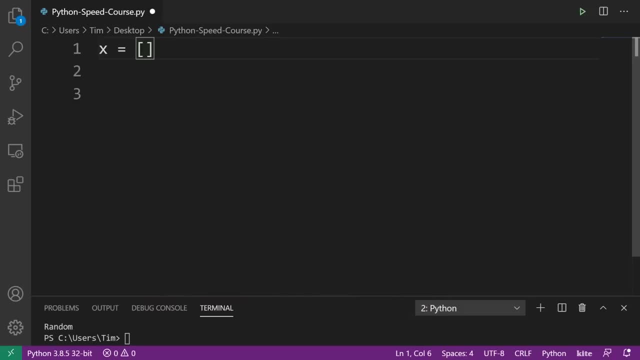 square brackets. Now, inside of the square brackets, we can have a series of elements. Elements are simply some data type, So I could have the integer, for I could have the value true, I could have some string high, and these elements do not need to. 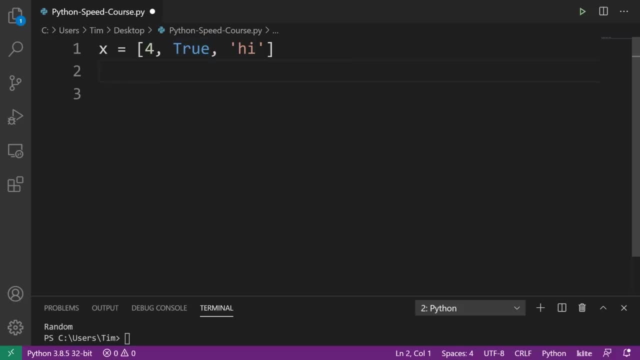 be the same type, like in many other languages. So this is a list, And the way that the list works is that it can store a bunch of different elements. in a list is an ordered collection, which means the order in which we enter things into the 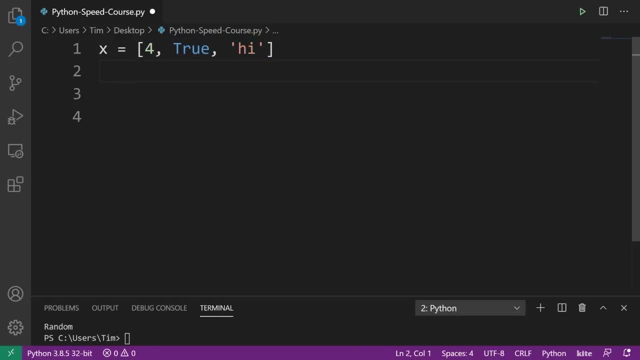 collection matters and is maintained- In fact, it's very important- in the list. So how do I actually access elements in the list? How do I deal with the list? What are some things we can do with it? Well, of course, I can define a. 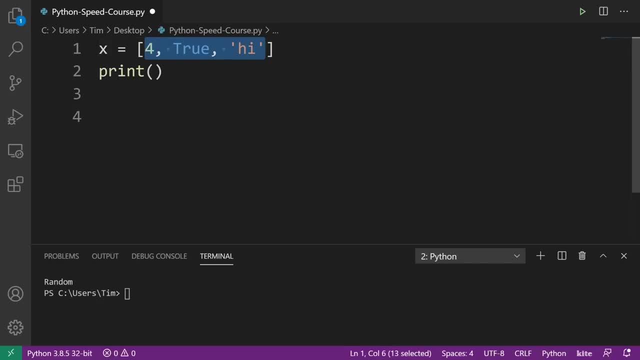 list by simply opening up some square brackets and then finding some elements inside. I also can just leave a square brackets like this empty. That would give me an empty list. The first thing to look at on a list is this function called Len. Len will tell us: 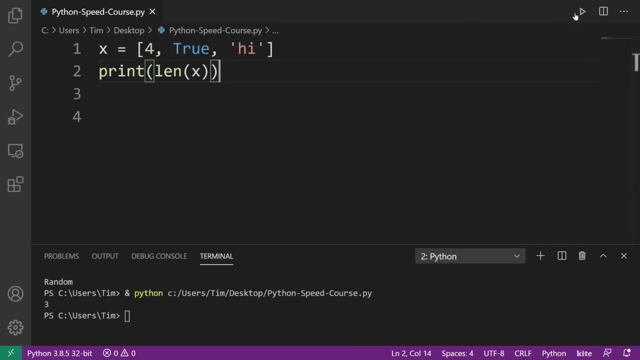 the length of the list. This also works on strings and a few other things as well. But if I look at the Len of X, that tells me three. now just to kind of show you here, if I say Y equals high and I were to look, 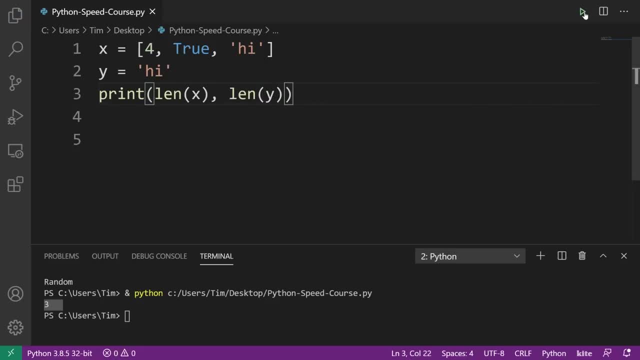 at the Len of Y after I look at the line of X, we obviously get two. So Len is a function in Python that we can use to look at the lengths of stuff. All right, So that is one of the things we can do on a list. What? 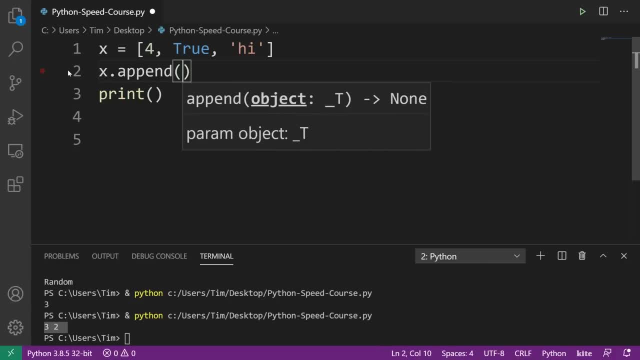 we can also do is we can append things to it. What a pen does is add to the end of the list. So if I want to add to the elements, hello, I can say X, dot, append. Now I can print out X. 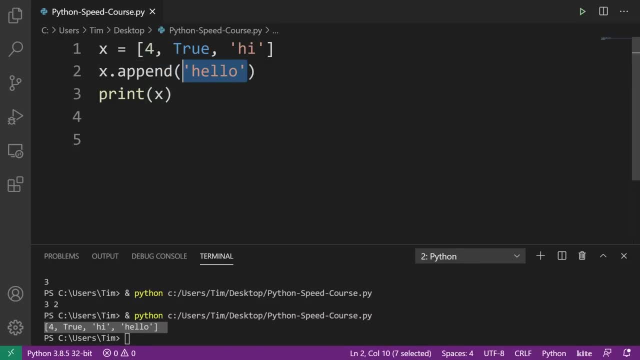 And if we have a look, we get four true high. Hello, Of course we added this element to the end of the list. I can also extend the list by another list. So let's say I have a list here and inside of this, 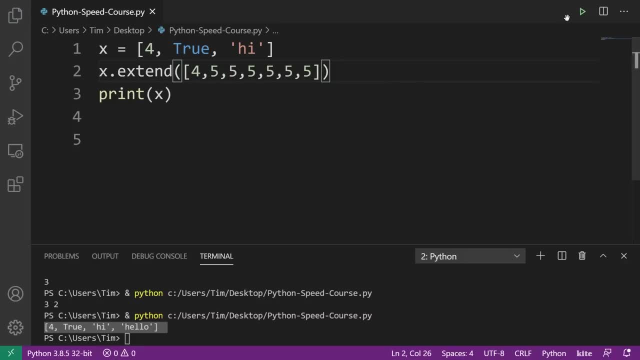 list. I have four or five and just a bunch of other stuff. Well, when I extend it, what that will do is take all of the elements From this list and simply append each of them to the end of the list. So you can. 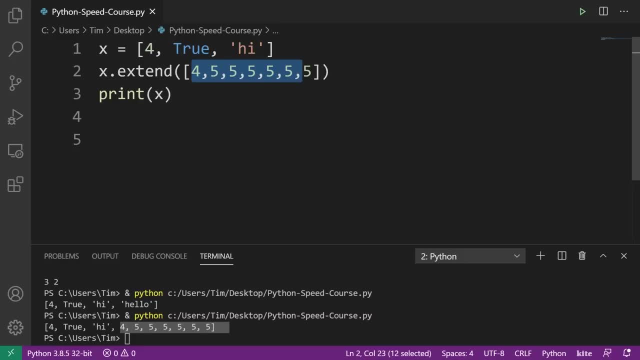 imagine, extend its internal implementation- just loops are all of this- and appends all of those elements to this list. Now, what about removing something or popping something off of the list? Well, I kind of already give a gave away. what one of these 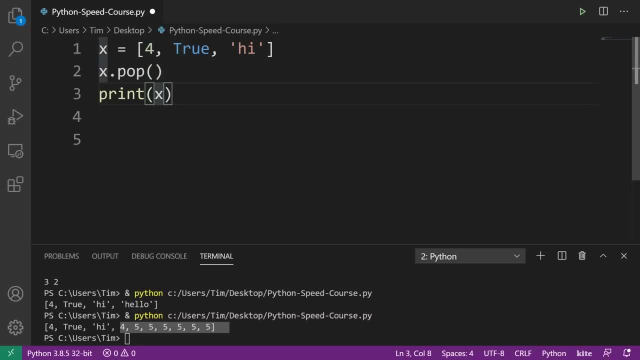 things is, but what pop does is remove and return the last element in the list. So if I actually go ahead and print X dot pop, what this will do is it will print high and it will remove high from the list And you can see. 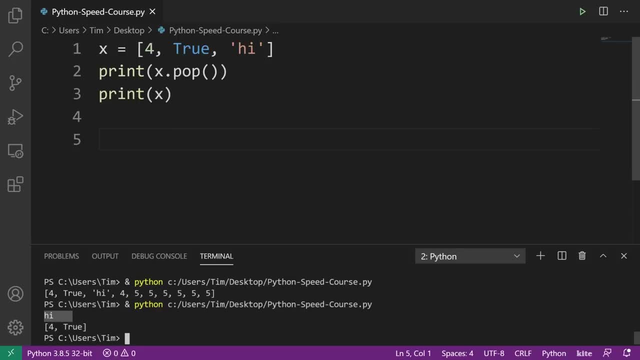 that When we print X again, so we get high and now our list has high removed because we popped it off of the end. Now another argument for pop is actually the index of what we want to remove When we look at a list. 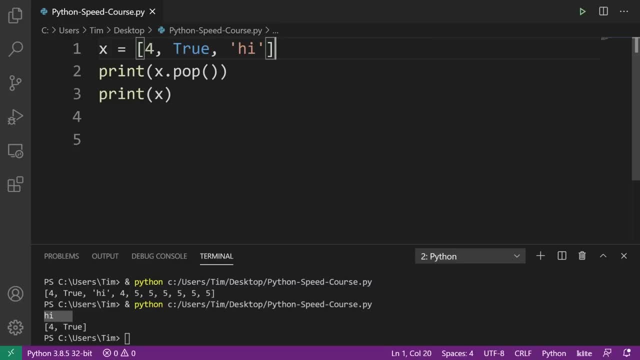 every single element in the list is identified by a number. That number is known as its index, otherwise known as its position in the list. When we start looking at indexes in a list, we start counting at zero. So the first position in the list is: 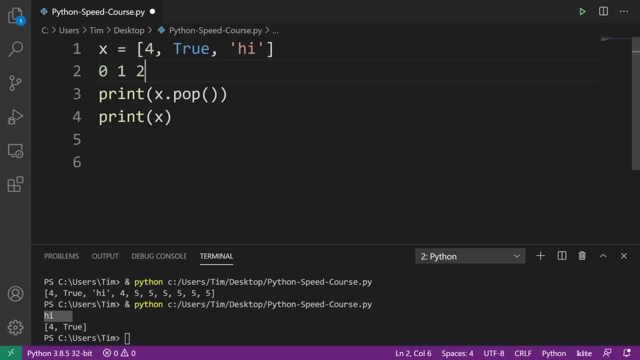 zero, The next is one And the last is two. If we want to know the last index X in a list, we look at the length of the list and subtract one. In this case we have three elements: The last index. 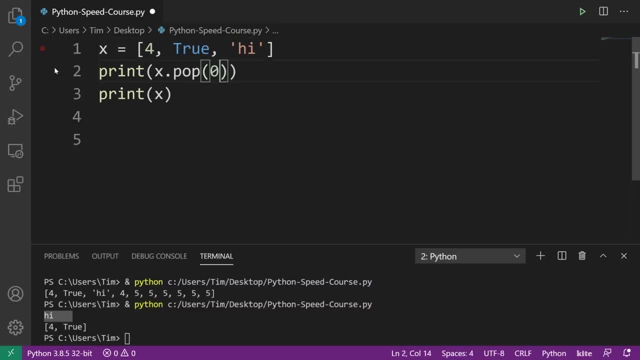 would be two. The first is zero. So if I go ahead and say X dot pop zero, what that's going to do is remove the first element from the list, which is four. So now we remove that And all of a sudden, if we look at 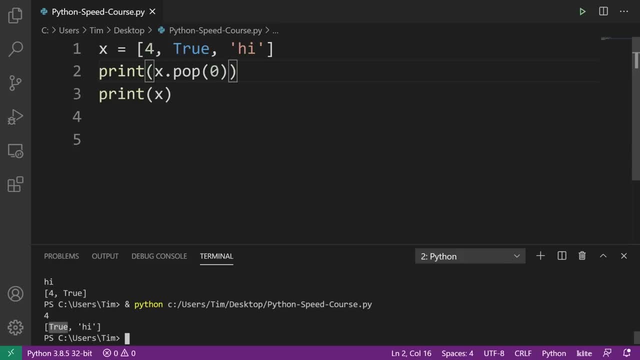 this new list, the first element at position zero, index zero, is going to be true. Now, if we simply want to access elements of the list- maybe don't want to remove them, We just want to look at them, We can say X put these: 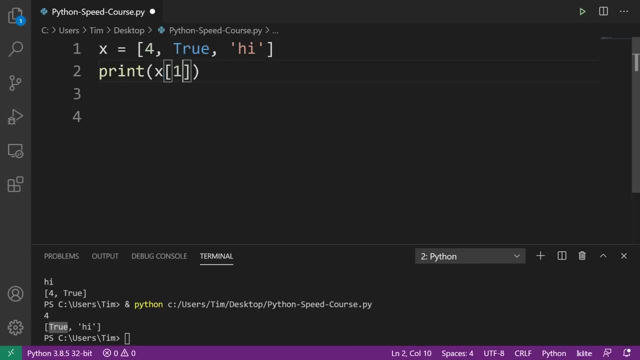 square brackets, which means we're going to access something and we can put the index of the element that we want to access. In this case, we'll access true. There we go, We print true, And that is the basics. Now what I can also do. 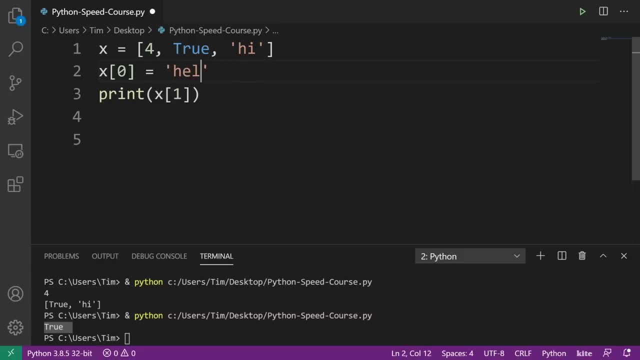 is say: let's do something like X, zero equals, and change its value to say hello. Now, when I print X, we'll get hello, true, Hi, let's have a look, And there we go. The reason I can do this is because 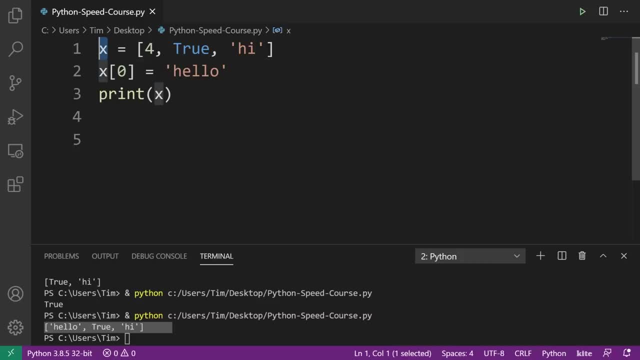 lists are what's known as mutable. This means this X right here does not actually store a copy to the list. It stores what's known as a reference to the list and the actual items itself are stored somewhere else. So for people that are more 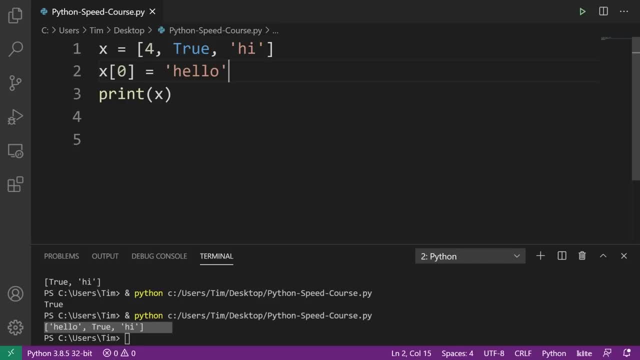 advanced and understand that. I'm hoping if you guys have come from another programming language, that makes sense. but lists are mutable, which means they can be changed. I can change all of these elements And if I do something like Y equals X, I go ahead and I make. 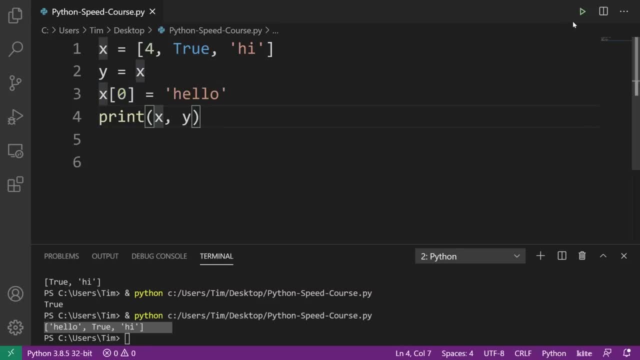 that change to X, but I don't make it to Y. you're going to notice that X and Y will be the exact same. So I have- hello, true, Hi, hello, true, Hi, making a modification to X, made a modification to Y. 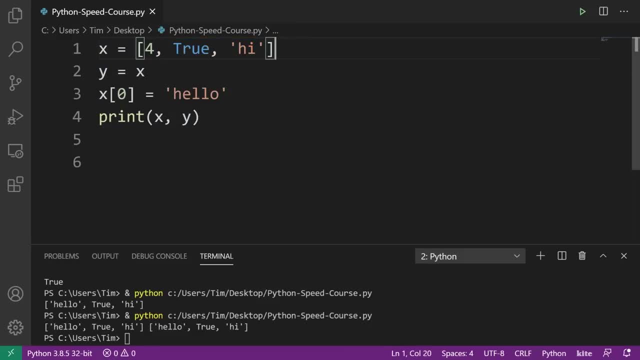 because X and Y are storing a reference to this list, not a copy of this list. If I wanted to copy the list, I would have to do this. I would have to do two square brackets, a colon inside. We'll talk about how this works. 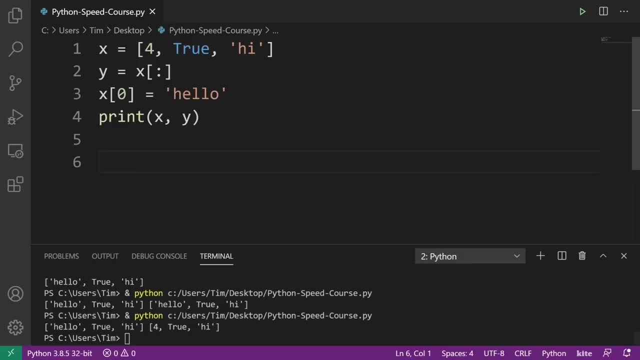 later, but now notice, if I made this copy, that change does not apply to the other list. There's a lot of other stuff that you can do with lists, but those are the basics And hopefully that makes sense. Next I'm going to talk about 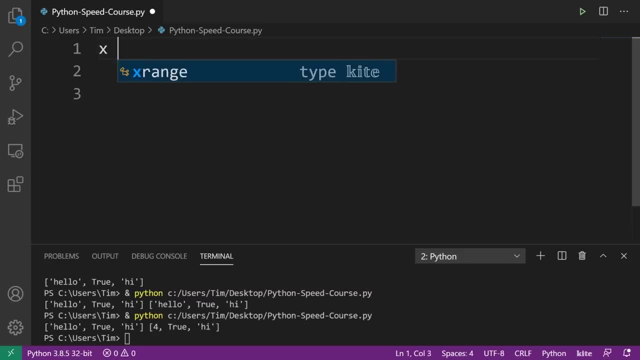 tuples. So tuples are similar to lists, except they are immutable. So a tuple uses round brackets instead of square brackets and it works pretty much the exact same, except we cannot append, we cannot remove and we cannot change elements. So a 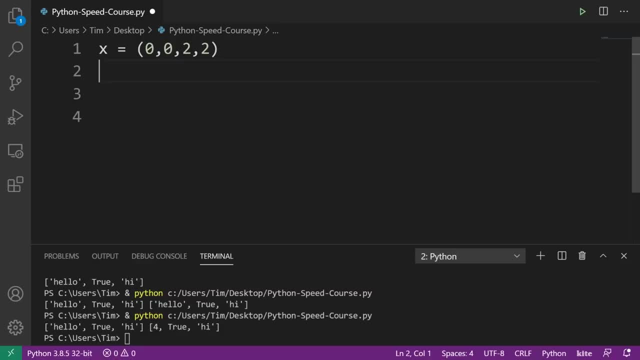 tuple is really an immutable list. You can think of it like that. It means it cannot be changed Once it has been defined. we want to change it. We actually have to redefine it. So what I can do is I can print out, say X, zero and 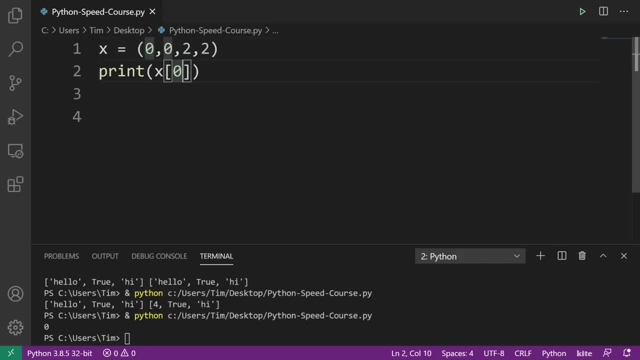 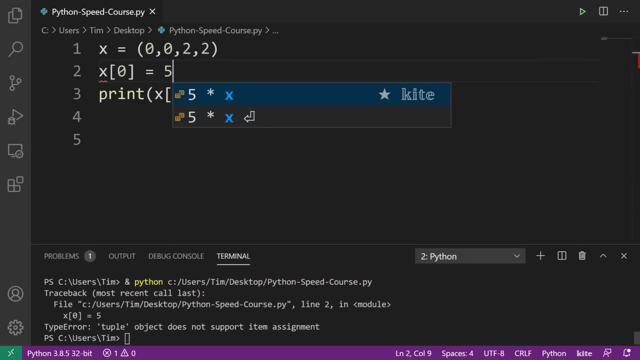 that's fine, That will give me the correct answer. So that'll give me zero. But if I go ahead and do something like X zero equals five and I try to do that, you're going to notice we get an error because the tuple object does. 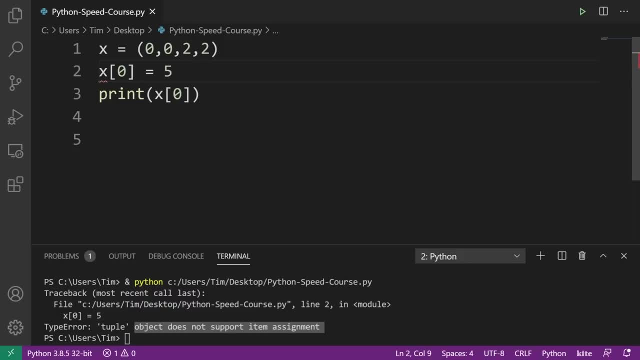 not support item assignment. reason for that Is because, again, it is immutable. I also cannot do something like X dot append. I can try, but you're going to notice that again we'll get another error. Tuple object has no attribute append. So this is a. 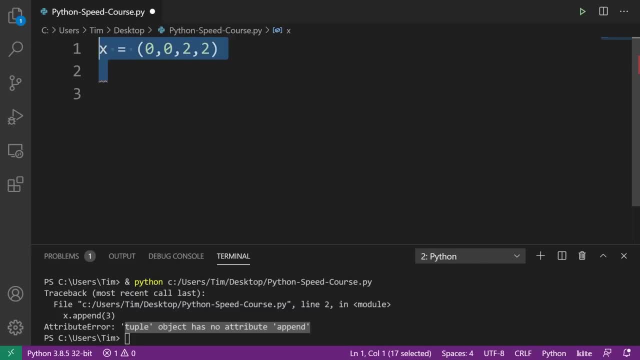 tuple, Um, they're not used a ton, although they are used sometimes. And just to note here, you can have lists inside of lists, So I can say something: like you know, I can have a tuple inside of a list, I could have a. 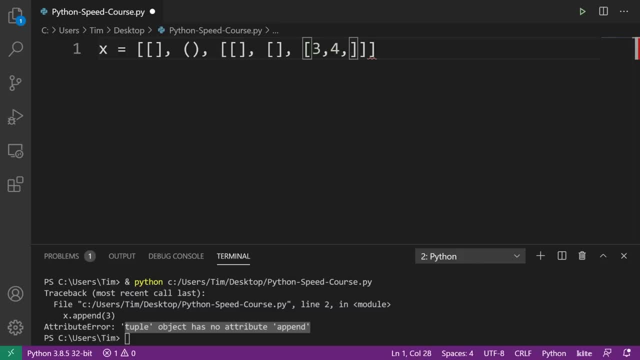 list inside of a list inside of a list, and I could have elements inside of this. They don't need to be uniform size, Um, sometimes in other programming languages, when you're looking at a raise, if you have embedded lists every. 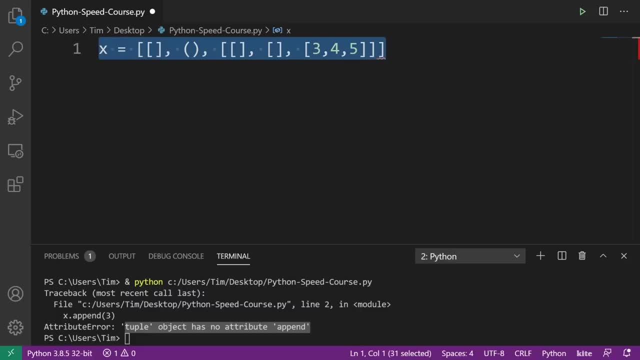 element has to be another list stuff like that. Just wanted to point out that you can do something like that. Uh, and I think that's all I'm going to cover right now for list and tuples. All right, The next topic I have for. 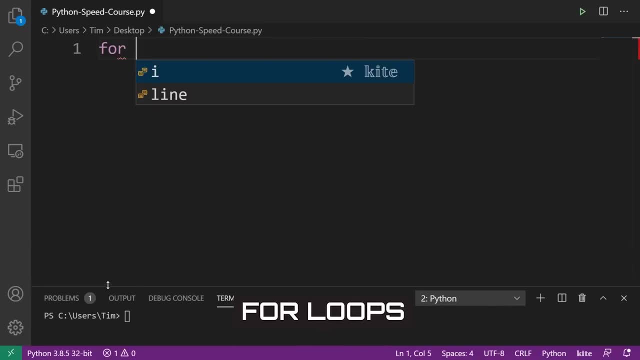 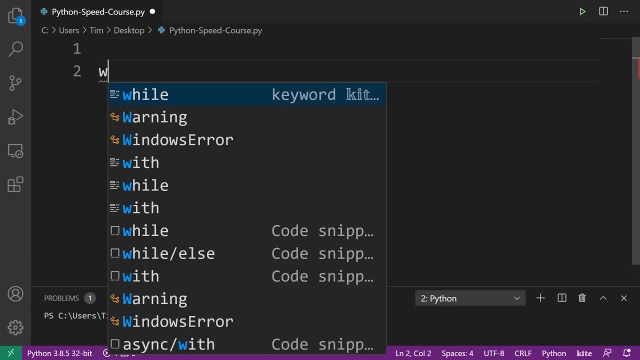 you is for loops, Now for loop. if you've learned in other programming languages, allow us, allows us to iterate a set number of times, So we will be talking about a while loop. The main difference between a while loop and a for loop is: a while loop is 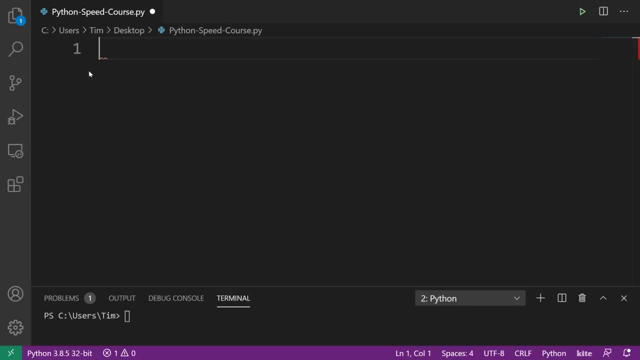 running and in defined amount of times. we don't know. we're going based off of a condition which we'll see shortly. Okay, For loop. We know how many times we're going to loop, at least relatively. So what I'm going to do is I'm 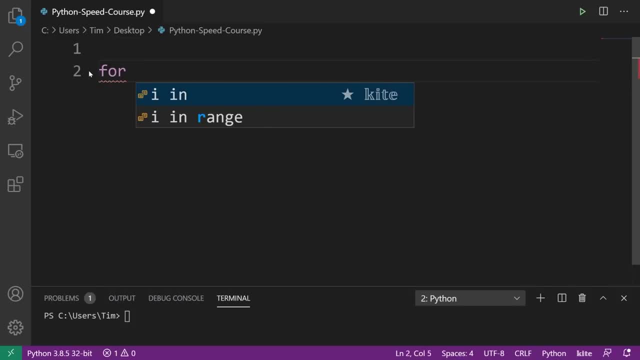 actually going to show you how we can just create a basic for loop to print the numbers that from one to 10, say for I, in range, And then inside of here we simply put 10.. I'll talk about what this range function does in a 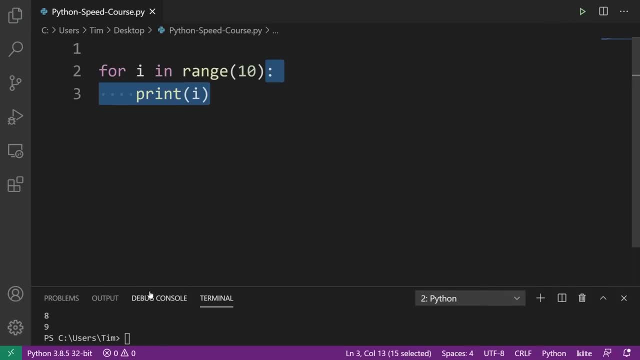 second, but let me just show you how the for loop actually operates. So now I can show you that this Prince- 0, 1,, 2,, 3,, 4,, 5,, 6,, 7,, 8,, 9- does not include 10.. 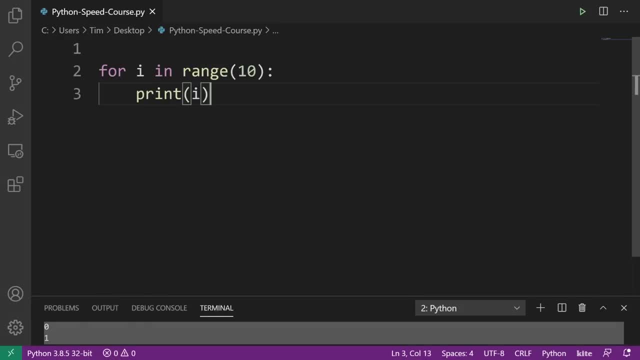 So the way we set up a basic for loop, if we're just going to be iterating through account, is we say for I or for some variable, this is going to be our iterator, or a counter variable, whatever you'd like to call it. 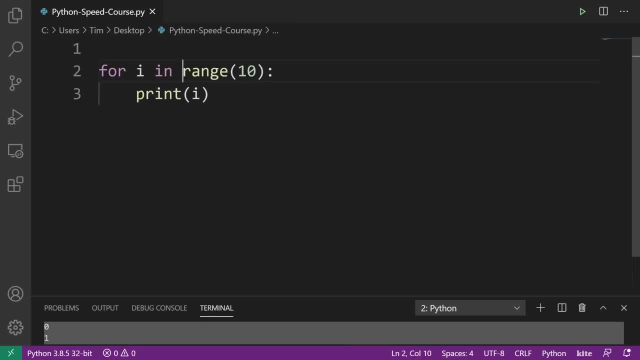 in. This is a keyword we always have for I in and then some word. here. in this case, we're going to put range. range is a function that actually creates a collection of numbers based on the input that we give it. The input to range is: 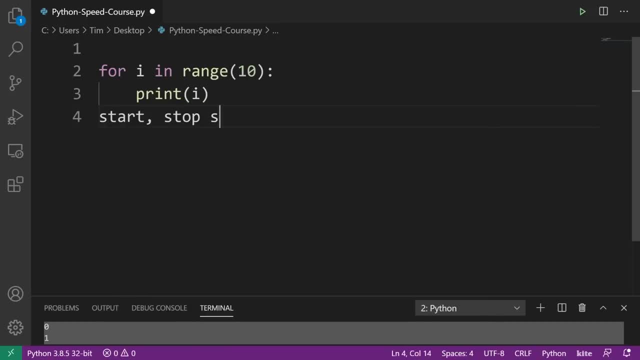 the following: start, stop step. So we're allowed to put up to three um and we can have less than three arguments inside of this range function. essentially, start stop step is saying okay, what number do we want to start at? 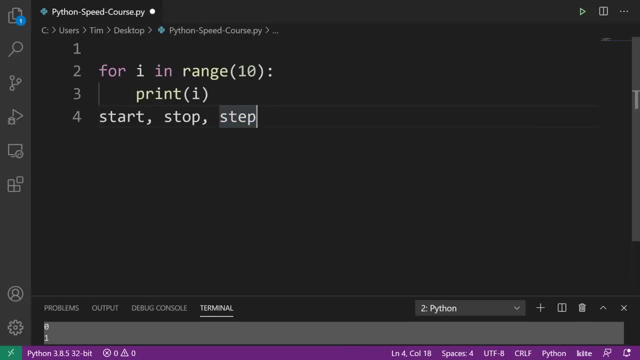 What number do we stop at? What number do we step at Now if we only have one argument? so we only pass one number by default. that is the stop argument. Uh, we usually start at zero, So by default our. 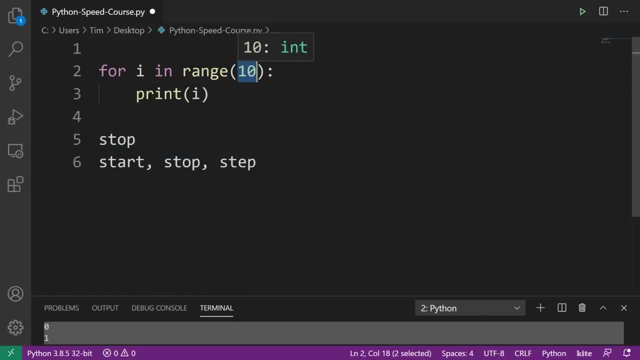 range will start at zero and we will go to whatever number we put here. Most of the times, you're just going to put one number and this defines the ending range. So in this case it says: okay, we're going to start at zero. 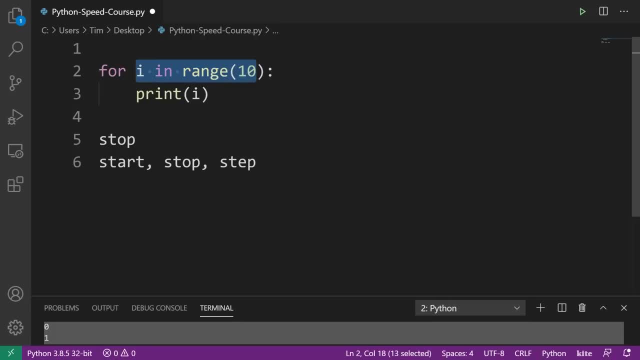 and we're going to go up to 10, but not include 10. notice, We didn't print 10.. Now, if we had two arguments, that's going to be default Start stop. So I will say, okay, we will. 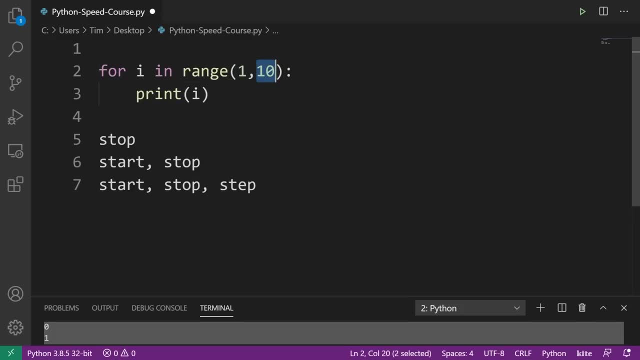 start here at one and we will stop at 10, but not include 10.. If we had three, we'll include a step, And that tells us how much we should increment every single time. by default, we increment by one, but we can. 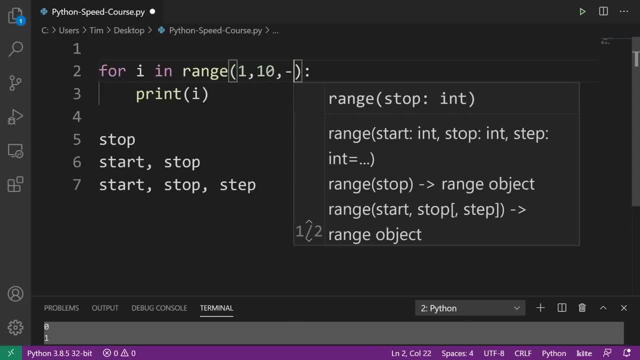 increment by two and we can increment by a negative number as well. Let's actually say that we wanted to start at 10 and we wanted to go to negative one And we wanted to step by negative one. Well, let's have a look at. 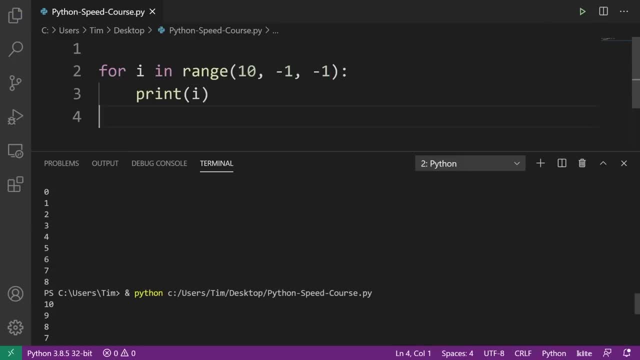 what this looks like and just test it out. Okay, So running, you can see we started at 10. Right there, And then we went all the way down to zero And, of course, we can start at negative 10 and watch. 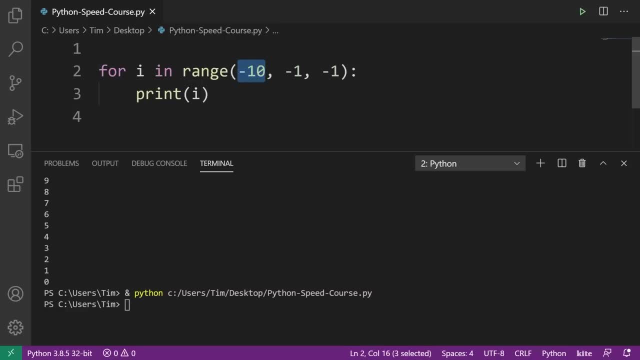 what will happen here? We do nothing. The reason for that is we started at negative 10.. We were going to negative one and we're stepping by negative one, but since we were already past negative one, we aren't going to go there, obviously. Uh. 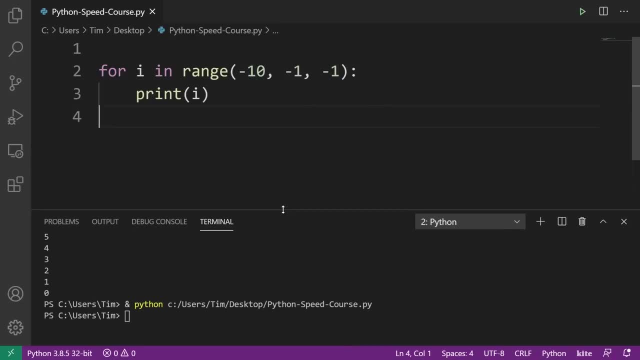 and we just immediately stopped. So that is kind of how the range function works. So for I in range again: start, stop, step by default. If you just put one argument, that's going to be the stop. If you put two, that's start. 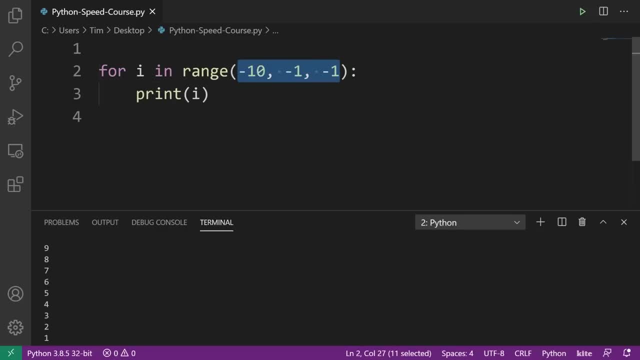 stop. You can mess around with that and see how it works, But I think that's enough of an explanation. The next thing we can do is actually loop through a list. So let's say we have four I in, and now, instead of range, we'll. 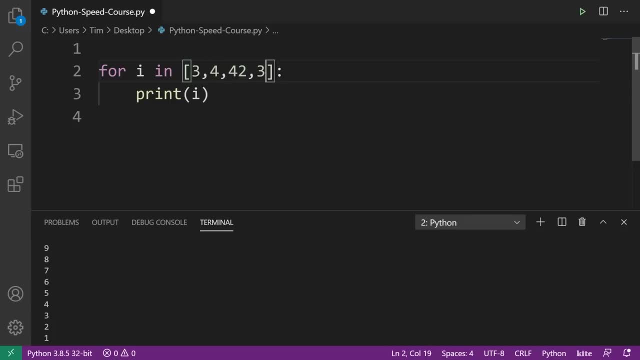 simply just put a list, We'll say for I in range, and we can do three, four and just a bunch of numbers here. Now if we print I, it will simply print all of the numbers in that collection or in that. 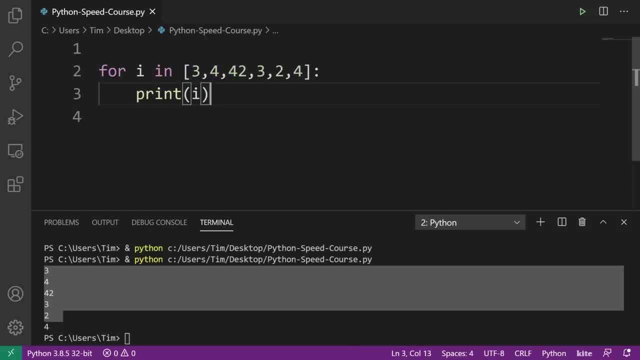 list. it will step through one at a time and print all of them. Now let's say that maybe we didn't want to do that. Maybe we actually wanted to keep track of what index we were at. We could say X equals the list We'd say for 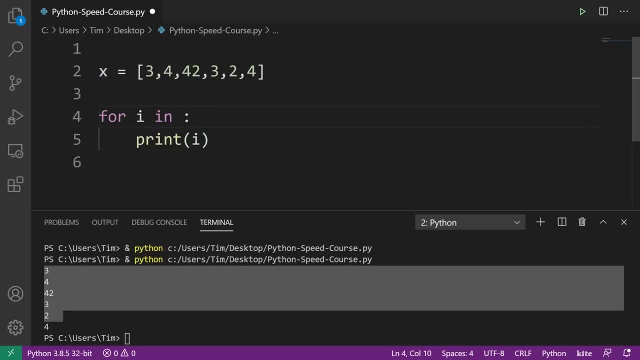 I in X, and then- um well, sorry, that actually would not be the right way to do it- We can say, for I in range the Len of X, and then instead of just printing I, we could print X square brackets. 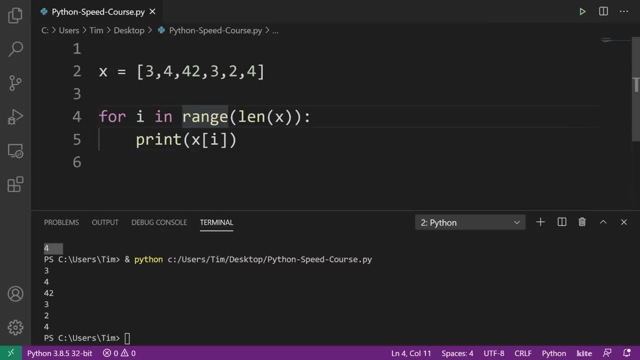 I let's have a look at this here. You see how that works. The way this works is we're going to go up to, but not including the last index of X or the length of X, Sorry. So in this case, 1,, 2,, 3,, 4,, 5,, 6.. So 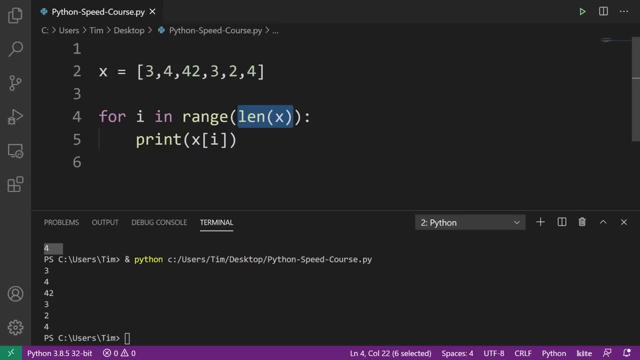 this right here. we'll say six. So for I in range six, that means the maximum value of I is going to be five. So we say uh, X, zero, X one, X, two, three, four, five and print all of the values out. 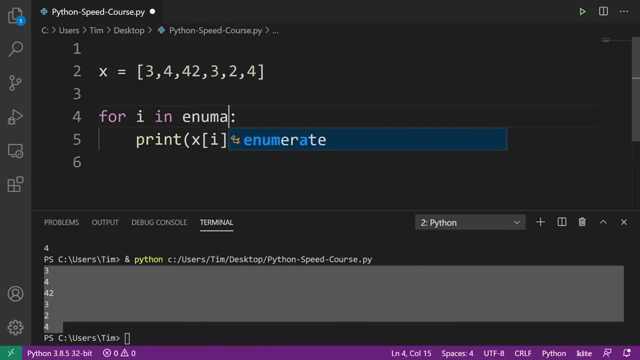 Now there is another fancy thing that we can do if we want to avoid using that. it's called enumerate. What enumerate will do is create indexes and values for all of the elements in our list, We'd say for I, comma, element in enumerate X. 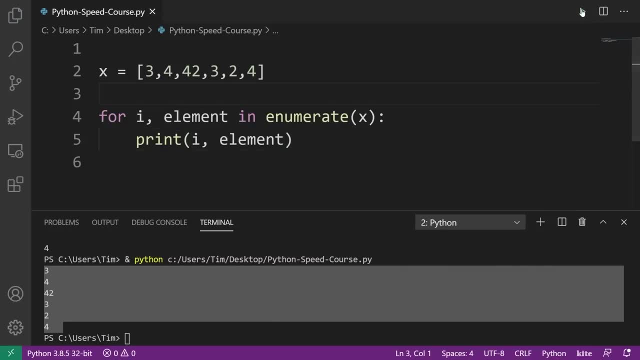 And then what I can do is I comma element and you'll see how this works. What we do is you get zero, one, two, three, four, five and then all of the elements. So this works kind of like a combination of the two. 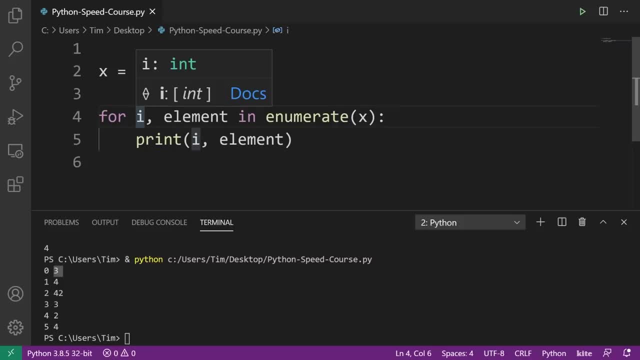 four loop styles. I just showed you what. we actually have a range, So we go from zero up to five. Those are all the indexes in the list, And then we print all of the elements for each of those indexes in the list And we just have. 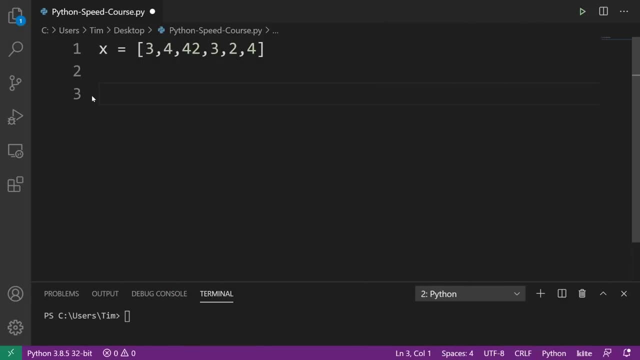 two variables here that denote that. So the next topic to discuss is a while loops. Now, while loops are pretty straightforward. essentially what they are is: while condition equals equals, true, go ahead and do something, So we're going to have some condition here. uh, 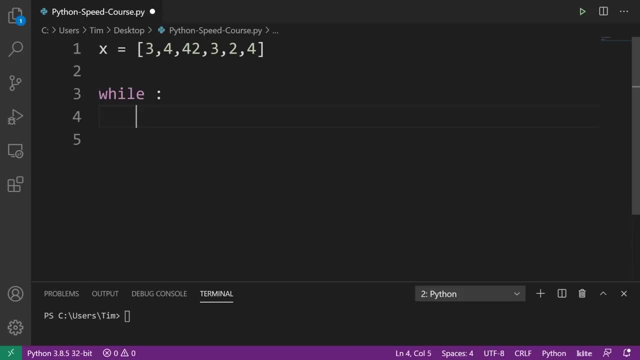 before this colon And then after the colon, there's going to be an indented block and whatever's in that indented block will run inside of the loop while that condition is true. To illustrate this, I will say: I equals zero. So while I is less than, 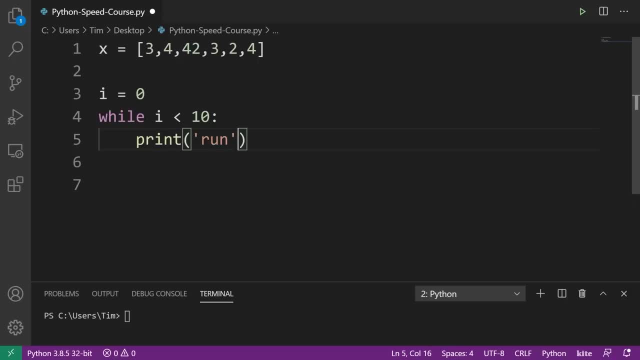 10, we'll say print run And then we will say I plus equals one. This is another way that you can add one to a variable. So you could say I equals I plus one. or you can do I plus equals one. You can also do: 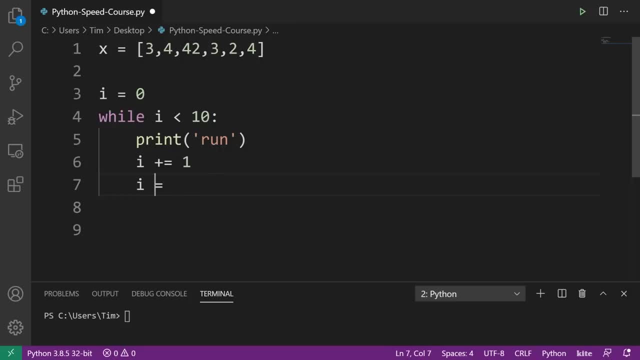 something like I multiplied equal by one, or divided equal by one, So multiplied by equal to. what that's going to do is say: okay, multiply I by two. We could do something like that if we want it as well. Just showing you some. 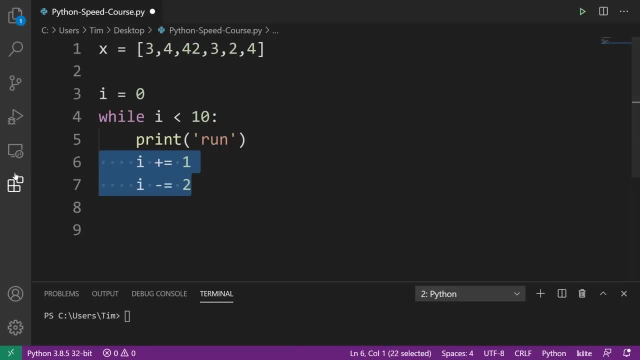 more syntax for some interesting things that we can do in Python, but as the basics of a while loop. if I go ahead and run this, we can see that this is going to run 10 times And there isn't really much more to talk. 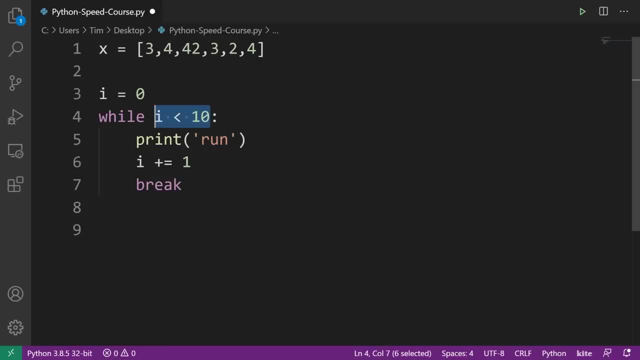 about for the wallet other than the fact that we can implement a break statement. So we could also write the same code like this: while true, I plus equals one, And then if I equals equals 10, break, and that will simply break out of. 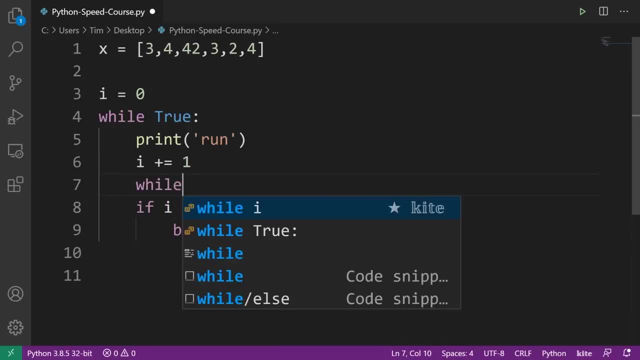 whatever the closest loop is to us. Imagine we had another while loop like this And we said: while true, inside of here, then this would break this while loop, not the other while loop. Hopefully that's making sense. Anyways, let's move on to the. 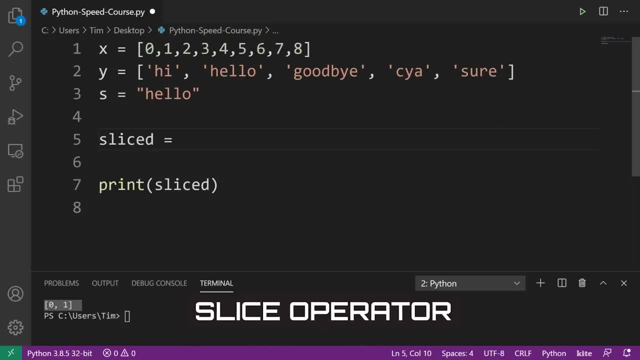 slice operator. So the slice operator is personally my favorite part of Python. There is implementations in other languages, but none of them are as nice as Python in my opinion, And what this allows us to do, essentially, is to take a slice of a. 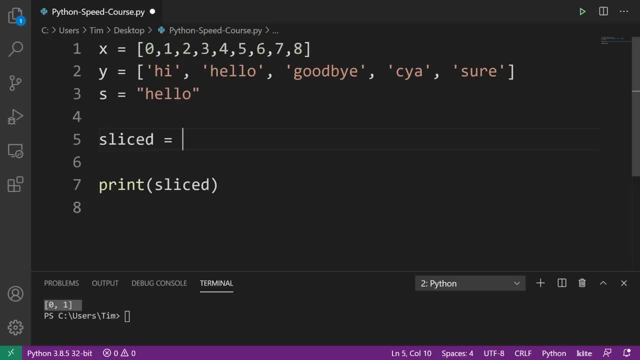 collection like a string or a list or a tuple, and do something with it. So let me just show you what I mean. The slice operator is simply the square brackets like this, with a sequence of colons and numbers within it. The way that it works is we: 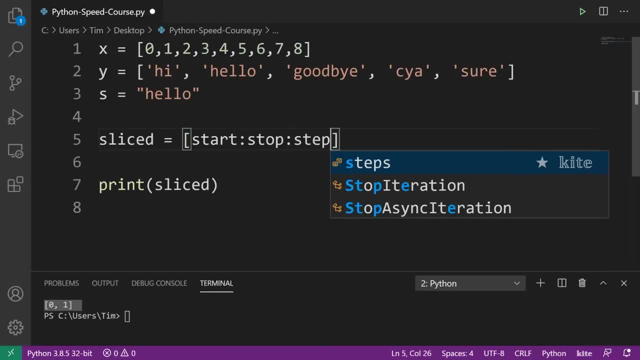 have a start, a stop and a step, just like the range function that we looked at before. So if I put something like X here and then I go start, stop, step, what I can do is say, okay, I. 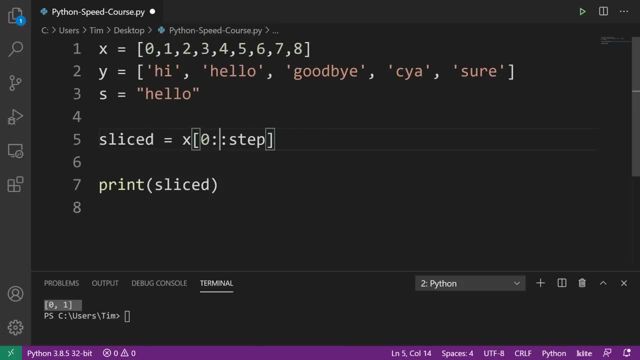 want to start at zero. I want to stop at index- These are all indexes that we're putting into here- three, and I want to step by two. Now, actually, let me just stop at index four, just so we get some more. 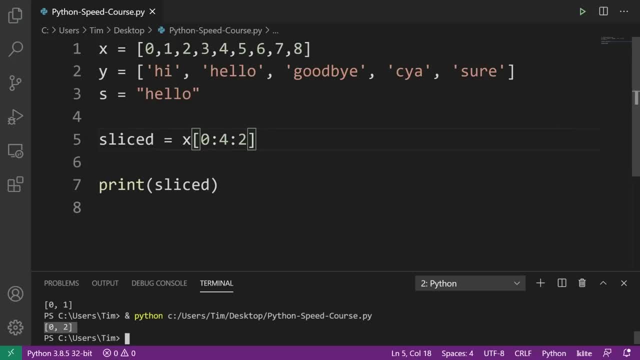 values in here. Let me show you what this looks like. We get the value zero to what I have, zero for two in my slice. What this is saying again is: start at the first index, which is zero. uh, go to the fourth index, but do not. 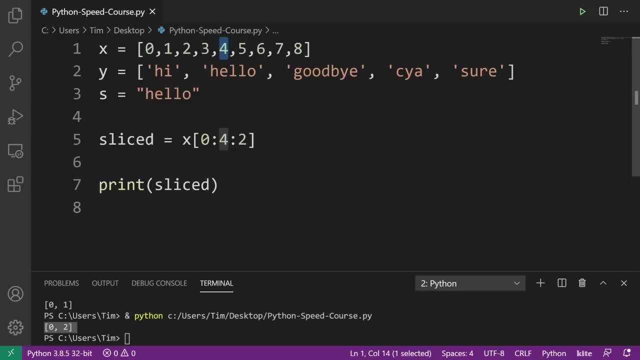 include it, which means stop as soon as we hit this and step by two. So we're going to start at zero, Then we're going to go to two, and then we're going to go to four, But since four is the stop, here we're. 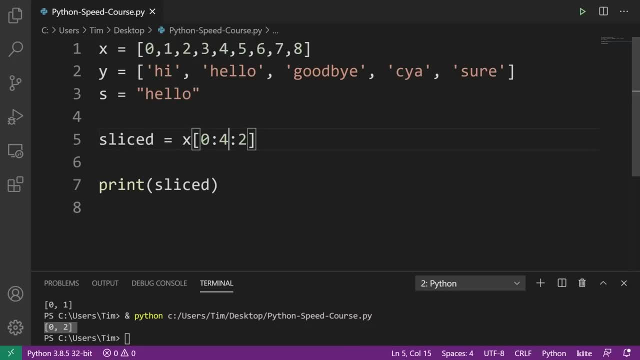 not going to include that in our slice Now when we do the slice operator, we don't have to include all of these different things as arguments. In fact, what we can do is just include a stop, just include a stop, and. 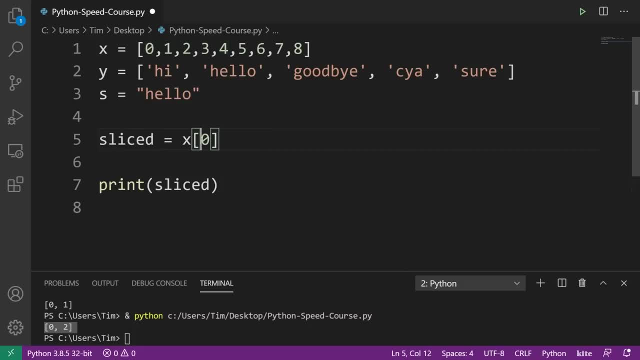 include a start and all of that, So just like the range function. if we don't include anything, so we just sorry. we just include a colon like that, And then we put something on the right hand side that is saying stop at. 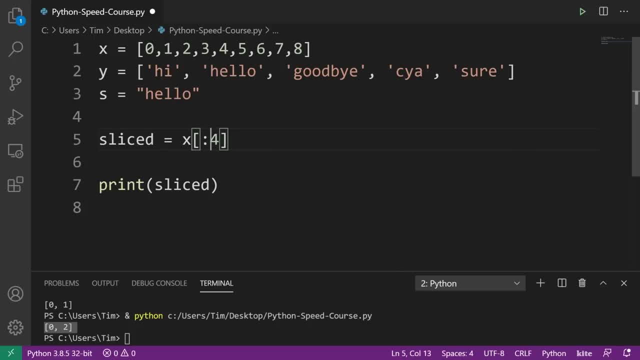 whatever index we put here. So if we do this, it says start at the beginning and stop at the end. Now, if we do something like two colon, that says start at two and stop at the end. So whenever we leave a blank, we're assuming 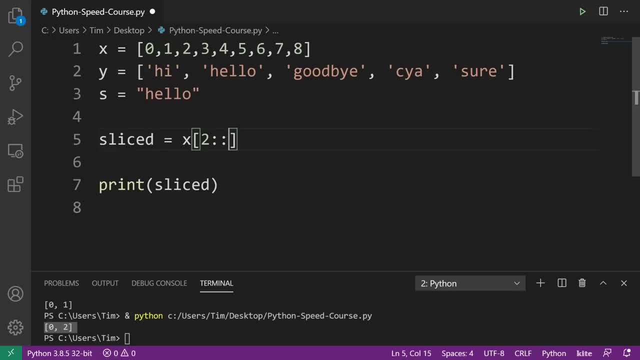 it's either the end or the beginning, or one in the case of a step. So if I did two colon colon, maybe I did two colon, four colon. This is saying, okay, start at two, stop at four and then step by. 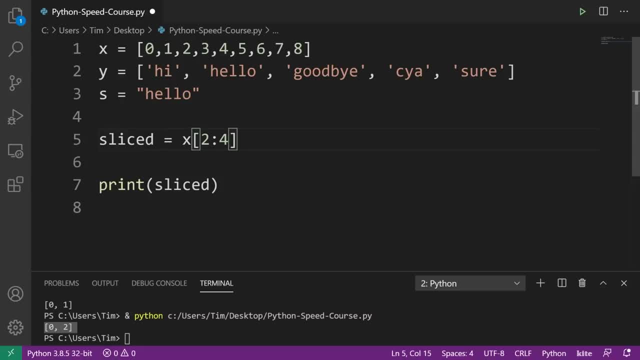 one, but I don't even need to include that. I could just do two, colon four. but now let's say I wanted to go four and then colon two, colon negative one. What this is saying is: okay, start at four, go to two. 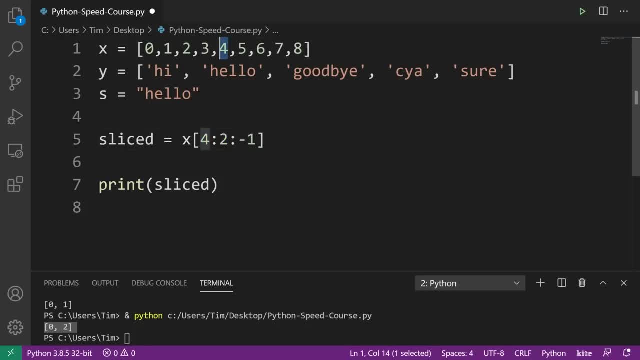 and step by negative one. So now, what this is going to do is start at four, which is actually this, and it's going to give us four, and then three, and then it's not going to include two or any of the other ones. 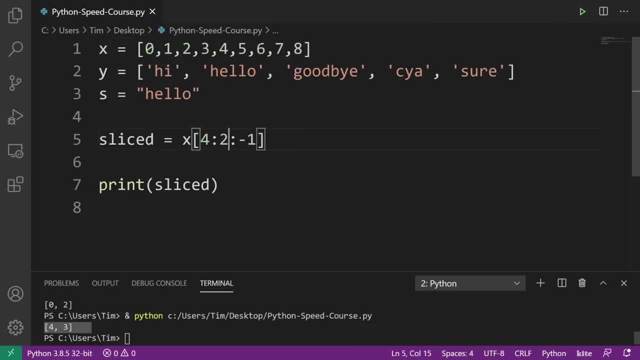 So that's what we'll get In fact. let's look at this. We see we get four, three. Now one of my favorite things with the slice operator is two. To reverse a list, all we have to do is colon. 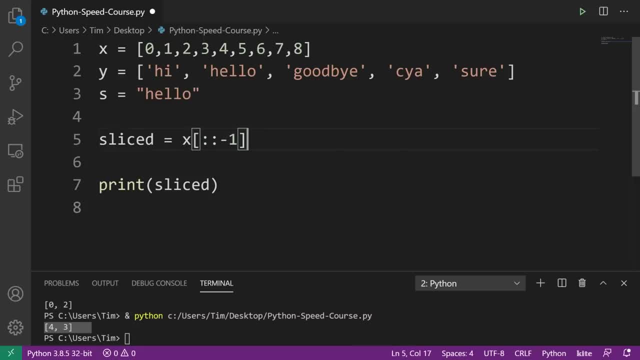 colon negative one. This means start at the beginning, stop at the end and then step by negative one. So this will actually start stepping backwards, which is kind of interesting. So when we look at that, we get eight, seven, six, five. 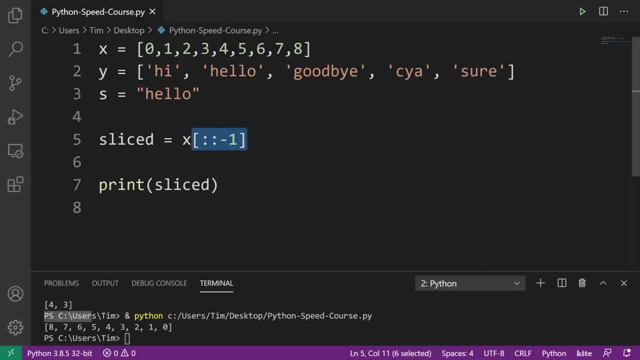 four, three, two, one zero. That is an easy way to reverse a list in Python. Now, of course, all of this works on a string as well. Let me show you that with S, you see, we can reverse the string like that And we. 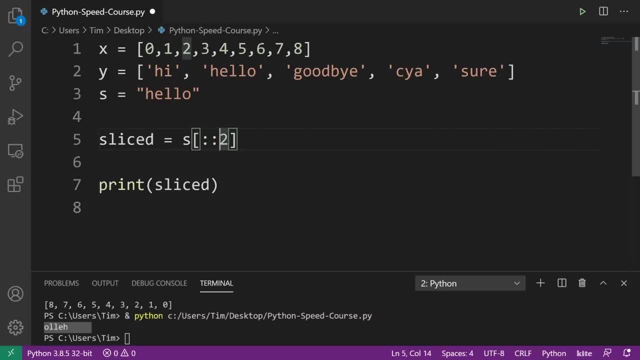 can also just do the standard arguments. So we would typically do let maybe we'll just step by two. So start at the beginning, stop at the end and step by two. We get H L? O. So that's the basics of the slice. 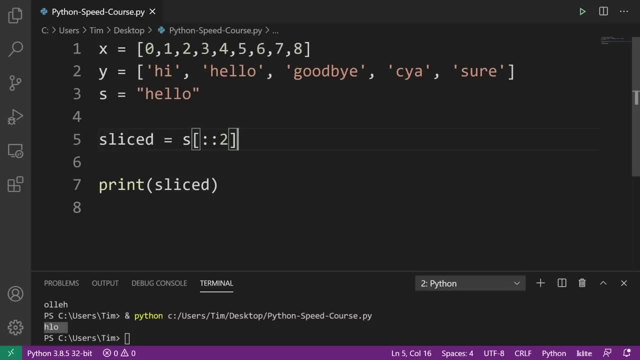 operator. There's a bit more stuff that we can do with this, but that is kind of how it works, And I believe this works on doubles as well. We can just try it out to make sure that I'm not lying to you guys. Uh. 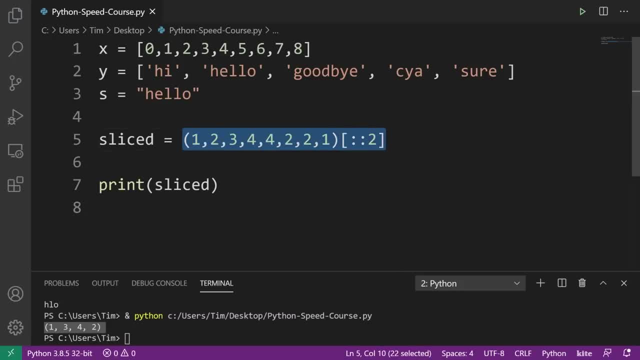 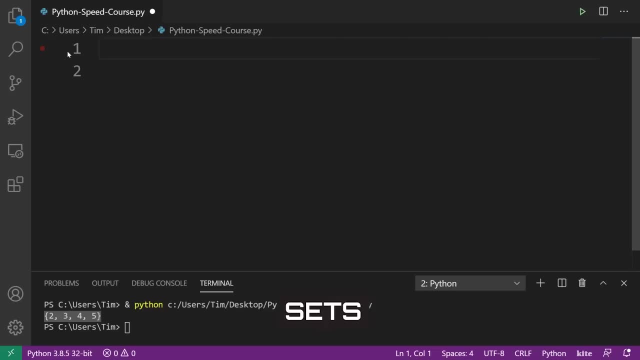 but if I do that, you can see that that does indeed work and we can use the slice on kind of any collection of elements. All right, So now we are moving on to sets, which are an underrated but extremely useful data type in 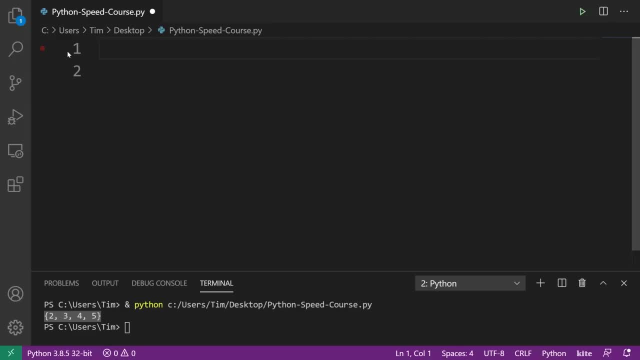 Python Now, a set is simply an unordered, unique collection of elements. What that means is there is no duplicate elements. We do not keep track of order or frequency of elements. All we care about is if something is there or if something is not. 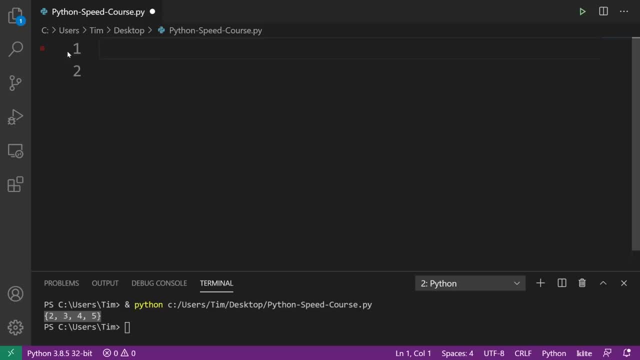 there. the reason we do this is because a set is extremely fast to do what's called lookups, removals or additions. When we're talking about a list, let's say we have something that's you know, has a bunch of elements in it. If we 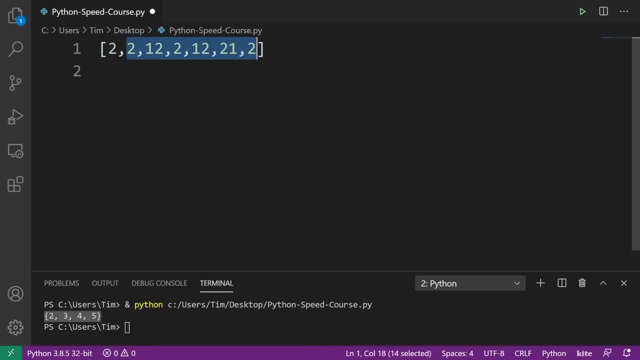 want to say remove the first element from the list. that actually involves shifting the position of all of the other elements, because we're keeping track of the positions of these elements with a set, since there is no notion of position adding and removing something. 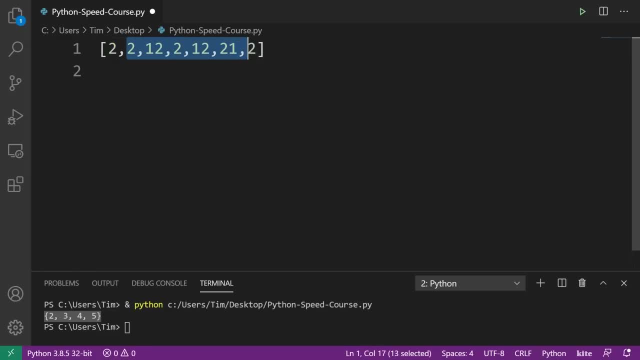 As a simple is just adding or removing that element. There's no other operations that need to be done, which means it's very fast to use. So think about a set to be used only in a situation where you care if something exists or doesn't. 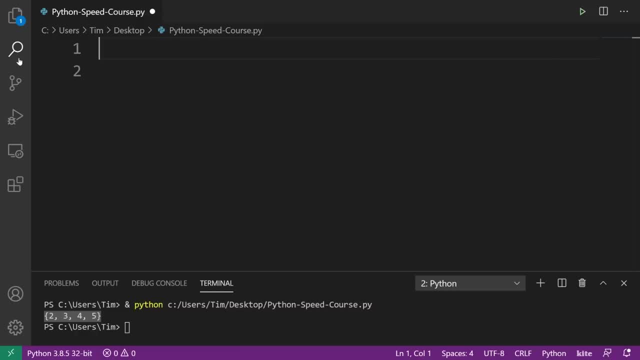 exist, not about the frequency or order in which that item exists. So to create a set is pretty straightforward. We can say X equals set and we use the open bracket and close bracket. Now the reason we don't actually write something like, say S. 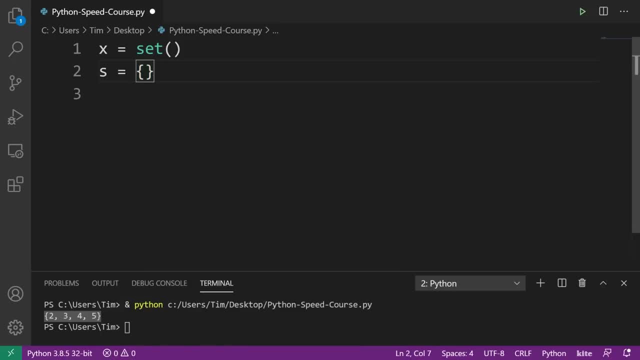 equals, and then this, which is really the representation for a set, is because what this will do is create a dictionary. Now, technically, if we want to create a set, we can do something like this, and this will create a set for us: that 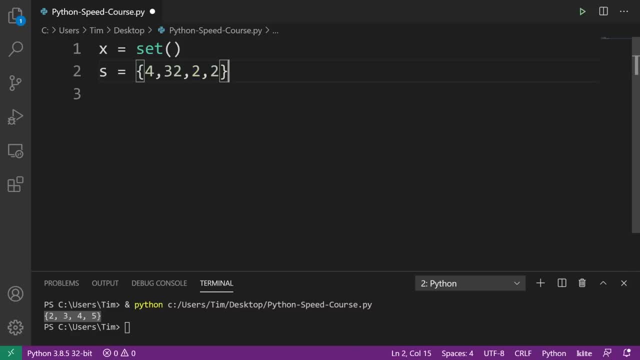 initially has the elements for 32 and two inside of it. This is what's known as a set literal. If you're not going to be creating an empty set, it's totally fine to do it like this, So long as you add an. 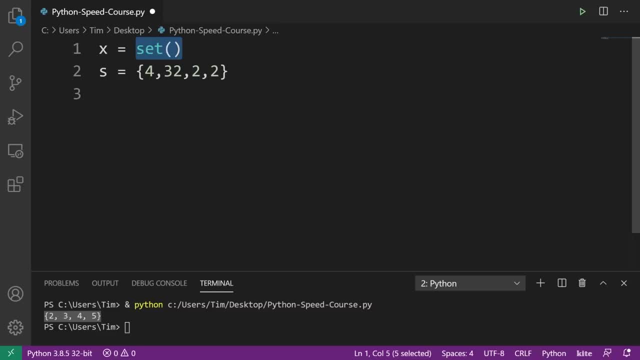 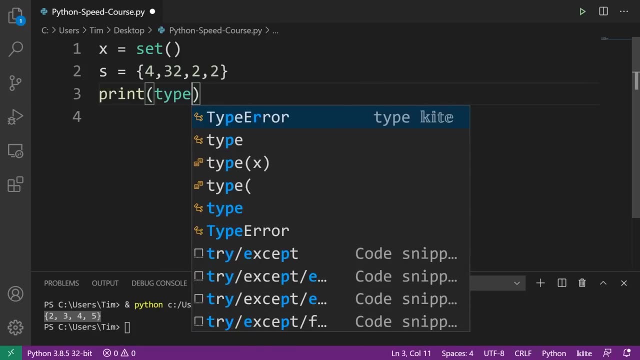 element inside, but if you are creating an empty set, then you need to use this constructor. Otherwise, you're going to end up creating a dictionary, which is not what you want. to prove the simple point to you, I will print out the type of just an empty 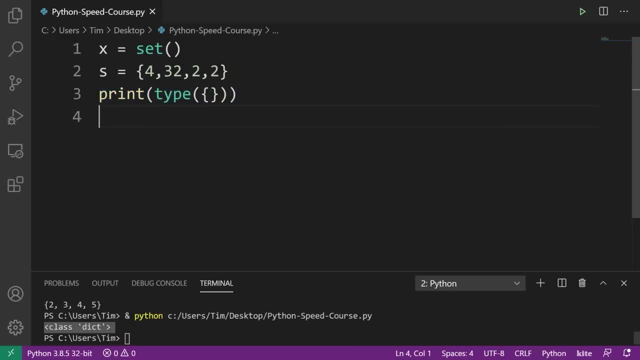 um, you know set representation and you'll see that it gives me dict Right Like that. Of course, that's not what we want. Anyways, let's have a look at this set and I'll just show you what I mean by unique. 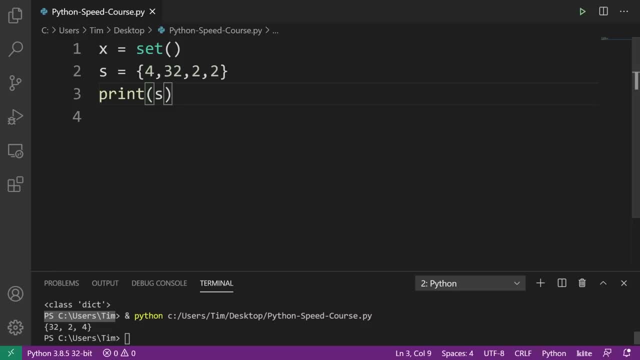 unordered collection of elements, So for 32 to two. if we print that out we get 32 to four. So obviously a different order than how we added in there and notice that the duplicate twos were removed. Now the set operations are pretty. 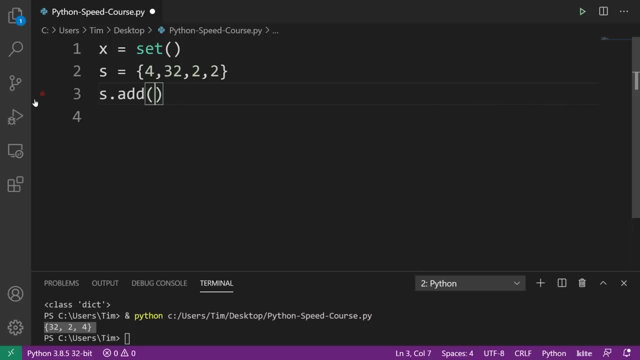 straightforward. We can add something to a set with S dot. add our set dot. add. I'll put five inside of here and let's just keep printing out S. there we go. We can see we added in there. We can also do S dot remove. 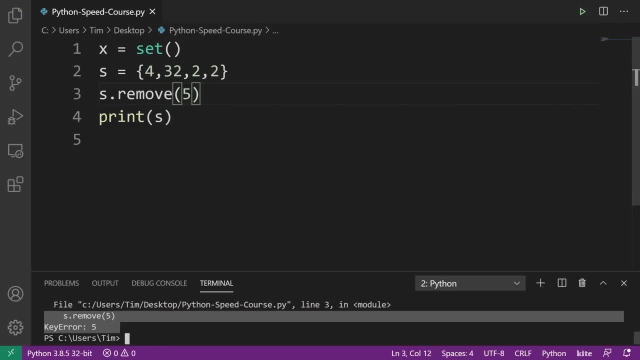 five, and that will well, since there's nothing in there- give us a key error. Now, if there is the element in there, so we can do it like this, it will remove that element for us, And then there's a. 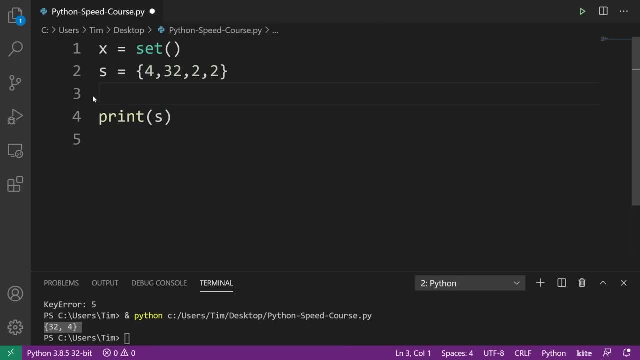 few other things that we can do as well for a set. One of the good ones is actually checking If something is in a set. what I can do is say for in S. what this will do is simply check if the element four is in the set, and 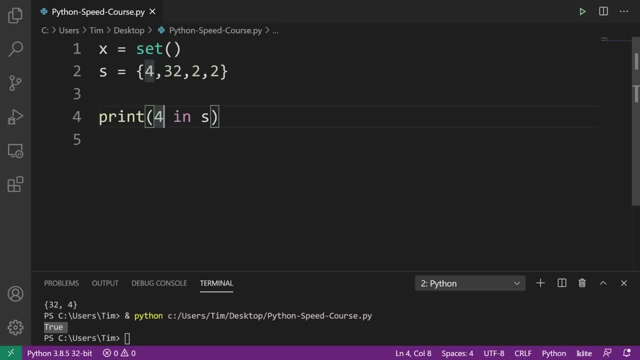 give me a true or false. in this case it is true, And remember this happens in what's known as constant time, which means it's just extremely fast to do this as opposed to a list, So we can say three, four, five and. 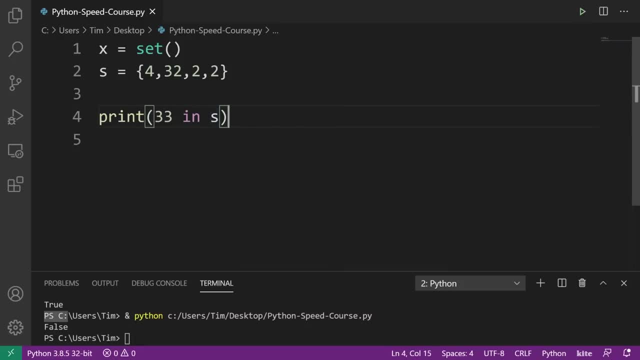 33 and S, that's going to give me false. Now the parallel I want to make here is if I had S equals two, four, 32, two, two, like that, So actually let's go S two. And then I said print: 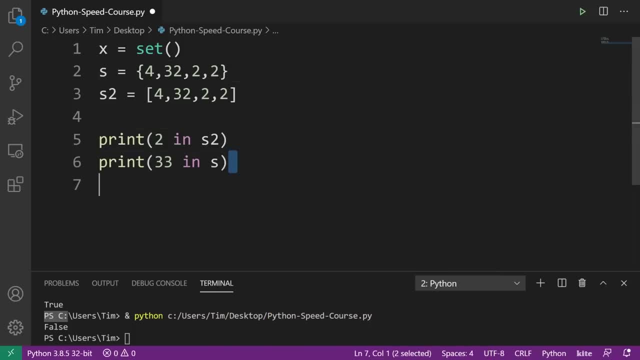 and let's just go to an S two. this operation, the one that's actually in the set, is going to happen much, much, much, much, much faster than this one. Of course, this isn't a big deal right now, because these: 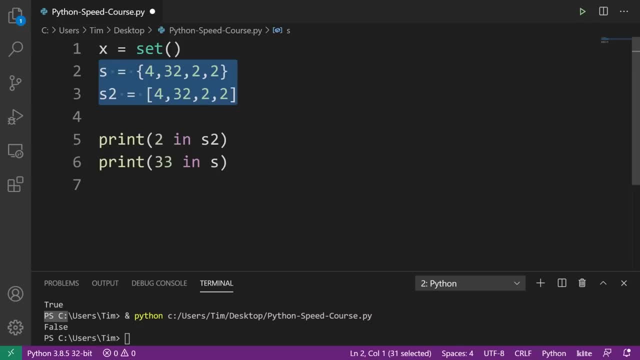 collections are quite small, but as these get extremely large, just understand that using a set is very beneficial when it comes to looking things up, checking if something's in there, removing and deleting. there's a few other operations we can do on sets. Let me just 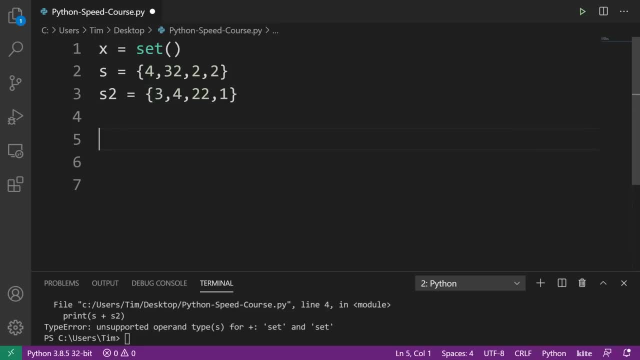 define S two And I'll just quickly show you a few of them. Uh, we can do, for example, the intersection or the union of these sets. So I can say S dot, union S two, and we'll go ahead and have a look here. 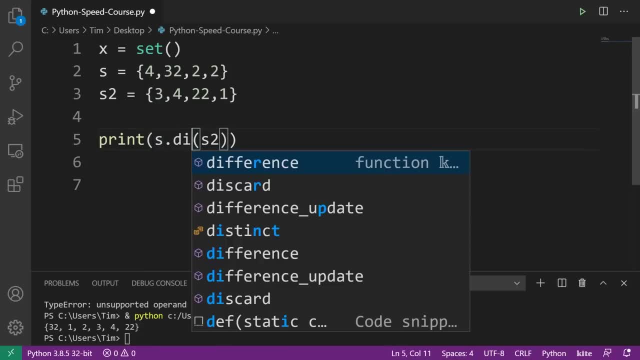 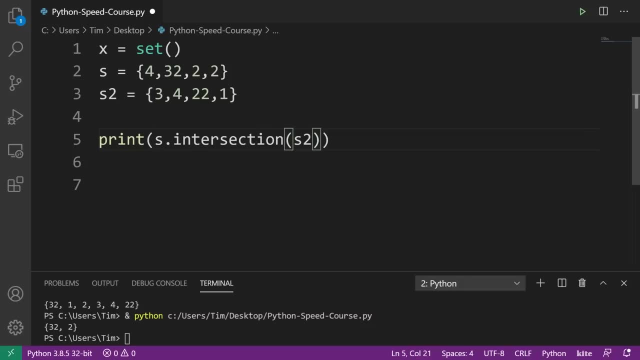 And we can see we get the union of these two sets, essentially adding them together. We can do the difference of the two sets If we want, we can do the intersection and we can do the symmetric difference and all that other fun stuff that you can do. 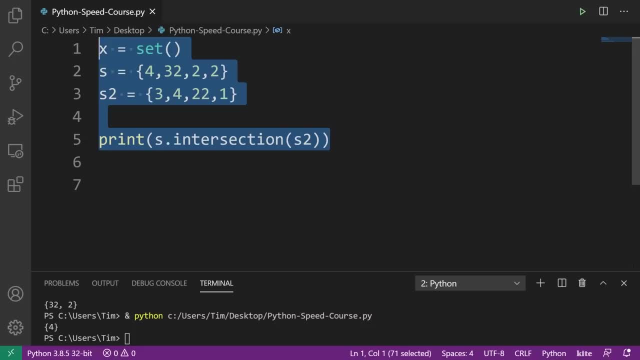 with sets. Now, I'm not going to get into all of that stuff, Just know that these are sets and that's some of the stuff that you can do with them. So now I'm going to talk about dictionaries. Now, if you're from another, 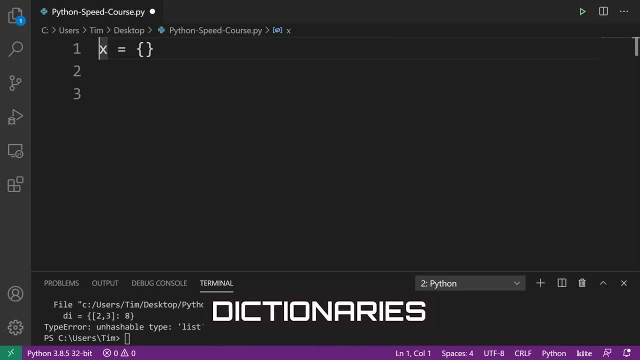 language. what may be familiar to you here is a hash table or a map, something like that. They're very similar to dictionaries, but a dictionary is essentially a key value pair. You have some key, you have a colon and then you have some. 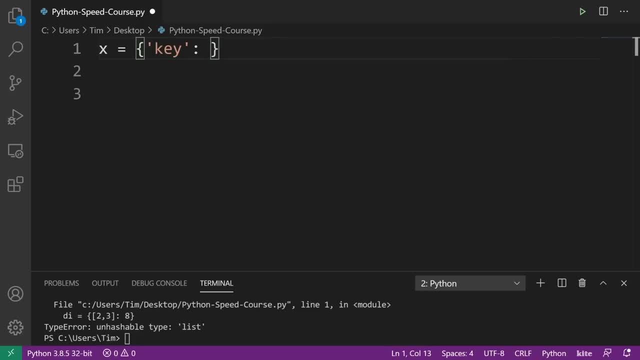 value that it corresponds to. Now, of course, that value has to actually be a valid data type, but it could be something like a list. It could be a single value like that, And the way that you access and create new key value pairs is. 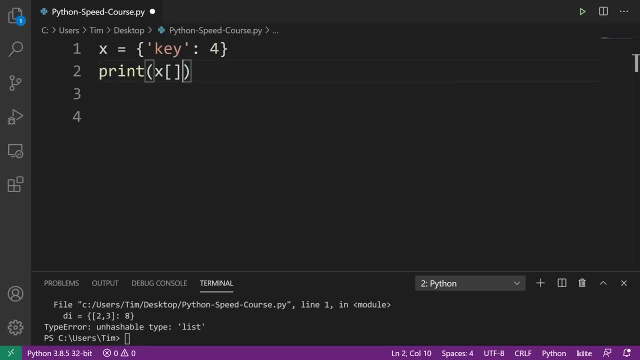 something like this: I can print out, say X, and then the key inside of here. in this case it's actually called key, And what that will give me, if you look down here, is simply the value for, because, well, that's. 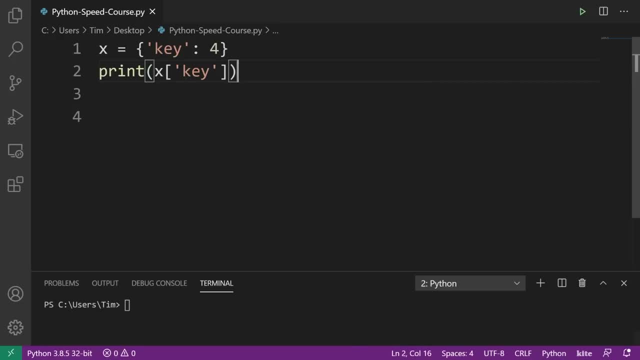 what corresponds to this key. So you have keys and you have values. Now to add a new key is pretty straightforward. What you can do is you can say X inside of square brackets. you can define whatever key you like. It can already exist If you. 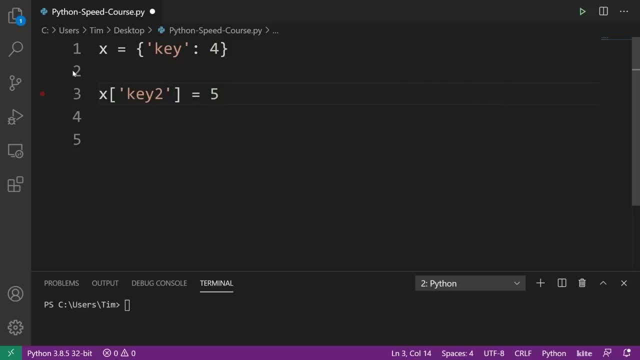 want. we can say something like key two and we can make that equal to five. Now, now note that these keys do not need to be the same- uh, I'm sorry. same data type, So I don't have to have two. 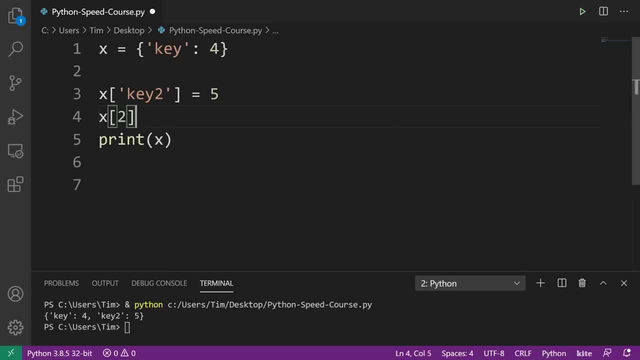 string keys. I can have integer keys and have whatever keys I want to do, something like X: two equals eight, And there we go. You see, that works perfectly fine. In fact, I can make this a list just to prove to you that the values don't have. 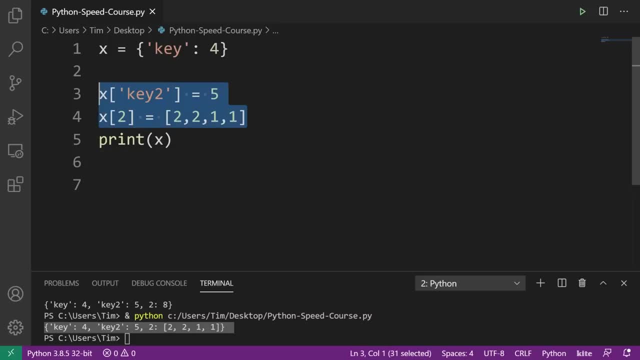 to be the same either. And there you go Now, just like a set. this actually works using a hash, which means this is very fast to retrieve, add and modify values within the dictionary. In fact, it's so fast. 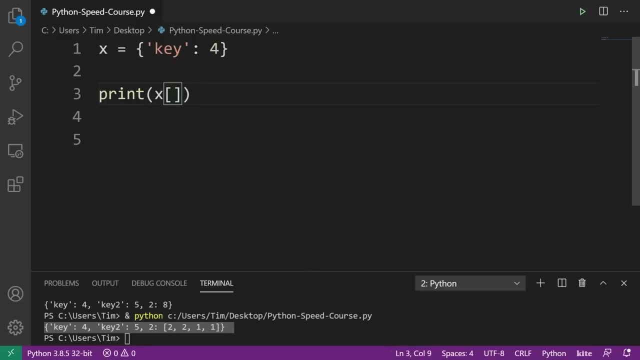 You can kind of assume that it's a assume that it's in constant time, Although there is a chance that there will be something known as hash collisions, Although I'm not going to talk about that because that's probably a little bit more advanced than what. 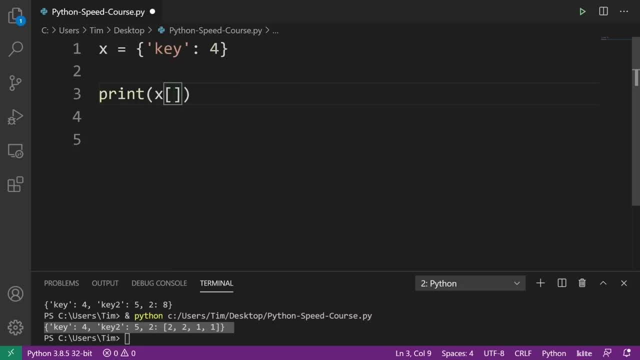 most of you know, anyways, what we can do here in terms of operations on the dictionaries. we can check if something is in the dictionary So I can say, okay, is some key in the dictionary, key in X. There we go. 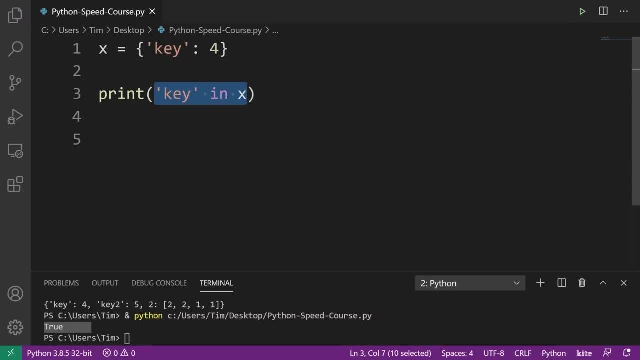 Print that out And that says true. A few of the useful things that we can do is we can get all of the values from the dictionary, So we can say X, dot values. print that out And it says dict values and it gives us a. 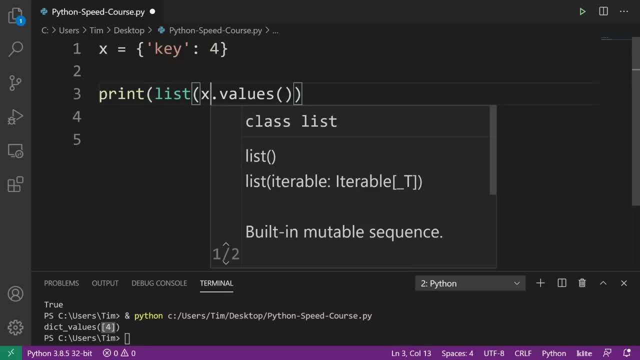 list of four. Usually, when you do this, you're going to want to actually create a list out of this, because that is a different data type that that's returning to us. And there you go, We get to the value for now. 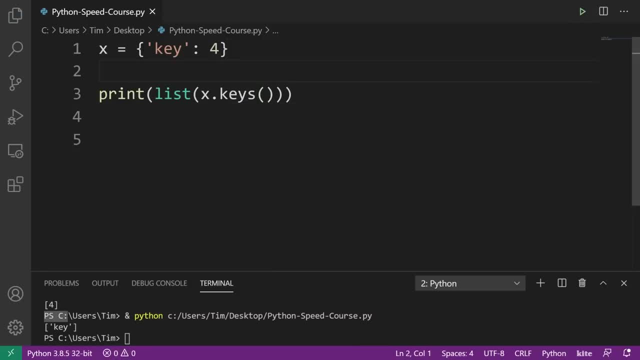 Similarly, we can do a Dick dot keys, So X dot keys, And there we go. We get a list that has all of the keys in terms of iterating over or deleting values. I'll first show you how you delete something. to delete something, We can say: 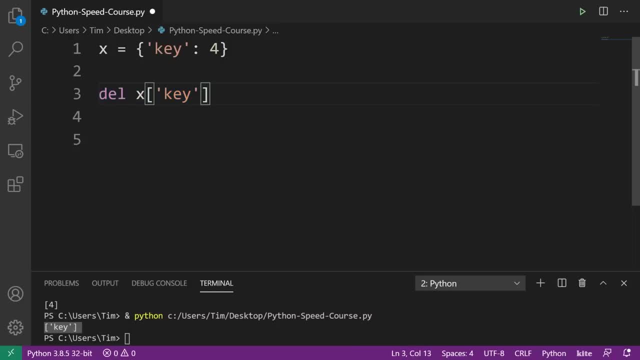 X, uh, and then the key that we want to remove. in this case, it will remove this key, So let's go ahead and do that. Uh and well, I guess. uh, it didn't really show you that it was. 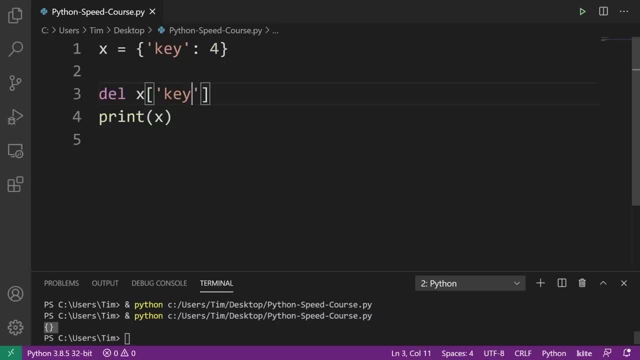 deleted. Let's just print it out to prove that. there you go And we get an empty dictionary. of course, like I showed you before, we can use that in operator and to loop over it. There's actually a few interesting ways that. 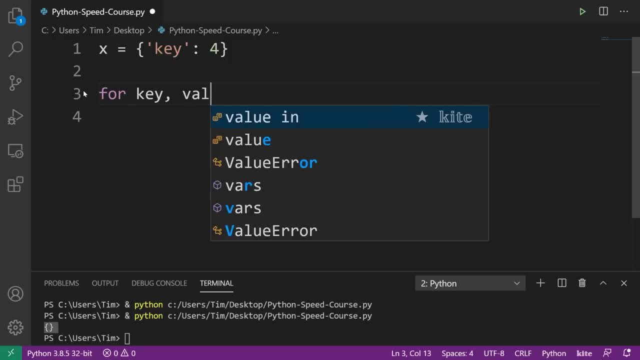 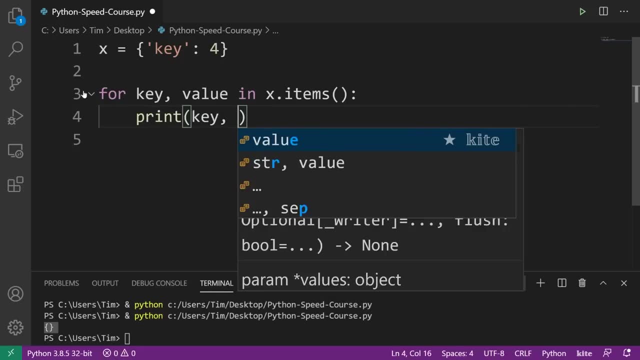 we can do this So I can say for a key: uh value in X dot items, And then what this will do is simply returned to me all the keys and values So I can print key value and you'll see we'll. 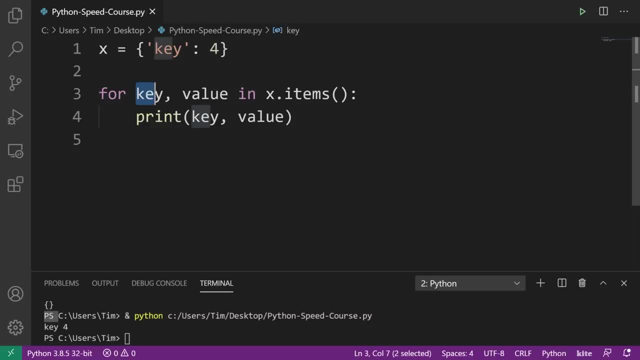 get a key for. so if I want to loop through all the keys and all of the values, I can use dot items. If I don't want to want to do that, I can just say for a key And then I can say in X: what this? 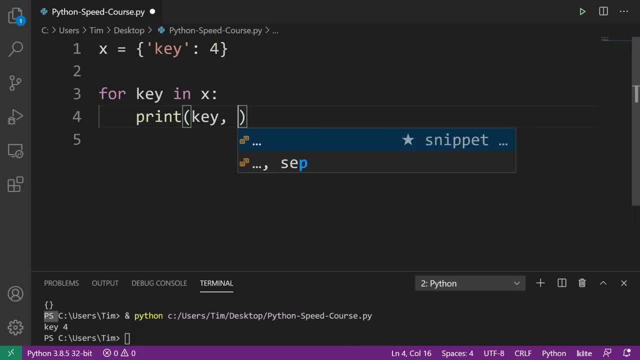 will do is simply just give me all of the keys in X, And if I want to access the value, of course I can say X key, like that, And that will give me the value And we get the same thing popping up there. Uh. 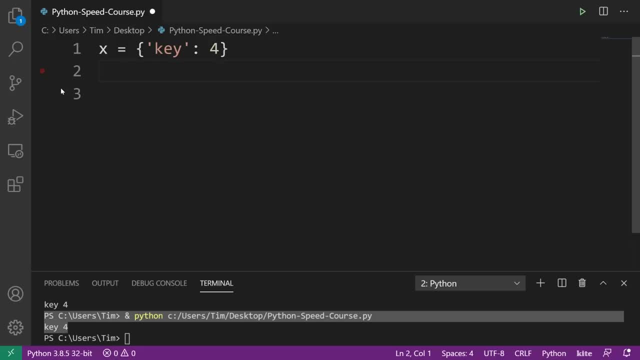 that's kind of the basics for the dictionaries. There's a few other methods as well, but I'm not going to talk about those. Um, that is a dictionary, And this next one is a fun one. This is comprehensions. Now, as 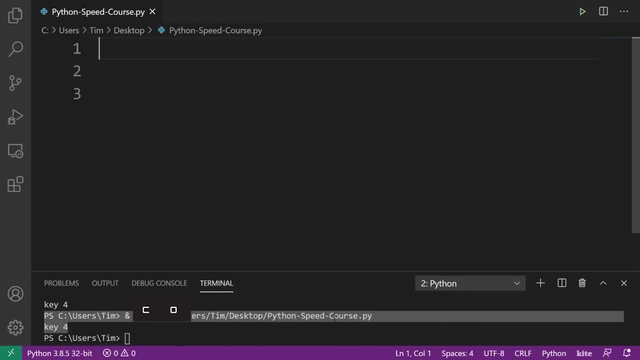 far as I know, Python is one of the only programming languages that actually has this. A lot of people absolutely hate it, but I personally love it, And if you learn to love it, you can use it quite well. Now to do a comprehension: 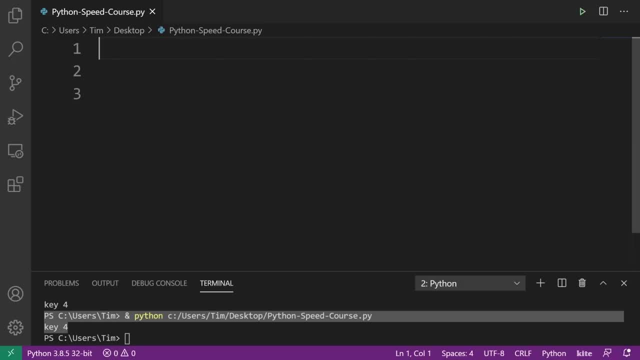 essentially what that is is a one line initialization of a list, of a topple, of a dictionary, of many other things. So let me just show you what I mean. I can do something like X equals a list, and then I can say X for 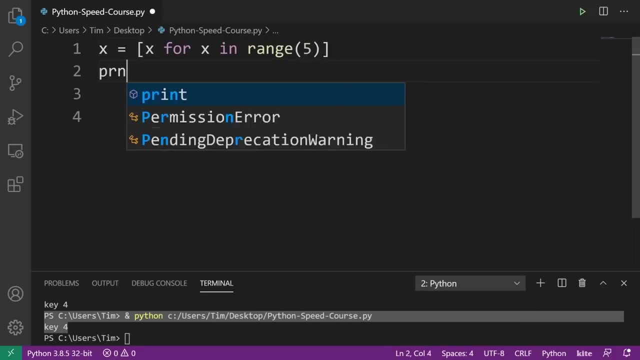 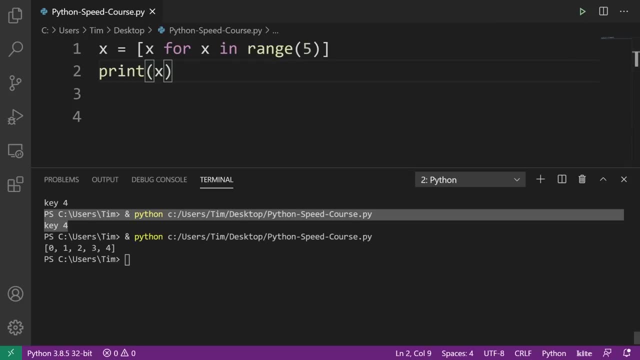 X in range five. Now, if I go ahead and I print the value of X, you're going to see what we get here. Uh, let's run it like that. You get zero, one, two, three, four The way. 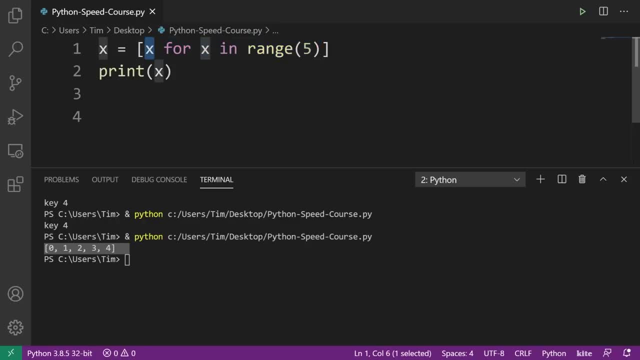 this works is essentially we can actually define a for loop inside of this list And what it will do is say, okay, we're going to loop through as if we normally would And whatever we have on the left-hand side. here is actually the element. 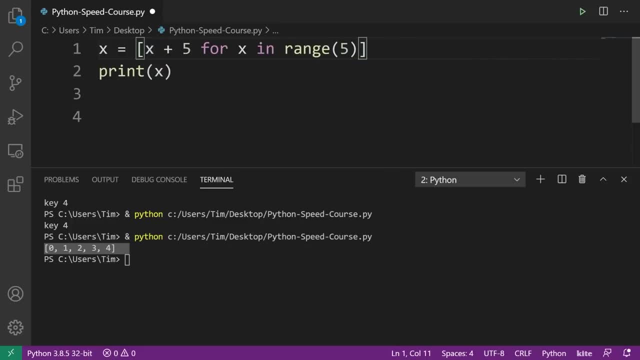 that we're going to add into the list. So I could do something like X plus five for X in range um five. And there we go: We get five, six, seven, eight, nine, 10.. I can also do something like: 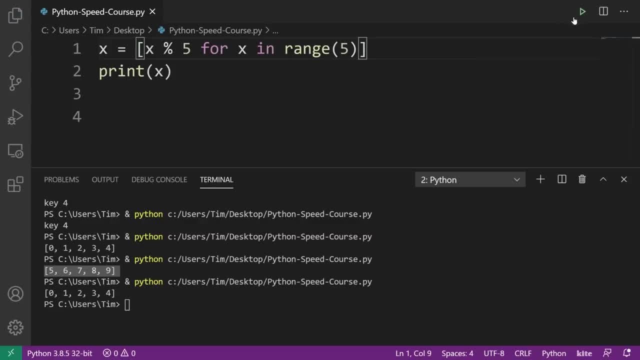 you know, X mod two and or X mod five. There we go. I can also, you know, grab something else. I could say zero for X in range five. That would give me a list of all zeros. You can see how. 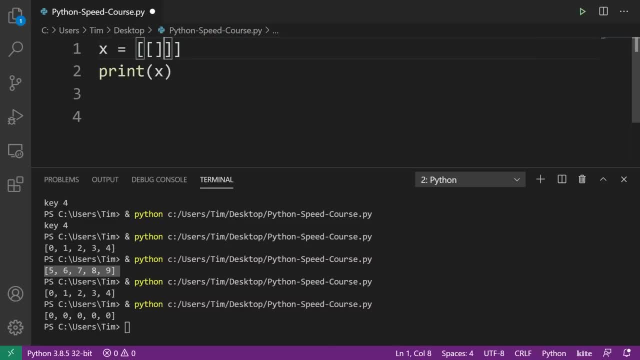 this might actually be useful. Now, if we want to go into a more complex example, I can do a list And then inside this list I could say zero for X in range a, hundred for X in range five. Now, what that's going to. 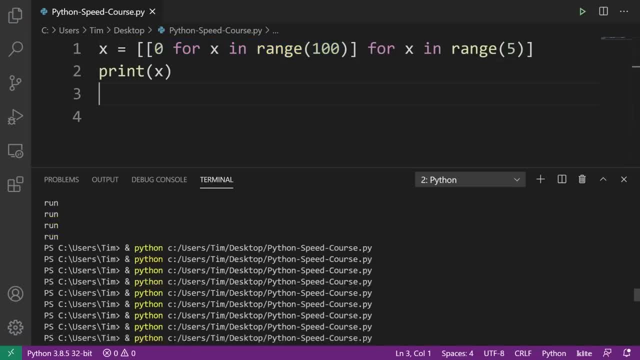 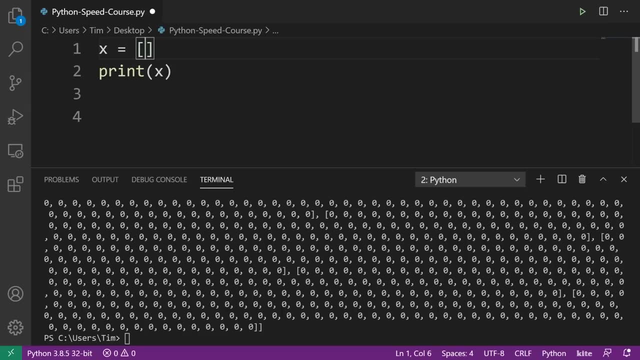 give us is five of these lists that each have a hundred zeros inside of them. You can see that's quite large, but that is kind of how that works. Now we can also go ahead and add some more complex stuff to this too, I mean, 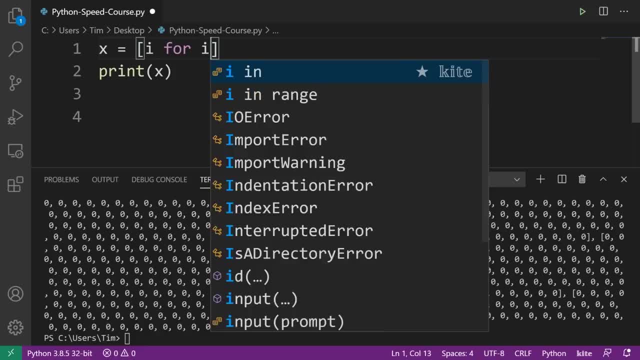 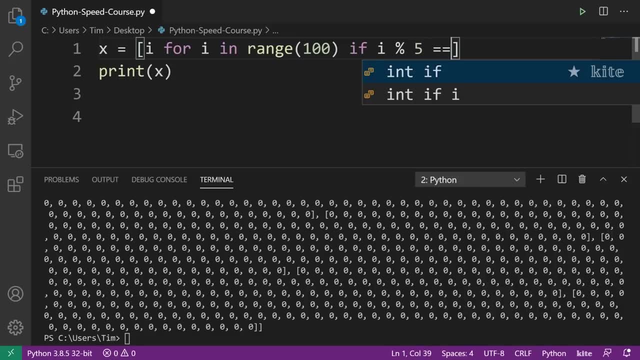 it's a zero four. or I can say I, for I in range a hundred. if I mod five equals equals zero. So essentially, if if I is divisible by five, then what we can do is actually add it into the list. Let's have a look. 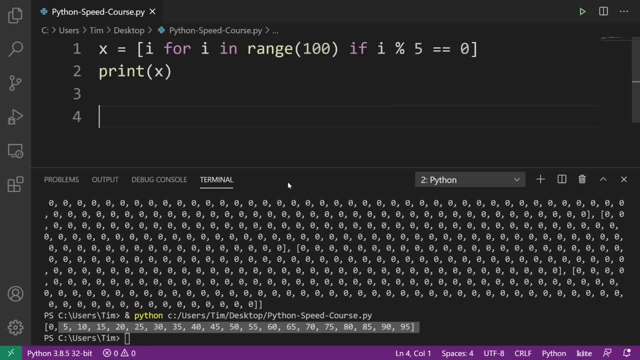 at that. And there we go. We get all the increments of five. So you can play around with that and see how that works. but this also works for dictionaries, In fact. let's just do the same thing here. Let's make it a. 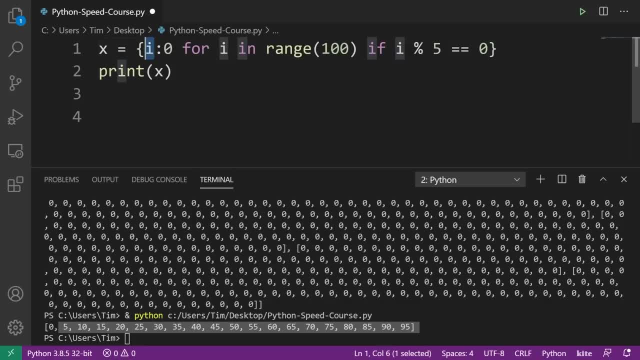 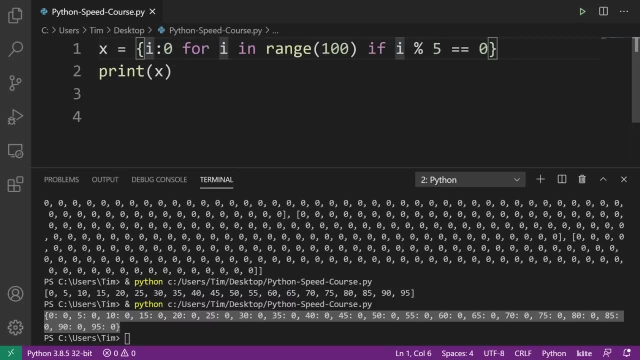 dictionary, and now we'll just go. I colon zero. So we have all these keys that are initialized at zero. We go there and have a look. We can see that dictionary works, And of course we could, uh, do the same thing for a set. We can just. 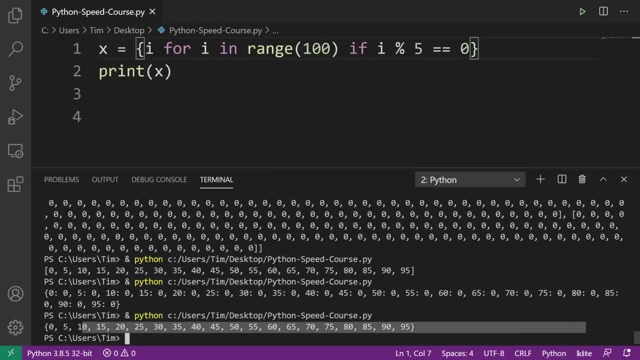 say: I for I in range, blah, blah, blah. And there we go. Now we get a set. So we can actually do this for tuples as well, except we're not going to do it in the way that you might assume. Uh, if 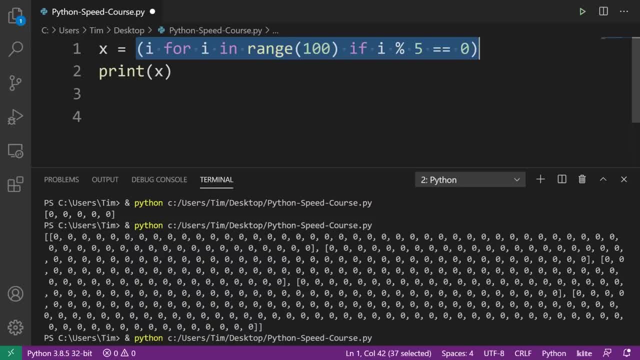 you just go ahead and do this. this actually returns to us what's known as a generator object. It's a bit more advanced for this kind of video, So I'm not going to talk about that, but what we can do if we want to make. 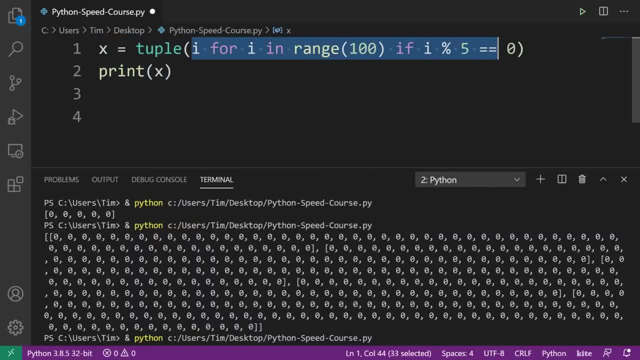 this work for tuple? is we actually type tuple? We can use the tuple constructor, which is simply this, and then do the comprehension inside of there. Now, that will return to us the tuple. You can see, I tried to do it the other way before and 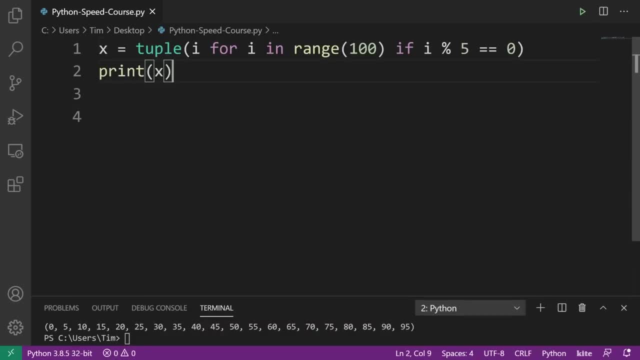 that returned to me the generator object. Anyways, that is comprehension. These can be used in a whack of different things. They're definitely interesting and good to know And one of the best features of Python that is not in many other languages. 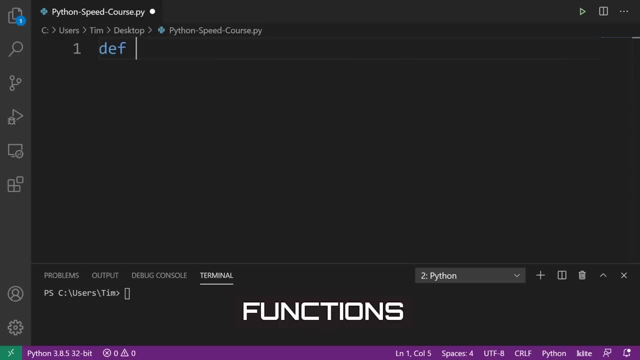 So now I'm going to start talking about functions. So to define a function in Python, you simply use the def keyword- This means define- then you pick your function name. In this case I'm going to pick funk. The function names are the. 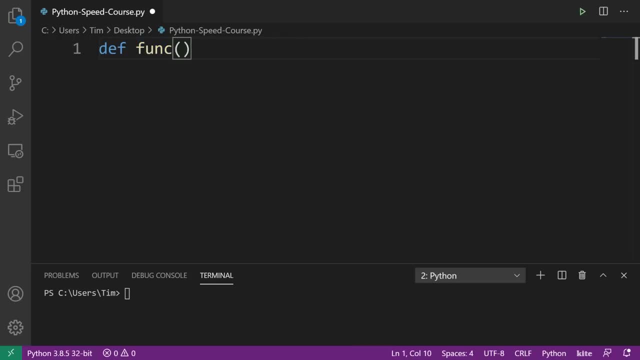 same as variable names in terms of how you name them. You can put some positional uh parameters inside of them or you can leave it empty. You add a colon indented block. then anything inside of the indent will run when you run the. 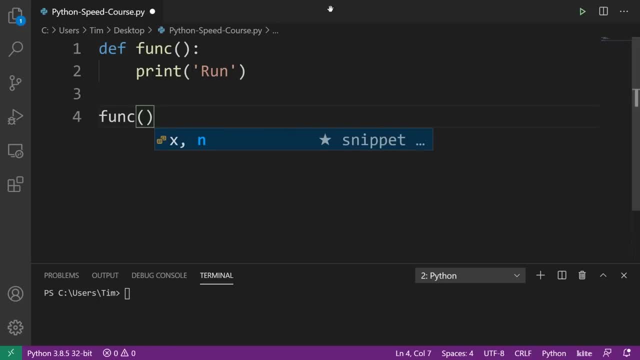 function. So let's go ahead and actually just run this and show you the basics of this. So that is pretty much how you run and define a function. Of course, you can define multiple functions. You can actually define functions inside of functions, If you. 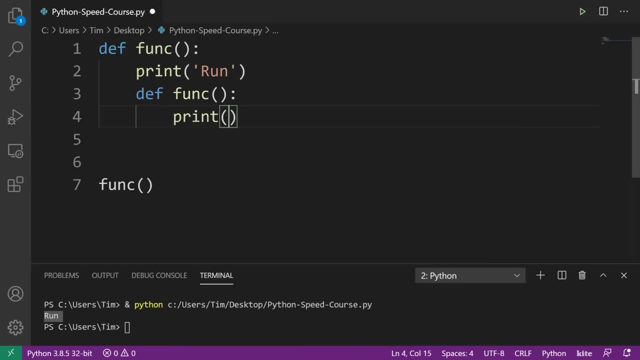 wanted to. uh, this is totally valid If I wanted to do something like this and then I could call funk like that. Now, of course, this is a more advanced use case, but just showing that you can do that because of the way. 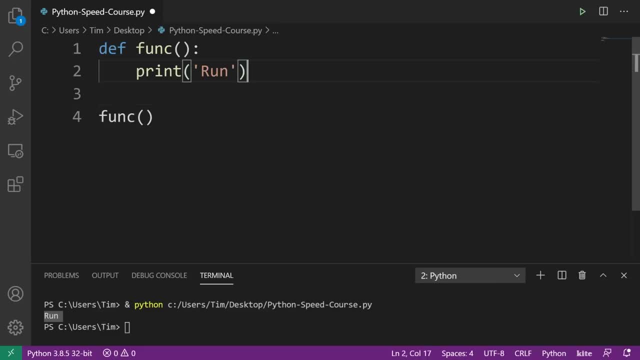 that Python works. In fact, functions are actually objects, which means you can technically return them. I'll show that in a second, but let me talk about arguments first. So let's say I want to add the argument X, Y inside of here, Of. 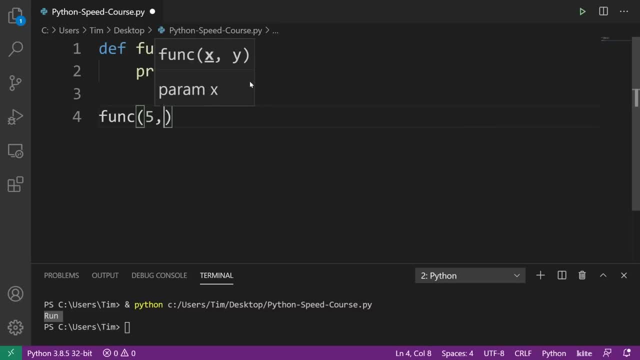 course that means now, when I call the function, I need to add some value for X and for Y. So let's go five, six And now, if I after run want to print those, I can print X and I can print Y. 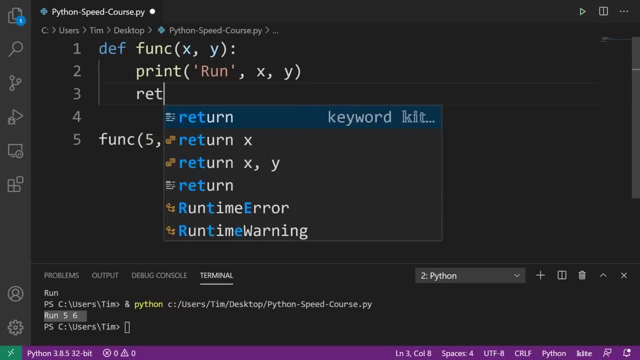 let's have a quick look. We get run five, six. Of course we can return something from a function as well. Maybe I'll return X multiplied by Y. Now, if we actually go ahead and print the value of this function, what? 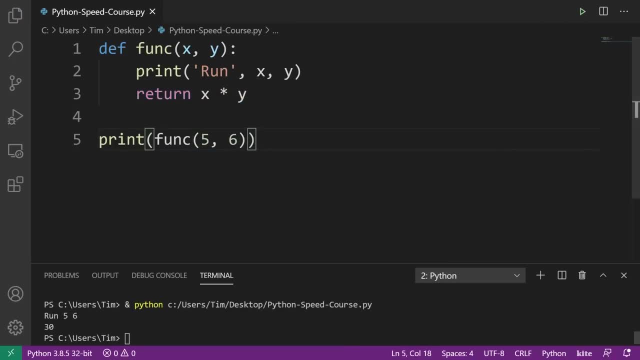 will happen Is it will evaluate what is here, return that to us and print that out. We get the value 30.. Now notes that when you return multiple things from a function, which you can do, I can return X, multiply by Y and maybe. 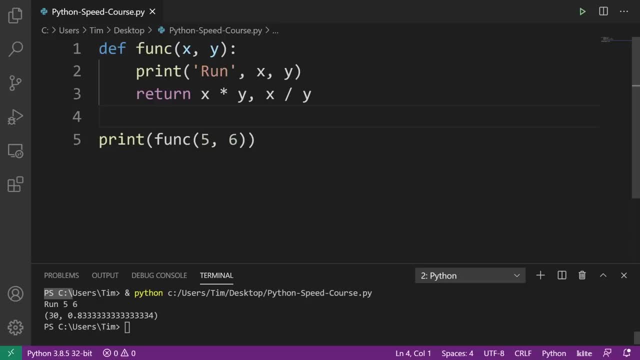 X divided by Y as well, This will return the value to us in a tuple. So if you look here, we get actually two values. We have, I guess, the X, Y value here and that's inside of a tuple. Now, if we 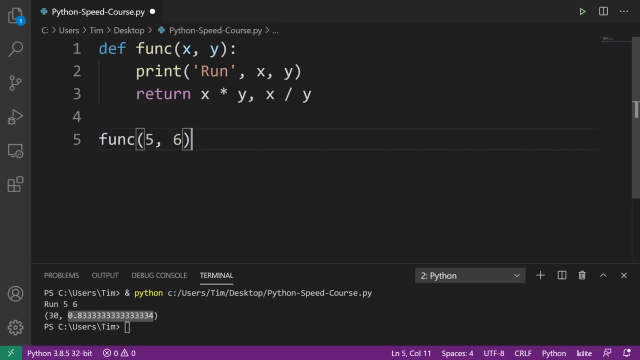 want to unpack this tuple and say: separate this out into different variables. we could, of course, index at zero and index at one, but a much cleaner and faster way to do Do this is to do something like R one comma, R two equals. 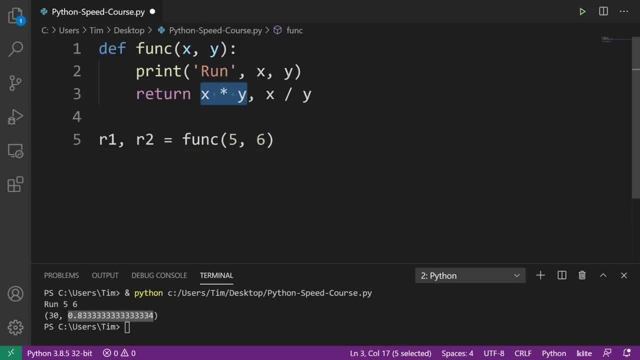 funk, five, six. What this is going to do is take these two values here and simply separate them into the R one and R two variable. Now if I go ahead and I print R one, R two, and I have a look here, you can see. 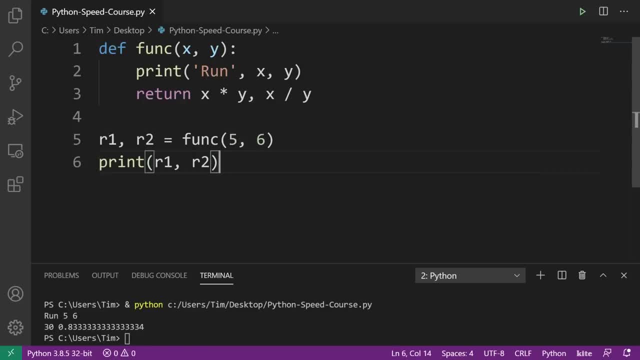 that we get 30 and then 0.8, three three, three, four. That is the basics for a function. If you want to do a optional parameter, you can do something like Z equals. You can set a default value. I. 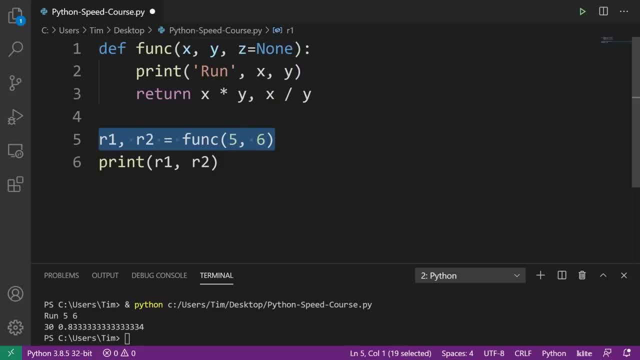 usually set it as none, And what this means is that you do not have to pass. set in, but if you want to, you may, And it will override the optional value that you have here. So let's just start by actually printing out. 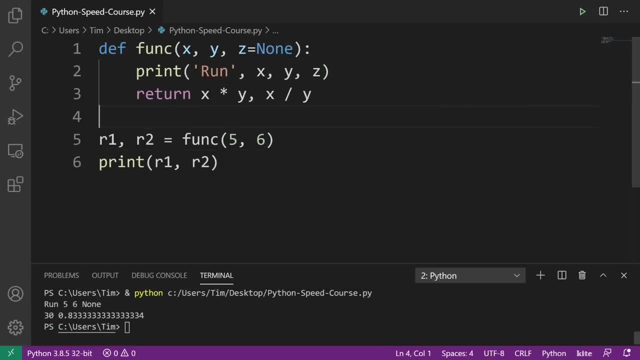 Zed. I'm not going to call it with Zed to start. You can see that, uh, oops, let's run that for a second. We get run five, six, none, And now if I add a Zed, so let's just 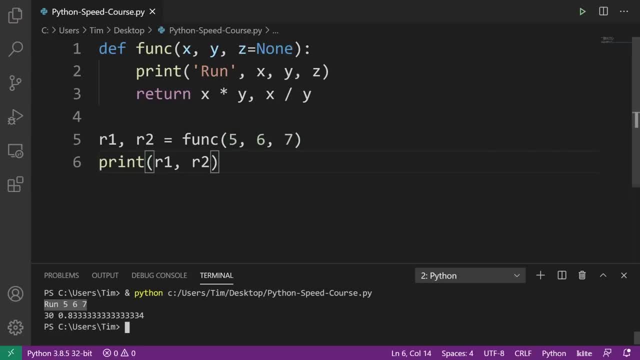 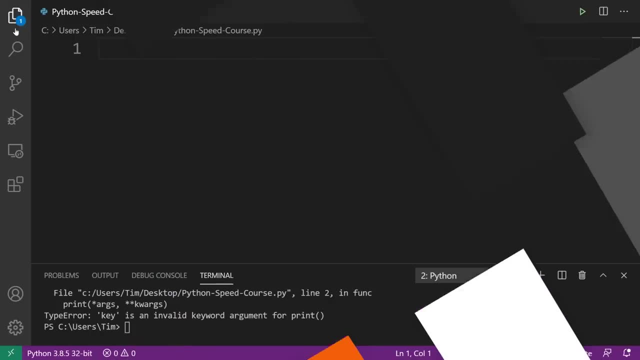 add seven there. We see then seven. none, We are going to get seven printing out right there. That is the basics of a function, And now we're going to move on to some other, more advanced aspects of it. All right, So I'm. 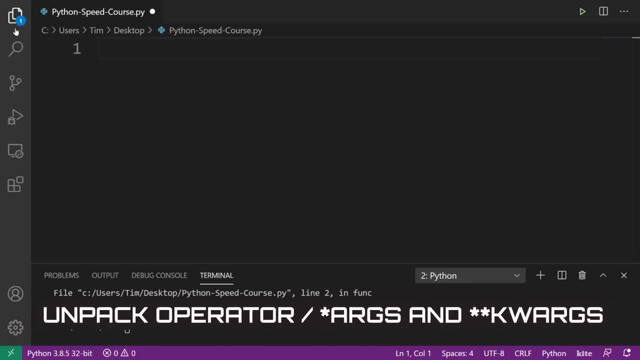 going to talk about something that's really cool called the unpack operator, And then I'm going to talk about star args and star star quarks, But I first want to show you an advanced example of a function. So if I say define funk, like 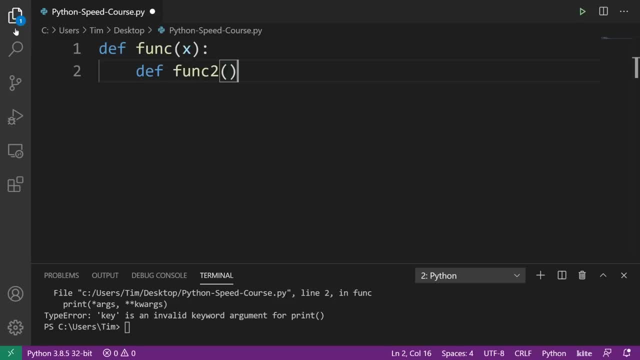 this, and then maybe I'll say: take X and I define funk to inside of here. this is totally valid, by the way. You can put a function inside of another function And then inside of here. what I'm actually going to do is say this: 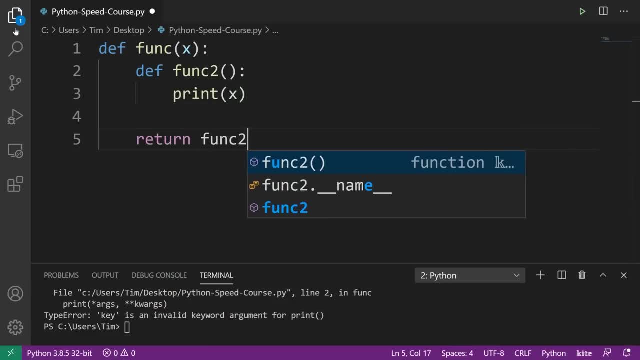 function is going to print X and I'm going to return funk too. but notice, I don't call it Now. this is just to prove to you that functions are objects, Hence they can be passed around just like variables. So what I can actually. 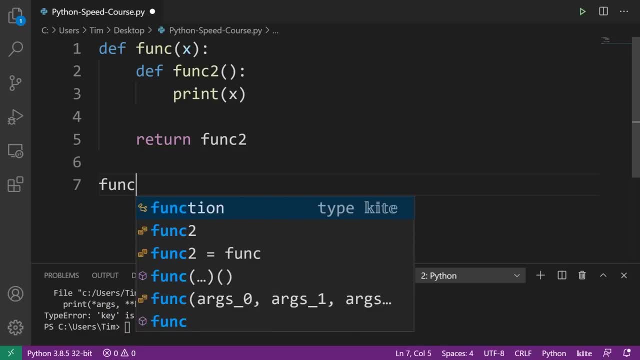 do here is I can go ahead and I can say print or sorry, not print, but I can call funk four or funk three, And then I can actually call it like this, What this is doing, essentially saying, okay, I'm going to call this. 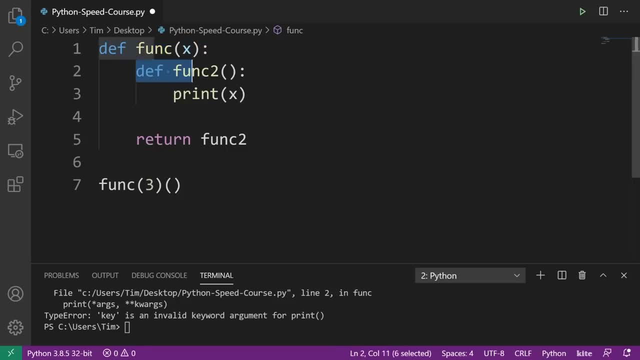 function here with the value three. What this function does is it returns to me another function. So it gives me funk to notice It's not calling the function, It's simply returning it. Now I'll actually just show you what I mean. first, 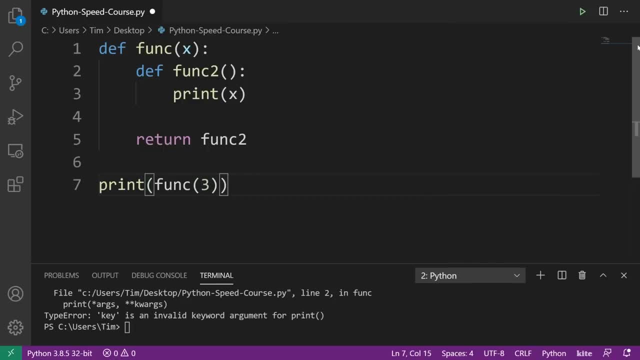 before confusing anyone, Let's print this out before I do the call statement on it. But you can see that this actually tells me this is a function object. It's a funk dot. locals funk too. So it's pretty much saying that funk too is. 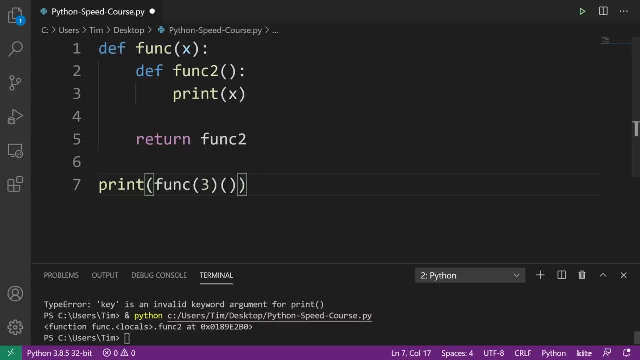 defined within funk. Now, if I'm going to actually call this, because that's just the function, reference or object, it's not actually, you know, being evaluated. If I call it like that, we can go ahead and we get three, and then we 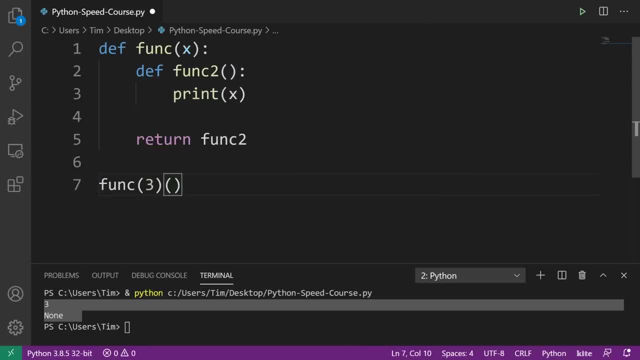 get none. Of course, the print statement is going to print none because there is no. there's nothing to print from the return of funk too. but just have a look here We get three. Now this is equivalent. If I did something like this, I 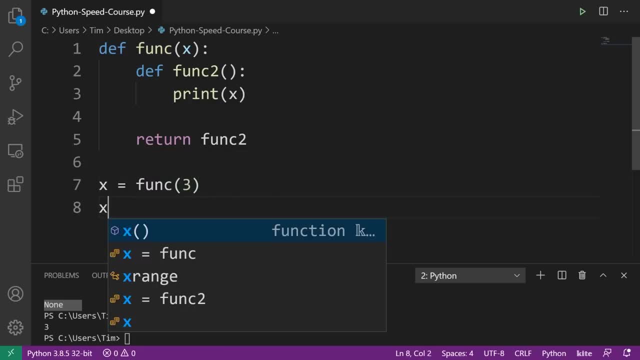 said: you know, X equals funk. And then, on the next line, I just called X. since X is equal to a function, funk too, I can call it just like I showed you before. And there we go, We get three. Anyways, that's the. 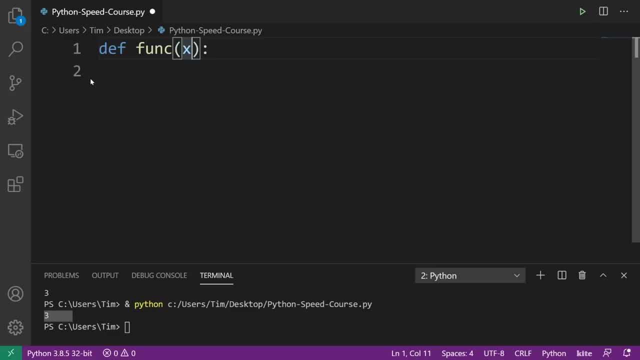 advanced aspect I wanted to show. Now, what I want to do is show you about star args and star star quarks. Uh, so I'm going to put in like this, All right, So before I define what this does, what I'm. 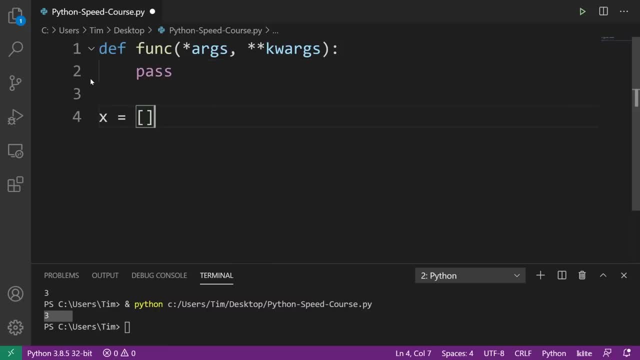 going to do is just show you what the unpack operators in Python. So let's say I have a list, maybe we'll call it X, and we just have a bunch of random numbers in this list. So what the unpack operator does is actually separate. 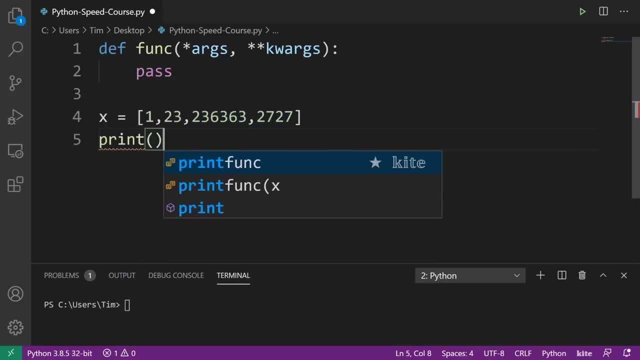 all of the elements from a list or from a collection into individual elements. The best example of this is the print statement. If I print asterisk X, it's X, which means unpack X. What this is going to do is take all of. 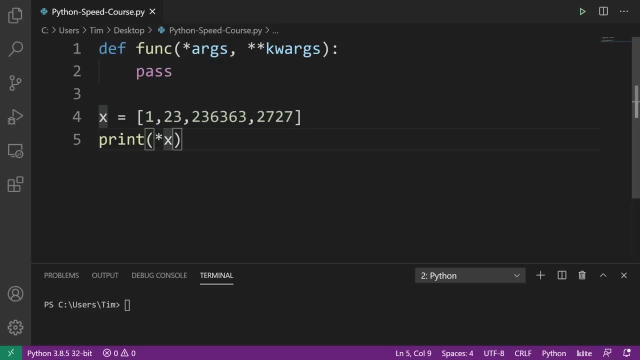 these elements out, So separate them by individual elements and pass them into the print statement as arguments. So instead of just printing, you know, say, the entire list, what it's actually going to look like is: print one comma two, three comma two, three. 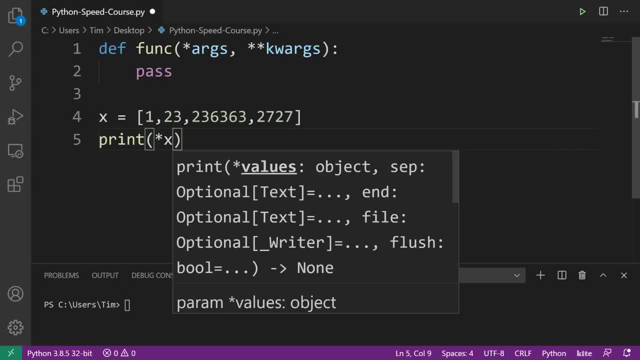 six blah, blah, blah. You get the point. That is what this is going to do. So just have a look at what happens when I print that. I get all of these things separated by spaces, like what happened if I just. 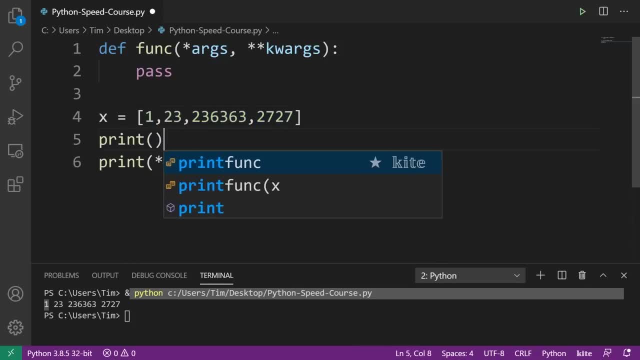 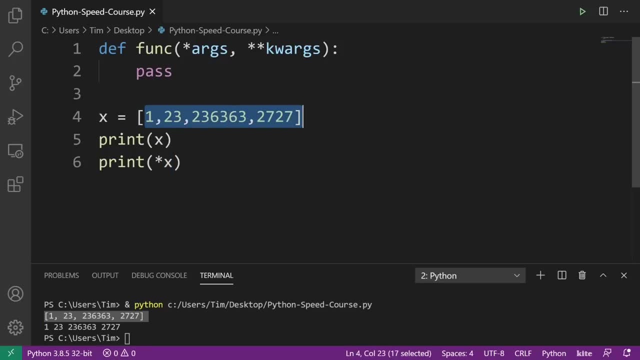 pass them in individually, not being in the list. Now look what happens when I just print X. Let's have a look. See, it actually prints the list out. So what this does is unpack whatever we have in a topple or a list or 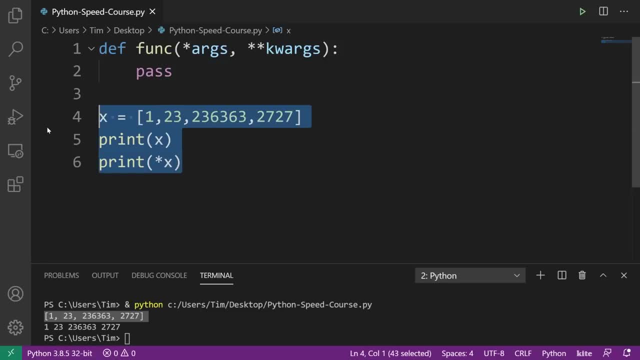 some kind of collection and sends it through as arguments to a function. So that's where star arcs and star star quarks come in, Although you'll see that in one second. So let's say: I have a, you know X, Y. 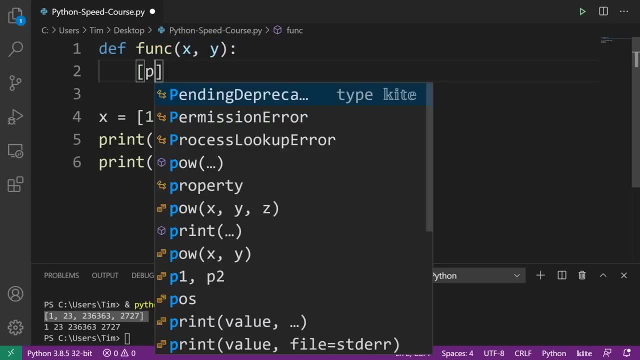 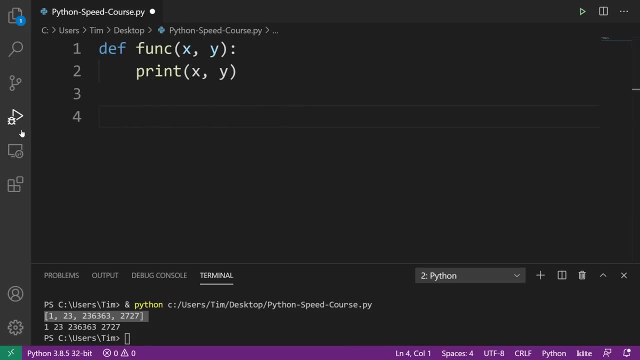 that we need inside of function. We've got to pass X- Y. what this will do is simply print X and then print Y. Now let's say I actually have maybe a bunch of pairs that I want to pass this function, So maybe 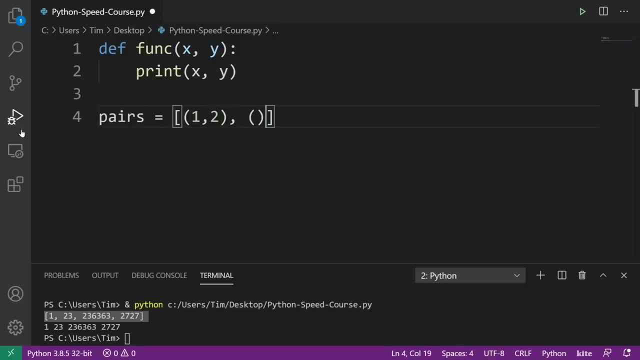 that's, you know, a say Paris equals, and then I have like one, two, three, four. Well, what I'm going to do is do a four looping and say four pair in Paris, And what I want to do is call this: 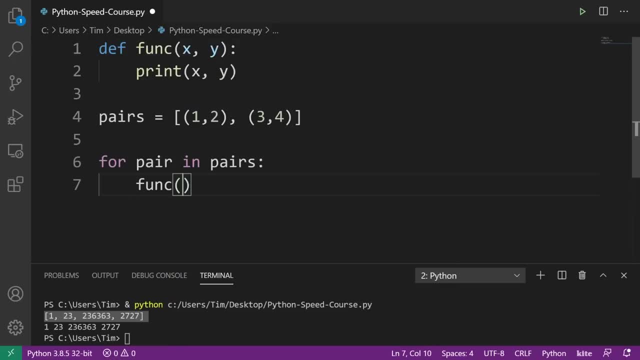 function with those pairs. Now, the naive way to do this would be to go funk: Okay, Pair zero and then pair one. great, That would work. but that is not to be Pythonic way to do this. What we can actually do is do: 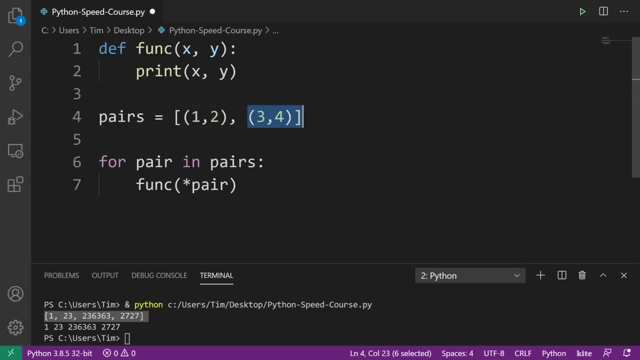 asterisk pair And what this will do is take one, two and take three, four, unpack them, separate them and pass them as arguments to funk. So if you have a look at that, that actually works And that is why the unpack operator is. 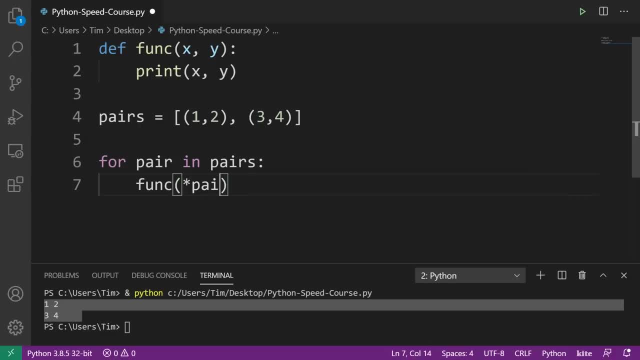 really useful. You can also use this actually on dictionaries as well, And I'll show you how that works with dictionaries a little bit more complicated: involves two asterisks. What this does is, if I have keys, I can say X, representing obviously the argument. 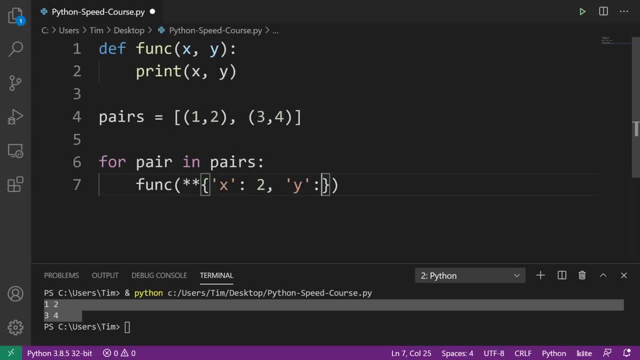 X and then make that equal to two, And then I can say why- and this could represent the argument Y, and I'll make that equal to five. Now, if I run this, this works fine. I needed two asterisks because this was a. 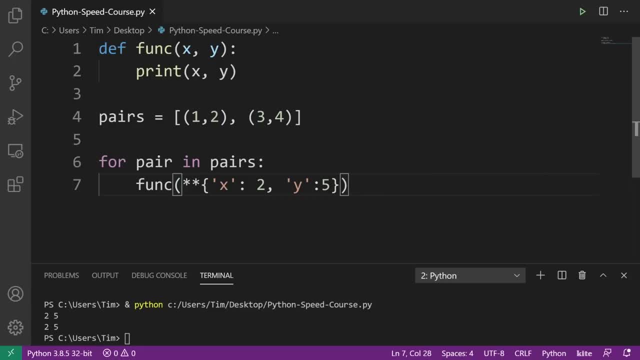 dictionary. Uh, and that is kind of how this works. Um, yeah, I don't, I guess, really need the four loop anymore To illustrate this. uh, but the double asterix is used for dictionaries, The single asterix is used. 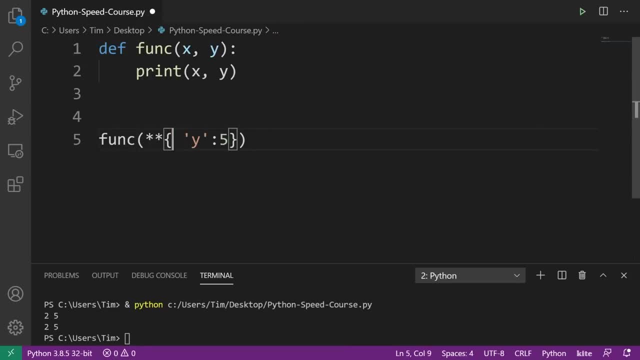 for a tuple or for a list. Now, I just want to make the point here that, let's say, these are not in the correct order, So it's Y and then X. this will still work, And that's actually why this is really useful, because 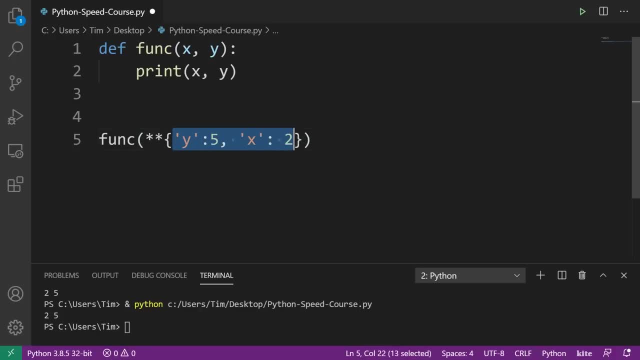 you don't have to have it in the correct order So long as you name the arguments as the keys. So now, hopefully that will explain to us how star args and star quarks work. So star args and star star quarks- essentially imagine you. 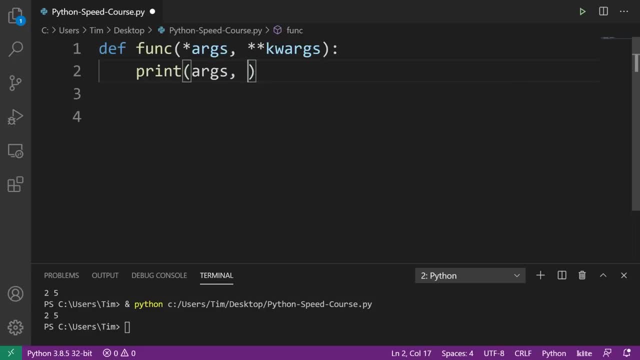 have a function and you don't know how many arguments- positional or keyword arguments- you want to accept. This is what quark stands for: keyword arguments. Well, what you can do is you can use star args and star star quarks, And what that will do is allow. 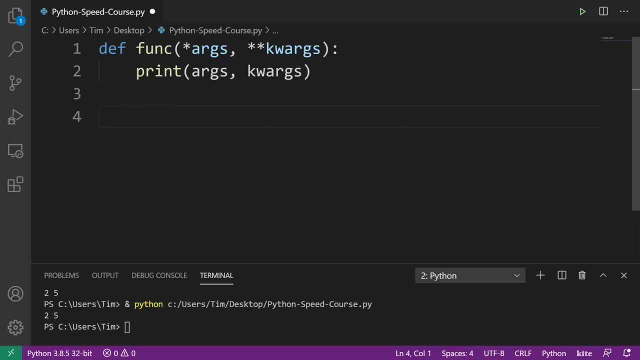 you to pass in an unlimited amount of regular arguments and keyword arguments. So if I actually go ahead and go funk and then I pass like 1,, 2,, 3,, 4,, 5, and maybe I'll pass some keyword arguments- 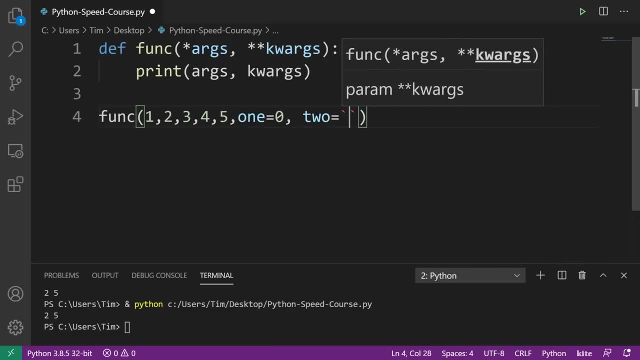 like you know, one equals zero, two equals one. I know this doesn't really make any sense, but you get the idea. Now, if I actually run this and print it out, you can see that when I print args and print quarks, we're getting. 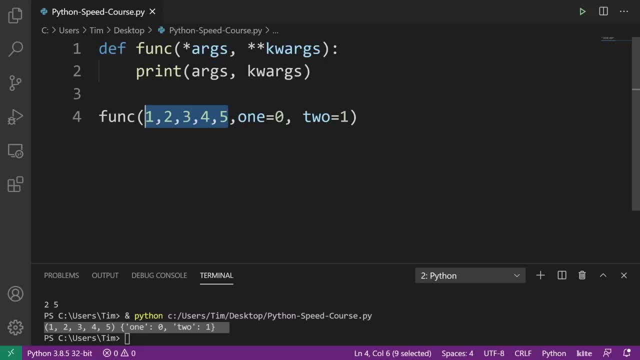 a topple that has all of the positional arguments, which are these, and all of the keyword arguments, which are one and two. Now, if I wanted to actually use any of these, what I can do is I can unpack them. So, first of all, I can. 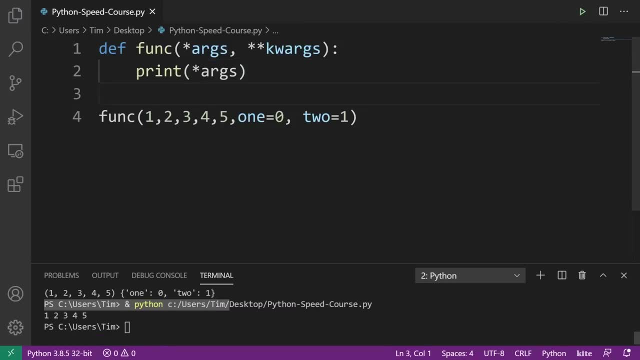 unpack args And what this does, if we have a look here, is it will print out 1, 2,, 3,, 4, 5.. I could try to unpack quarks, but you're going to see what happens when I do. 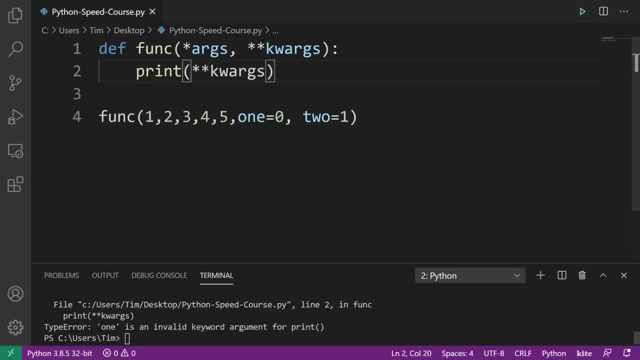 this And hopefully, if you remember the last example, you'll realize why this is not going to work. It says: one is an invalid keyword argument for print. So what this is going to do when I print this, when I unpack quarks, is it's going to take. 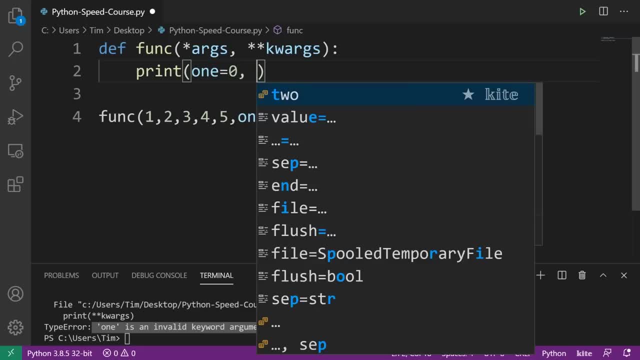 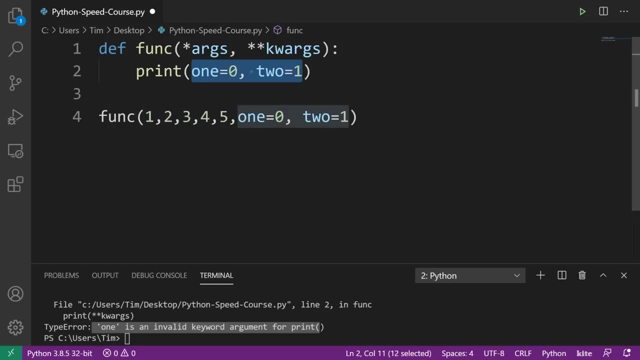 all of my keyword arguments. and it's going to say one equals zero And it's going to say two equals one and pass that to the print statement. Now, obviously, one and two, well, those are not valid arguments for the print statement. So 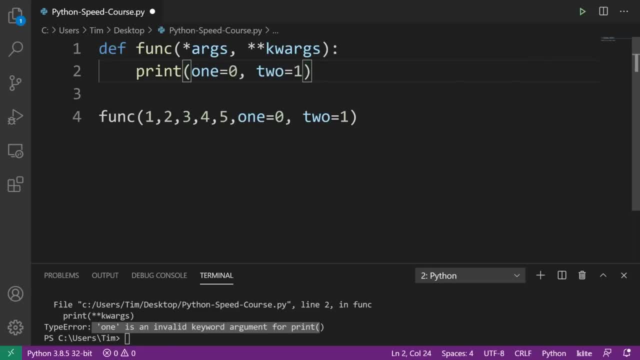 we're going to get an error anyways. that is args And that is quarks. Uh, you're going to have to look into this on your own and kind of learn about how it works. but that is the basics And I just wanted to show. 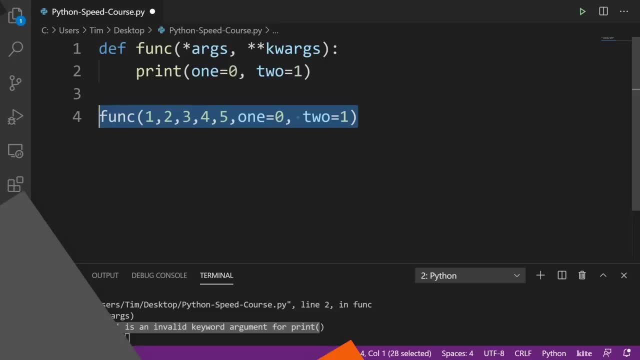 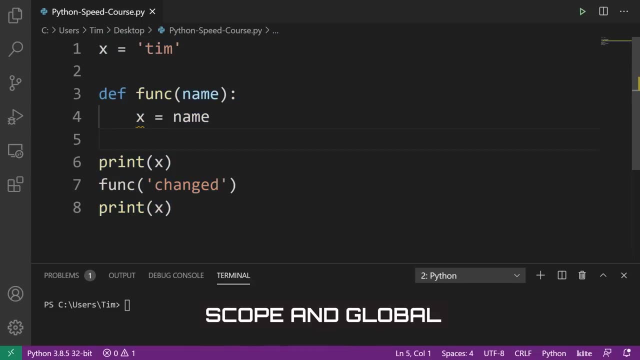 that to you so that you're aware that you can do these cool fancy things in Python. This next one is going to be very fast, but this is just defining scope and global. So when we look at a function like this, there is a notion of a. 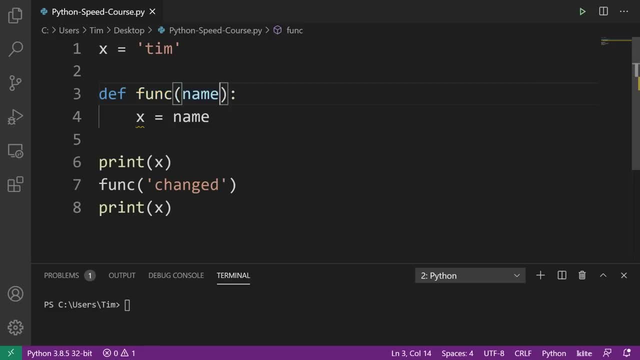 scope. So we have X equals Tim, we have defined funk, and then we have name as a parameter. And what we're doing is we're saying, okay, we're going to change X to be equal to name. So, essentially, if I was 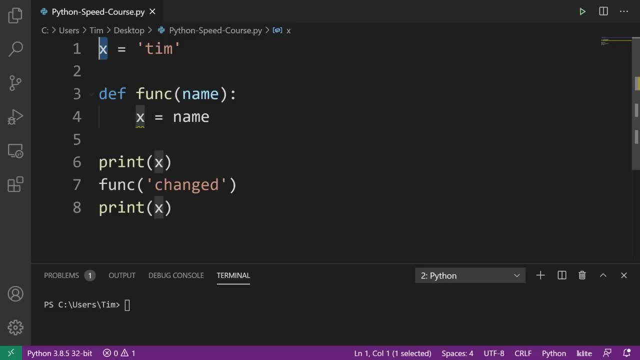 naive and I didn't know any better. I would assume that what's going to happen is well, this variable up here would change when I pass this name to this function. any of you that program before probably know that's not going to work. but if you have a 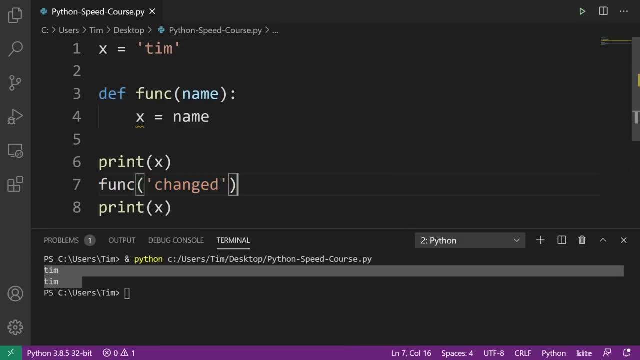 look here you can see that X does not change before or after when I call funk, with the string changed. The reason for that is that this X variable is local. It is within the scope of this function, which means it cannot be used. access changed. 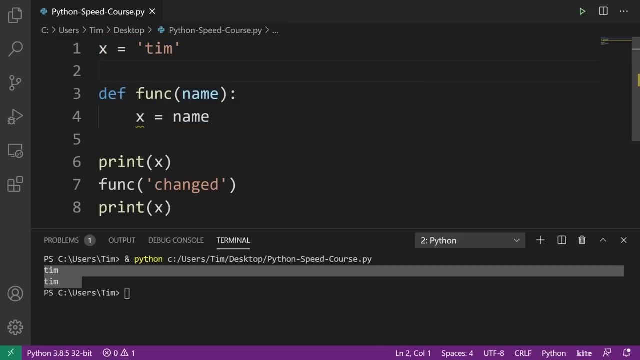 from with from outside. the same thing here with this X. this one is actually global. This is, on you know, not not defined within any scope other than this file, which means well, I can't just directly change it from. 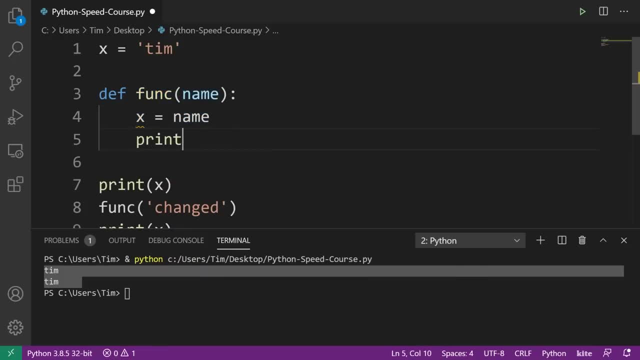 this function. I could, however, access it from this function. I could print it here, but I can't actually change its value, because if I do that, what's going to happen is I'm going to create a new X inside of here, which 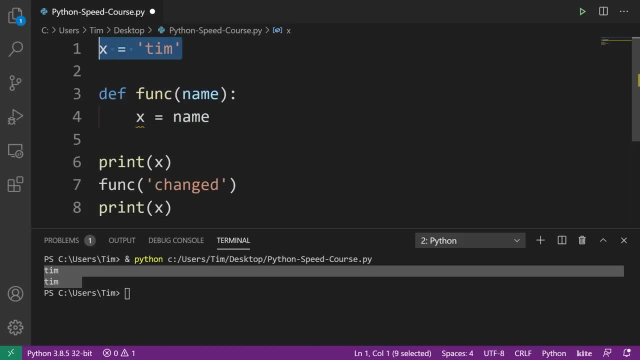 is equal to name and it will be local to this function. It will not modify this. However, there is one interesting thing we can do in Python, which is the global keyword. If I global X, now you're going to notice that the 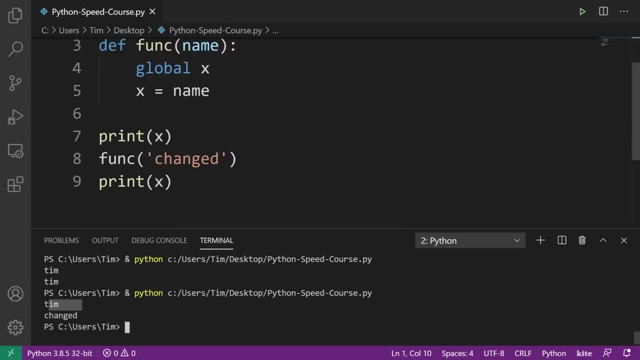 expected behavior will occur. Now we get Tim and we get changed. What that is saying is okay. I want to use X as a global variable, So I want to reference X in the global scope. never use this. This is never good to use And 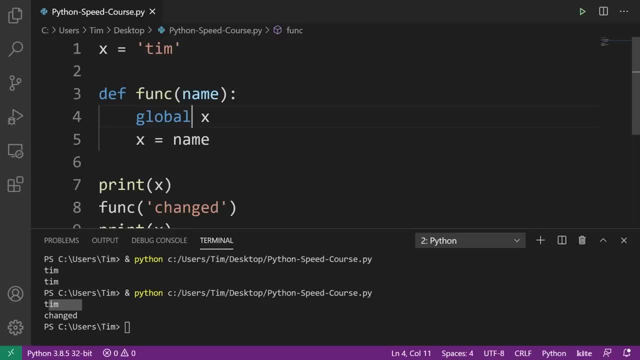 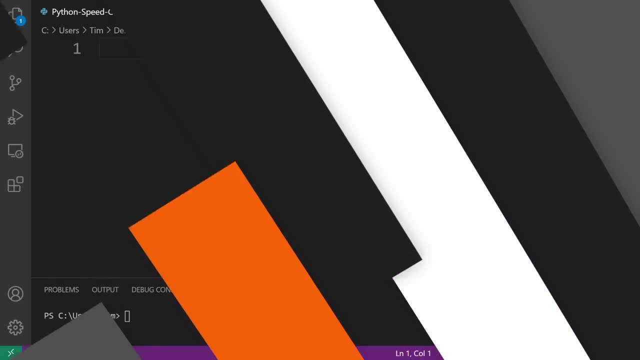 if I ever see a Python program that has it, I always get upset, but this is something that you can use And I feel obligated to show you because there is some very, very rare situations where you may need to use that. All right, So now I'm. 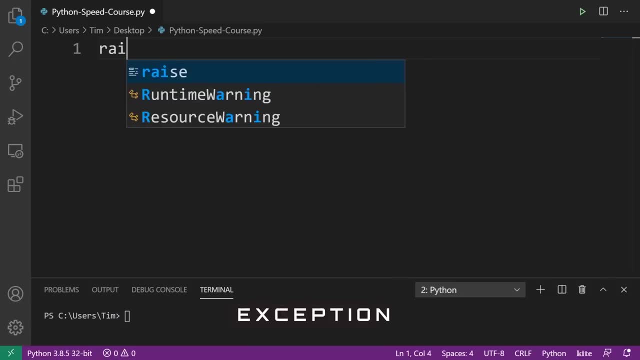 going to spend about 10 seconds showing you how to actually raise an exception. in Python There's a keyword called rays. Maybe in Java you've seen something like throw and raise can raise an exception if you want it to do that. 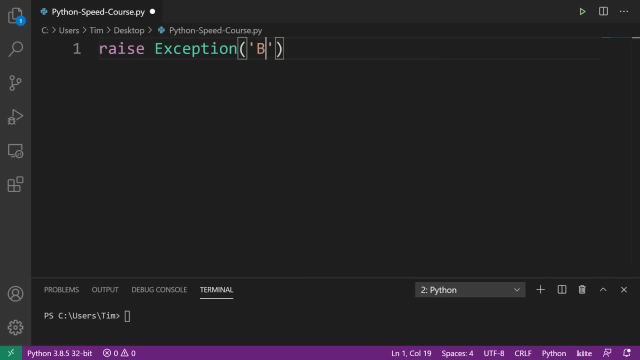 So I could raise exception And then inside of here I could just say: bad, you know whatever I want. Now, if I run the program as soon as we hit that line, immediately, I'm going to get an exception and it says: 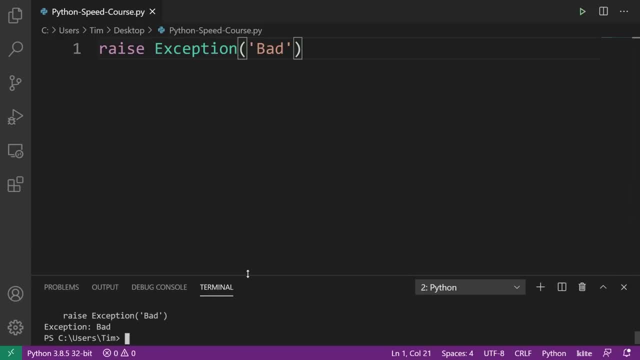 raised: exception, bad, exception, bad. Of course, that is the basics. There is more arguments and things you can do with this. This is a base class, which means you can extend it When you get to object oriented programming. make your 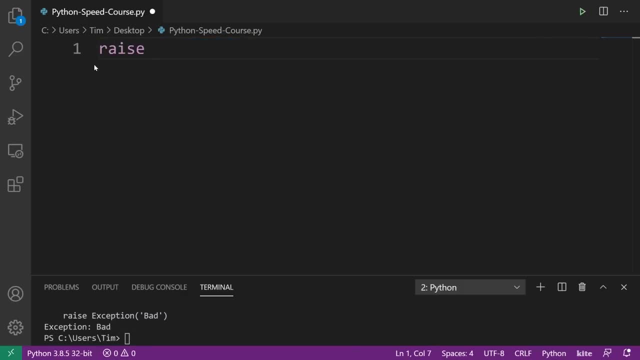 own exceptions and make all that fancy stuff. For our cases that's all we really need to know. I could raise, say, like a file exists error, any other kind of error that I want, And then again add some description for it by just putting a. 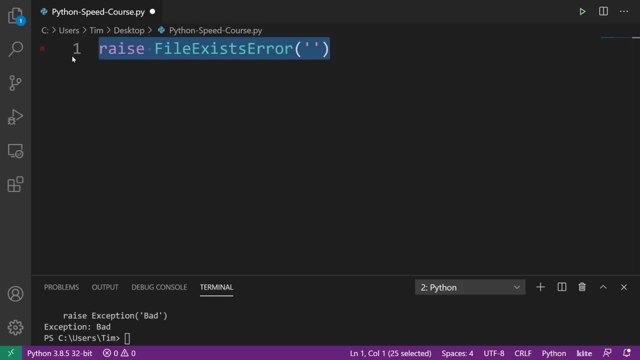 string inside of the brackets. but that's enough for that. Now let's show how we can actually handle exceptions. All right, So now that we know how to raise exceptions, it makes sense to learn how to handle them, So in Python rather than. 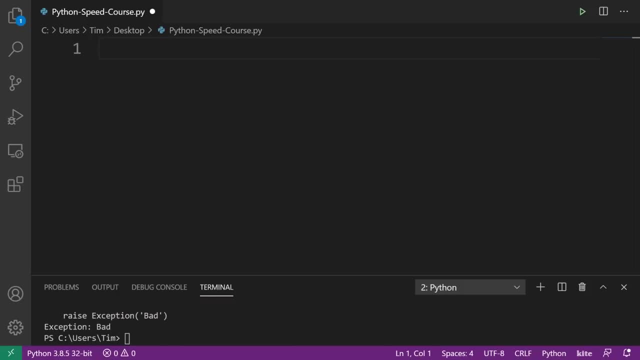 having like a try. catch, we actually have a try, except finally block. So what I can do is do something like try. That means I'm going to try to perform whatever code is inside of here. Maybe I'm going to get an integer division by. 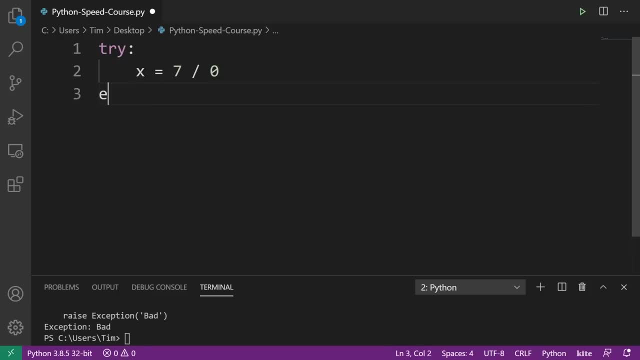 zero error. So I can do you know, seven over zero That's going to raise an error. Then I can create an except block, I can accept an exception as E. what this is going to do is mean whatever the exception is will be. 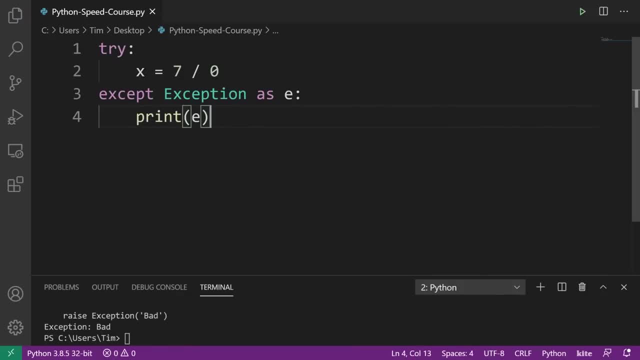 stored in the variable E and then say I could print out that exception and we can continue running the program. This is the basic try except lock. You don't actually need to define something here. I can just say try except, like that. 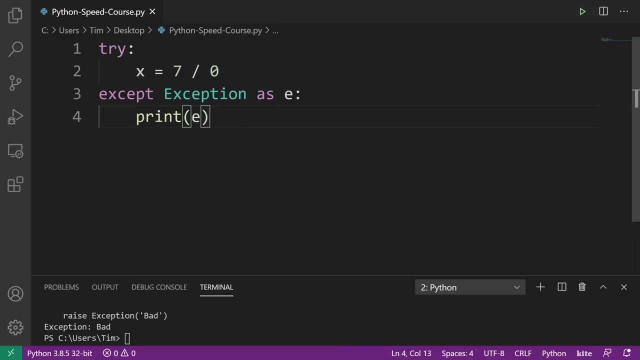 If I want and also accept a specific exception, So I don't have to just put exception. This is general. This means any exception that occurs I will actually catch. You can only catch specific exceptions if you want. But But again, that's up. 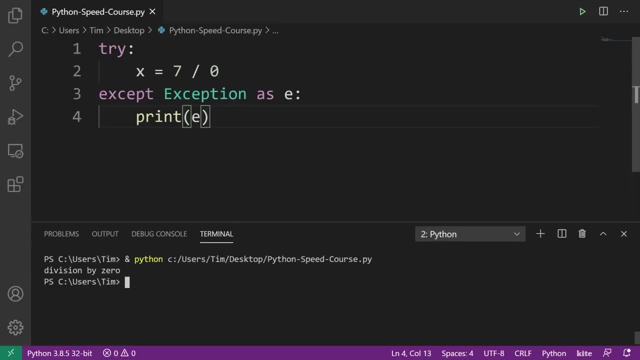 to you. So in this case, you see, we get division by zero. It's just printing out but it didn't actually raise, or, you know, show us that error. So it did raise it, but we didn't actually see it. 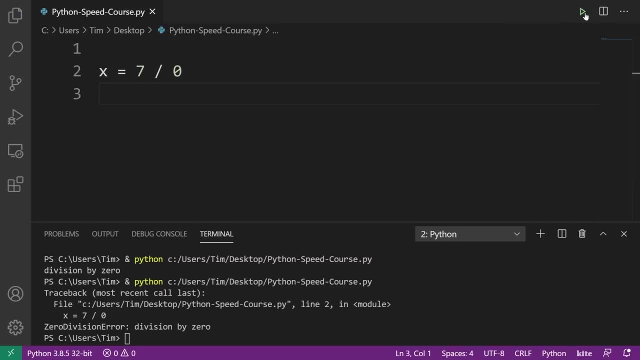 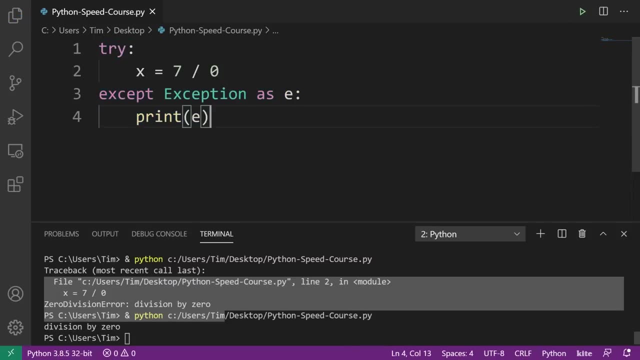 Now, if I go ahead and just do this, what we can do is we can say: Oh well, that is the actual problem, And now our program is going to crash and not work. But if we have this, except block, like this, of course we're. 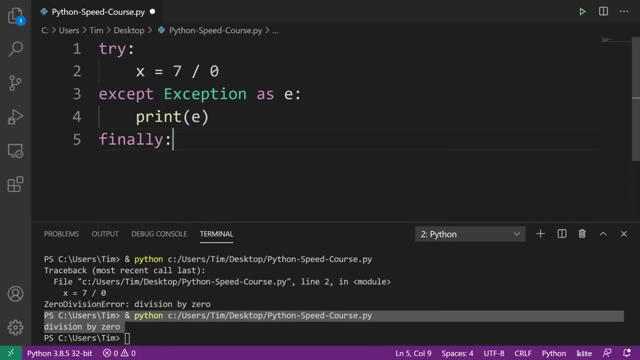 good to go. Now. there also is a notion of a finally block. The finally block will run no matter what. Usually you put cleanup type operations inside of here. Maybe you're trying to write to a file, some exception occurs, And then no matter if this 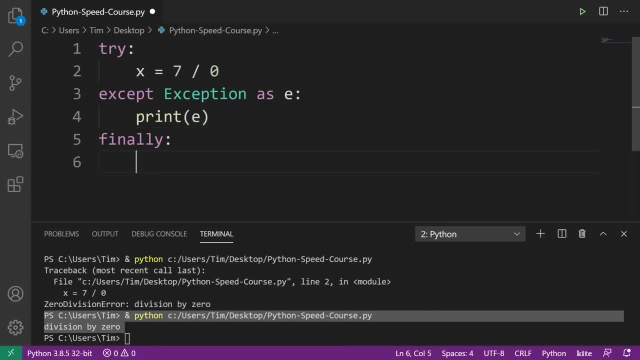 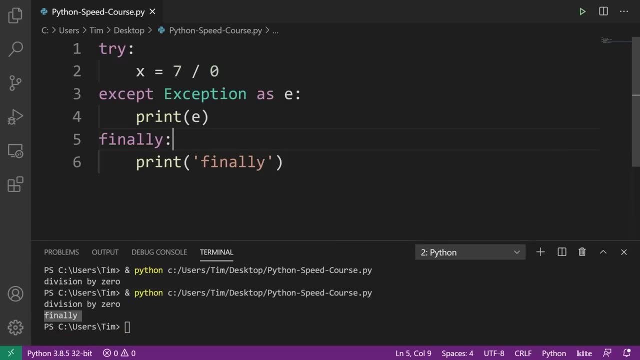 was successful or not. you want to close the file after you would put that inside of finally, So I could say print finally, like that. have a look here and you can see we get finally. I'm not going to go through this too. 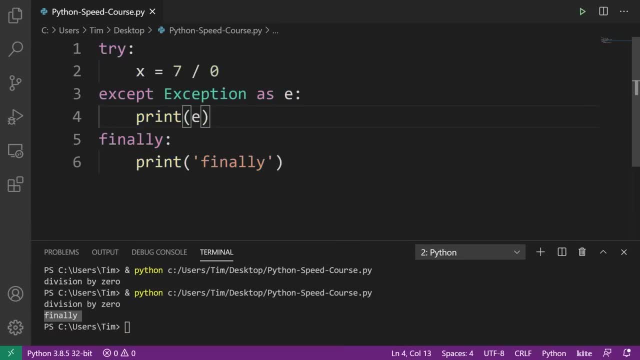 much. I assume, if you're going to be using this, you understand how try, except and finally work. but that is the implementation in Python And that is the basics for raising and catching an error. And now we're going to discuss the lambdas. So 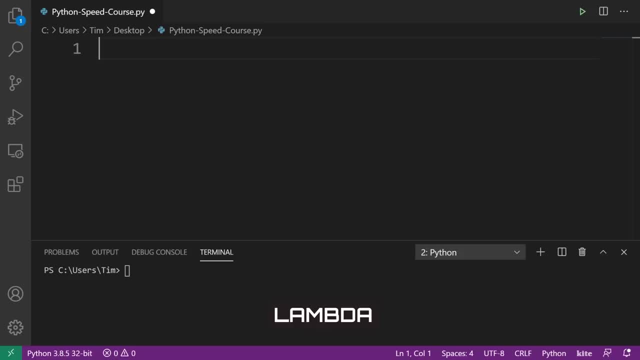 lambdas are actually a really cool aspect of Python. I'm pretty sure they have them in many other programming languages as well, but it looks something like this: Essentially, a Lambda is a one line anonymous function. What that means is not really a named. 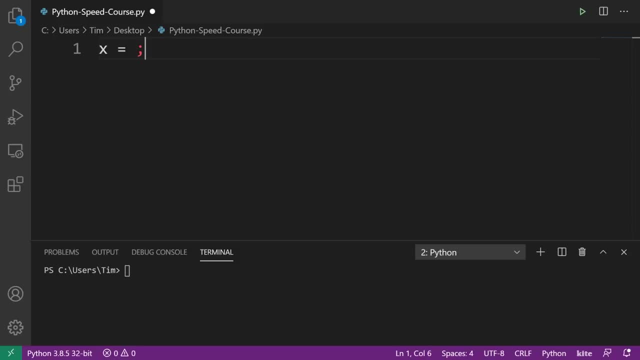 function. You don't define a Lambda using the deaf keyword. What you can do is something like: X equals Lambda X and then X plus five. What this means is this Lambda is going to take one argument, which is X, and then it's going. 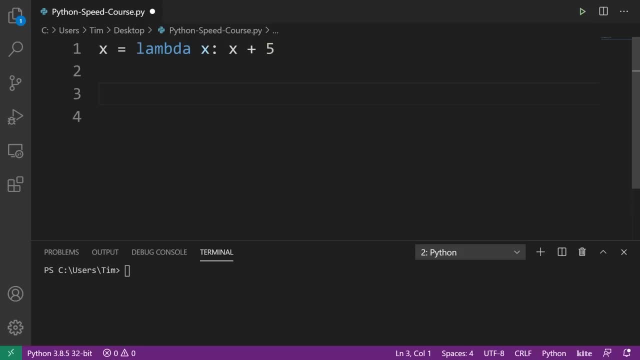 to return X plus five not multiplied by X Didn't mean to do that. That means if I call X like this and I go, I don't know X two and we print this, let's just go ahead and have a look at this here. 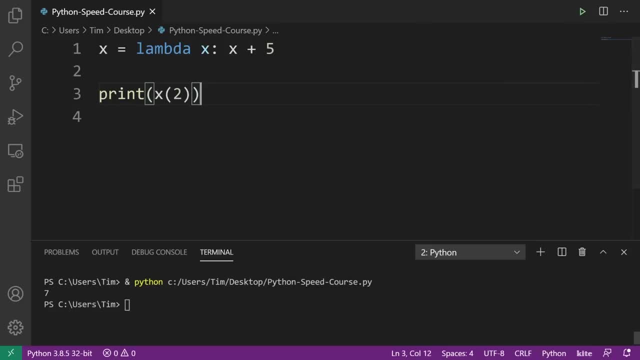 Oops, again, did not mean to do that. We see that we get the value seven. Now I will note that this is not the advised way to use a Lambda. We're going to see how to use it in just a second in the 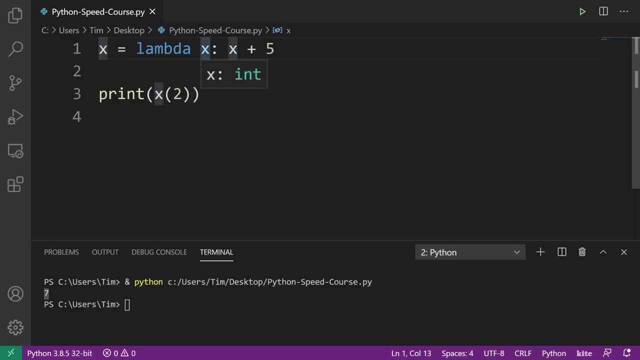 next section. This is the basics of how it works. It's just a one line anonymous function, So I can do something like X- Y as well, And then I can do something like X plus Y, not capital Y, And if I go, 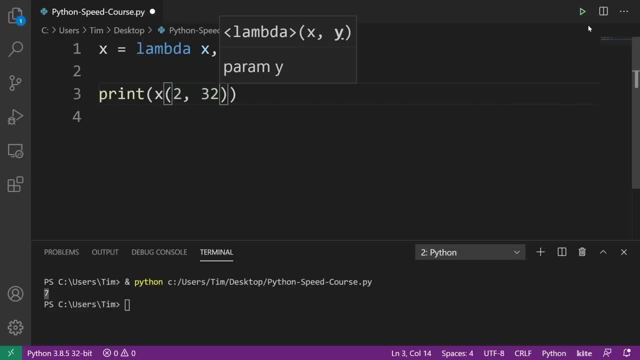 ahead and call X with I don't know two, three or two, 32.. Sure, That's fine, Let's have a look. here We get to the value 34.. So hopefully that makes sense on how the Lambda works. 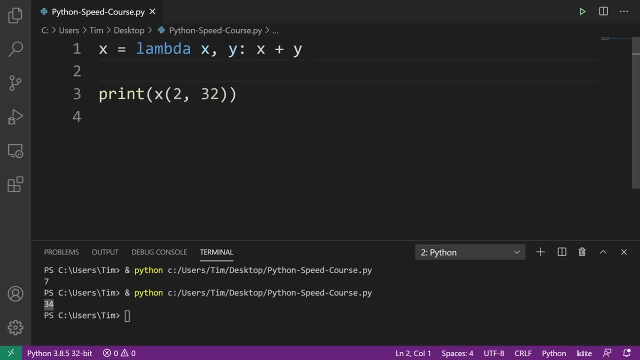 It looks intimidating, but it's really not that complicated, And in the next one you will see why these are useful. And now I'm going to talk to you about map and filter, which are two useful functions in Python which make use of the 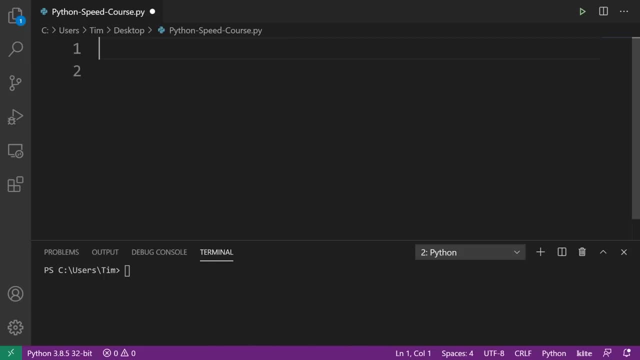 Lambda functions. Now, you don't necessarily need to use Lambda function, but a lot of times it comes in handy. So let me show you what I mean. Let's make a list, Let's add: oops, I wanted to do a. 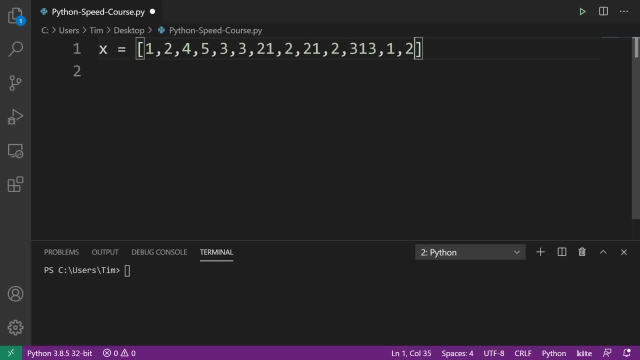 few more commas than that. Let's add a bunch of elements inside of here, Just make it kind of nice and long, So we get some interesting output. And now what I'm going to do is I'm simply going to show you how we use map. 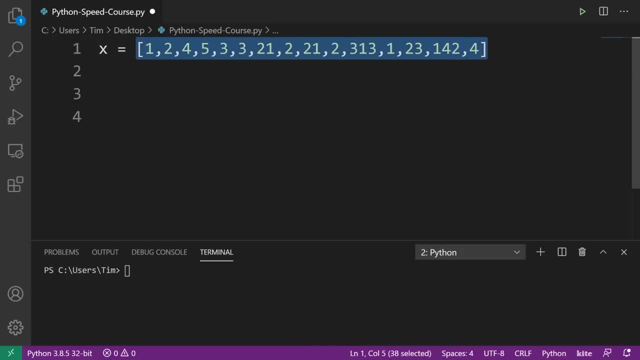 So what map will do is we'll take all of the elements of a list and use a function to map them into a new list. So if I say something like MP standing for you know map, I can say map, which is the. 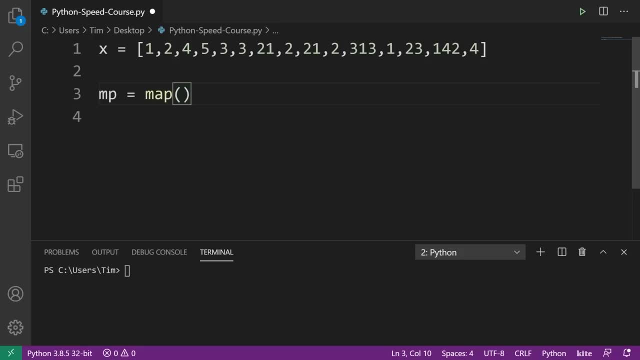 actual function. Now what I do is I put a function inside of here that I want to use for the map. So this will make sense in a second. but I'm gonna say Lambda X, X plus two. So this is essentially saying: add two to every. 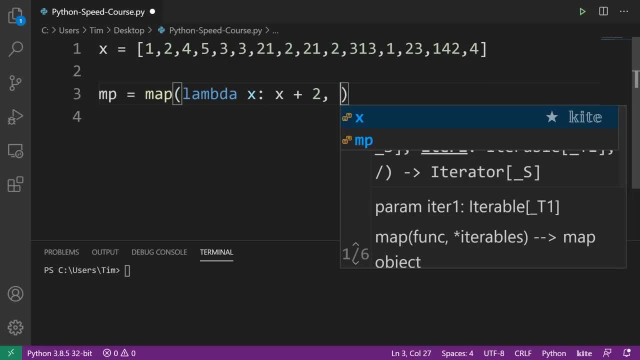 single one of these elements, or add two to X in this case, And then what I do is simply pass X. Now I know X is kind of confusing, So maybe we'll just change this to I so that it's easy To differentiate. But 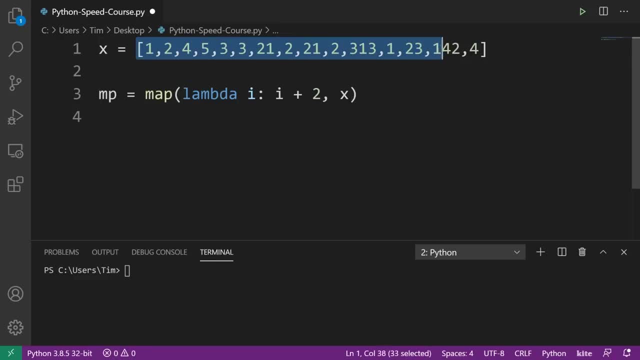 what this is going to do is say: okay, we're going to map all of the elements inside of X. So in this list, X to this Lambda function, which means take this Lambda function and apply it on every single element of X and then put that: 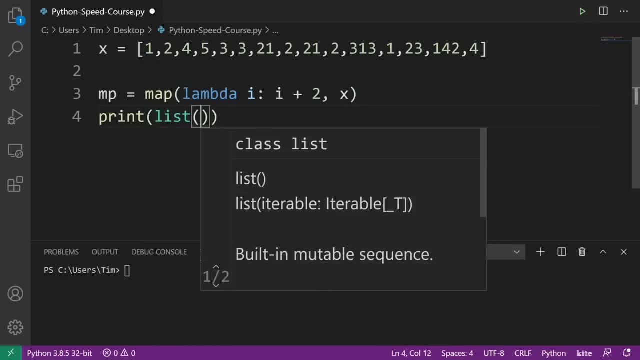 into a new list. Now what I'm going to do is I'm going to print the list. representation of MP map actually returns to us a map object. We can use that if we're going to iterate over it, but it's usually more. 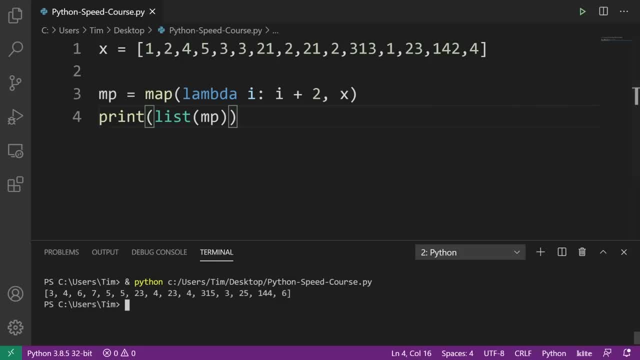 useful, just to convert it right into a list. So let's have a look at what this does. And there we go. Now we get three, four, six, and you can see all these elements have been added by two. Now we can do a more. 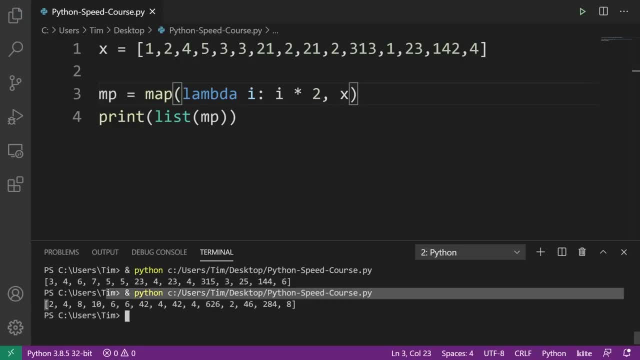 complicated one. Maybe we can multiply by two. You'll see more of a difference. And there we go Now. the next function I want to show you is filter. So hopefully you get the idea of how map works. but filter I don't want. 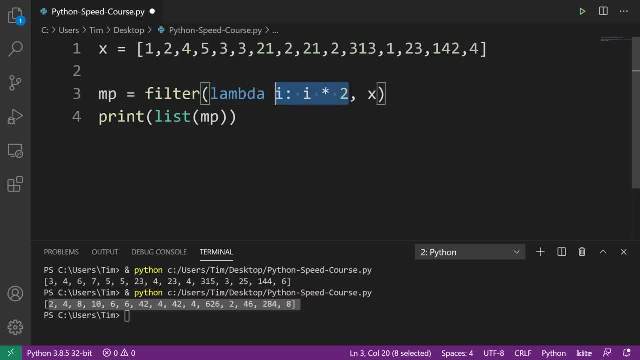 to say the opposite, but it does something a little bit different. So this function here, which is the Lambda, what it's going to do is, instead of actually returning some value, it's going to return true or false And it's going to tell us whether 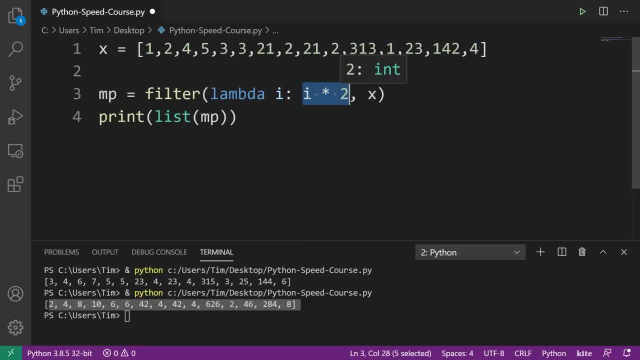 or not, we should include the item in our final filtered list or filtered object. So essentially, this Lambda function, or whatever function we put inside of here, has to return true or false based on the value of an item. So what I could do is say: 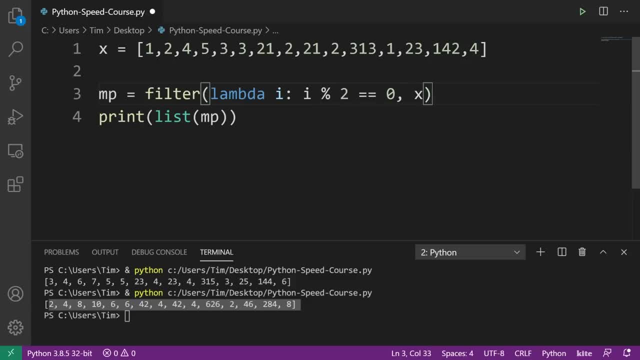 something like I is: I mod two equals equals zero, So this means, you know, only return it if it's even so. this is the function: take some value. I tells us if it's equal to our sorry- divisible by zero And 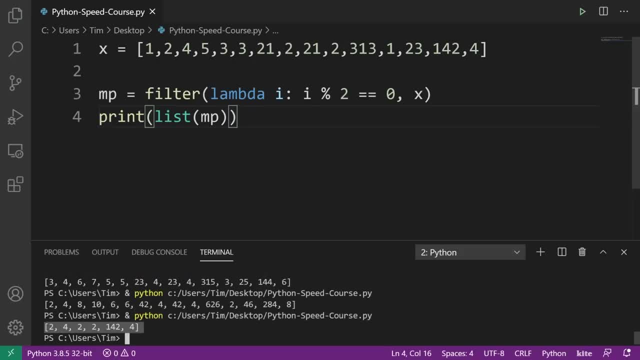 if it is, we'll include it. So let's have a look now And you can see that we only get all of the even elements in our list. Now, of course, what we can do is also define a more complicated function. 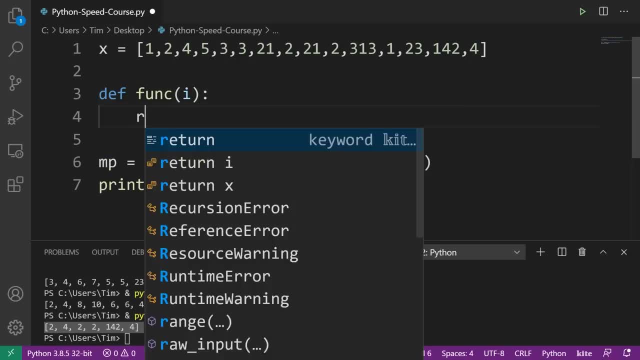 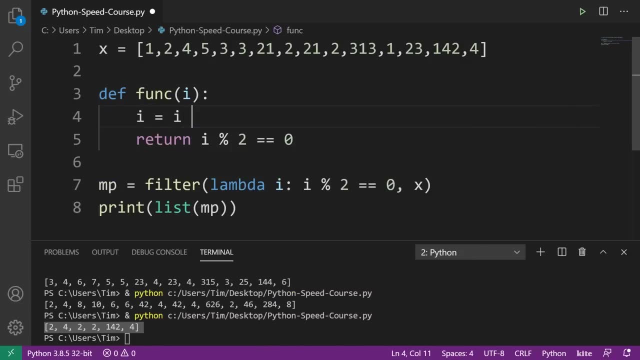 So we can say: define funk, take some value, Let's go with I. and we can do the same thing here. We could say: return: I mod two equals, equals zero. but we can also say: you know, I equals I multiplied by three. So 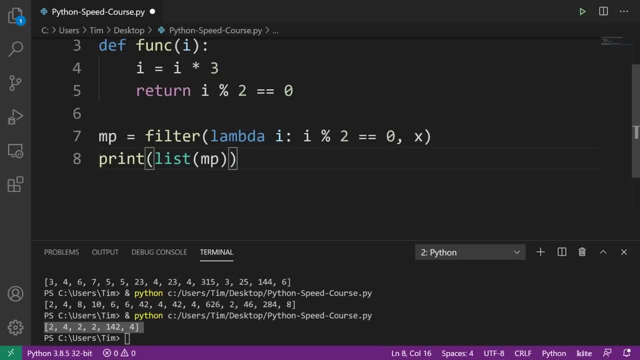 we can do that. And then we can say: I've mod two equals equals zero. Then, instead of using a Lambda here, we could simply just write funk. That's totally fine. So we just put the name of the function that we want to use. 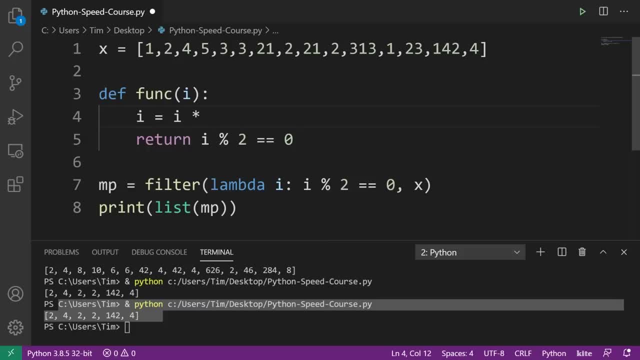 and then we run this and that works fine. But this is why Lambda is useful, because a lot of the times you don't want to define your own function up here, You just want to define it right inside of the map statement or the filter statement. So that's. 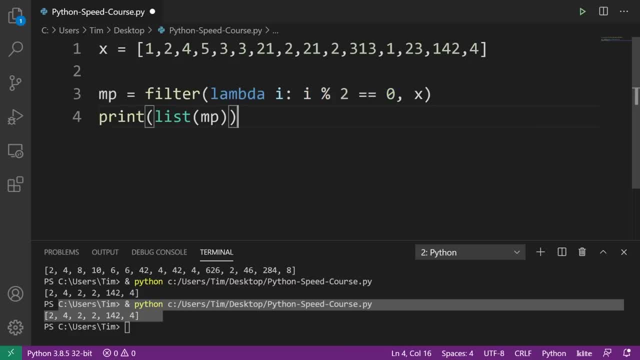 kind of where you would use this. There's no other. there's another few use cases for it, but this is kind of the most common and where you'll often see it. So, anyways, that is a map and filter. And for our last, 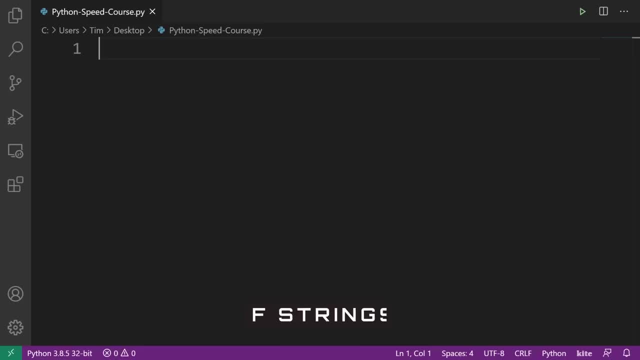 and final topic. I'm going to be covering something called F strings. Now F strings are new in Python 3.6.. If you have any version lower than that, you are not going to be able to use F strings, but they're a really cool. 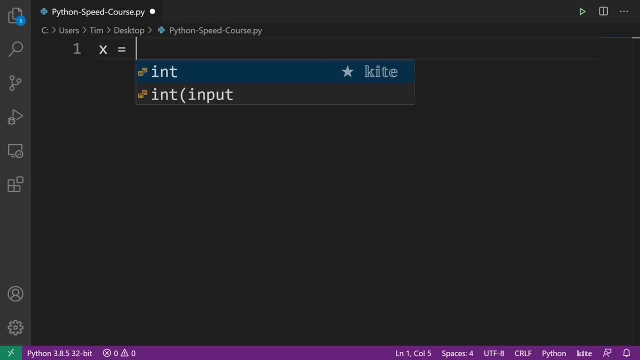 way to actually just manipulate and create strings. So what I can do is do something like X equals. I can do an, a lowercase F or a capital F, It doesn't matter- And then a string notice that this will highlight, or maybe it'll be a. 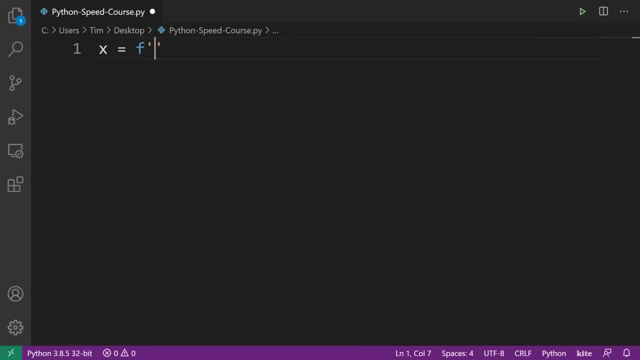 Talos, Depending on what editor you're using. and well, what you can do is type a string as you normally would, except now, if you want to embed an expression, what you can do is do that inside of curly brackets, So I can do a. 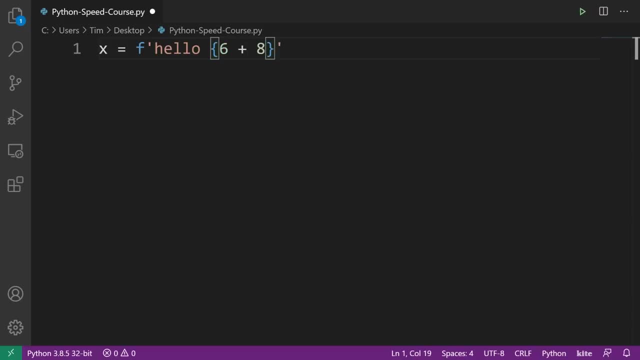 hello. And then I could say, like you know, six plus eight and this will actually be evaluated. And now, when I print this out, it will give me the answer 14.. So this is great, because if you have some variables, say 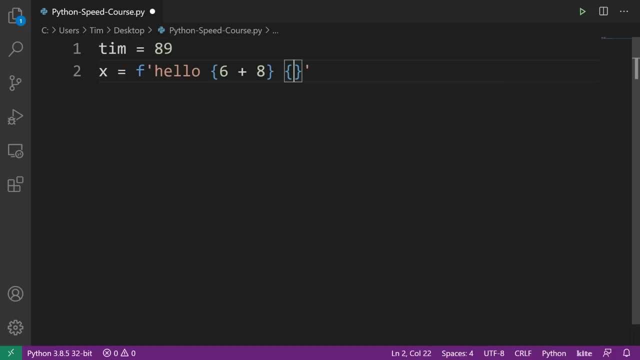 like I have. you know, I don't know, Tim equals 89 or something, And I want to embed that in the string without having to concatenate it and convert it into a string with STR. I can simply just use the F string and just. 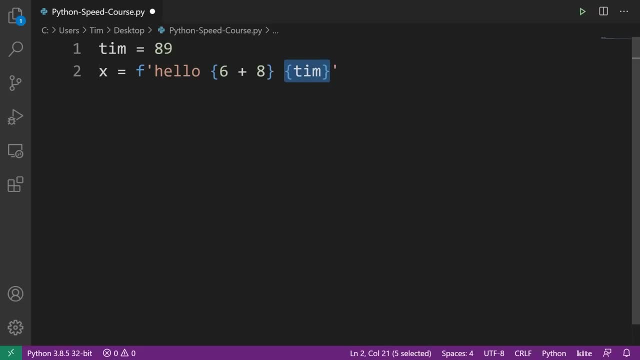 embed it with all the formatting uh, by putting it inside of these curly break uh braces. So that is kind of how that works. You can go ahead and mess around with this If you want to really see how it works. but 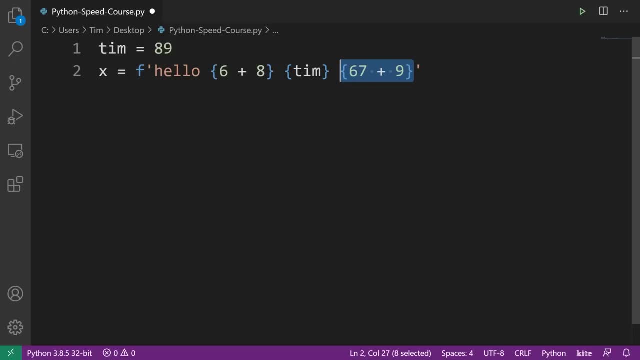 essentially, you just put an expression inside of these curly braces, it will be evaluated and then it will turn into a string. Really great, easy way to work with strings. Of course, you can print an F string as well. I could print hello, and then we can. 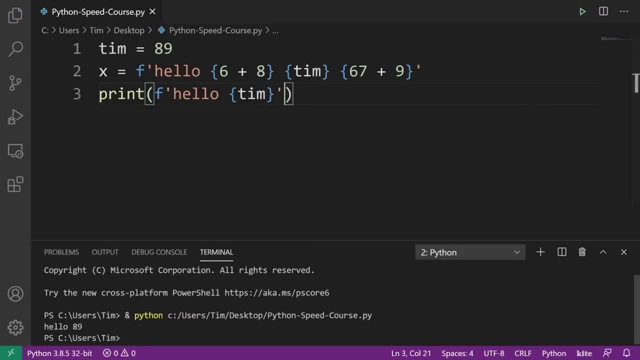 do that And, in fact, let's run this and just see what we get. And then we go, we see we get hello 89.. So that is F strings. So, with that being said, I'm going to conclude the video. 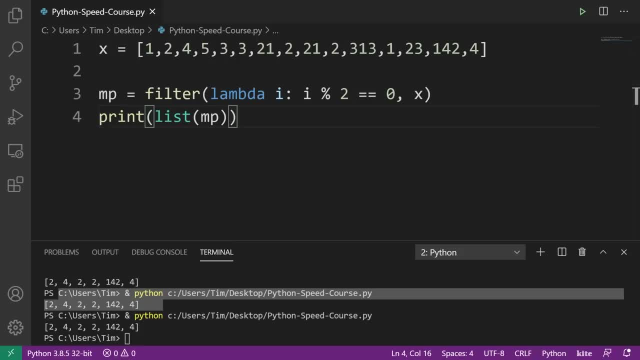 here I am officially out of breath. I went very fast through this tutorial with the purpose of making it as quick as possible and not wasting any of your time. If you guys appreciate this effort, please do leave a like, subscribe to the channel And, of course, 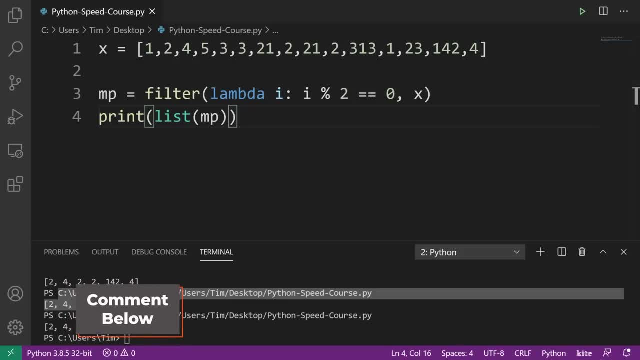 let me know what you want to see next. I will quickly mention that I did miss a few things in this video. uh, specifically, object oriented programming and advanced language features. If you would like to know about those two things, I have a ton of. 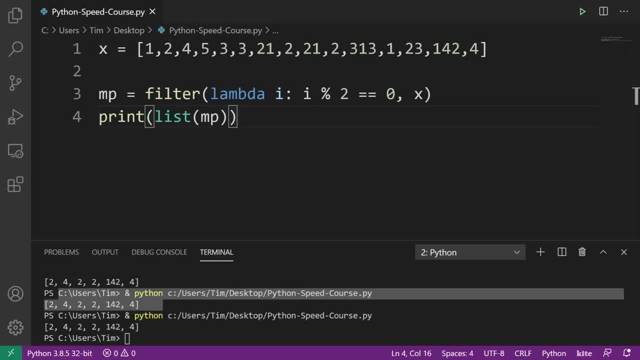 resources related to them. I will leave them in the description. The first is a bone an hour long video on object oriented programming in Python. that covers kind of all the fundamentals and everything you need to know. Then the next one is a whole series on 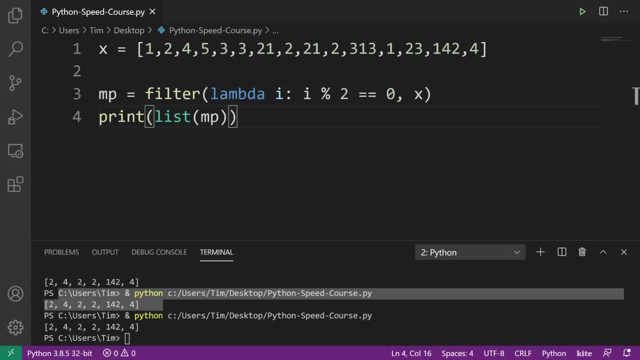 expert level features in Python. I believe. that's about six videos and covers things like meta classes, context managers, generators, all of that. Anyways, as I said, I hope you enjoy. leave a like, subscribe. I will see you in the next one.